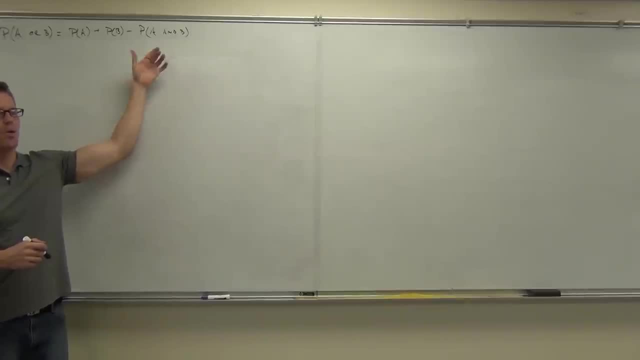 That's the double count. That's right. Or, in other words, this is the probability of event A and event B occurring in the same trial, The same trial. right there, That same is the key word. So this, right here, I'm making a clear point, because I'm going to do something that looks similar to this, And you have to know the difference between them, okay. So, right here, this means both at the same time. 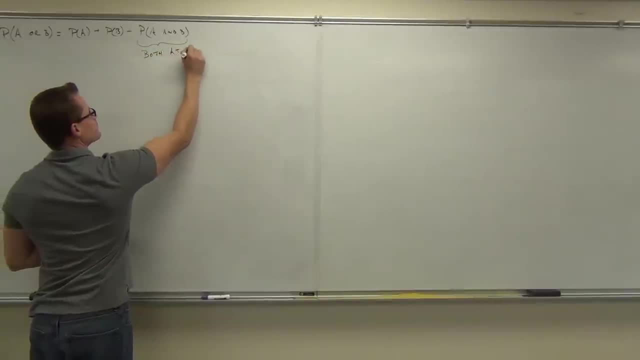 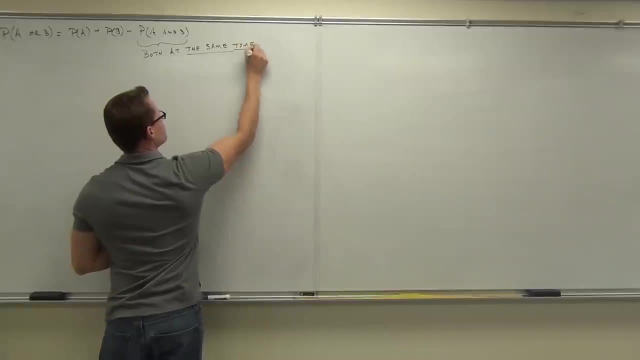 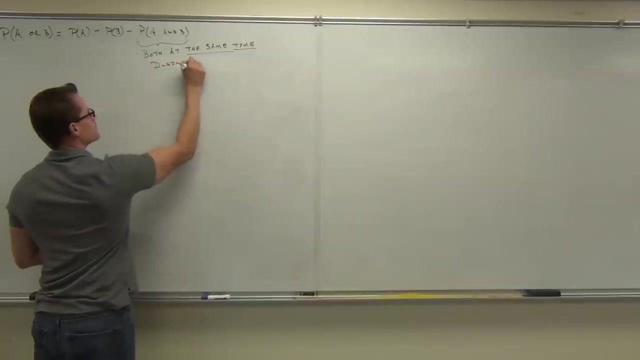 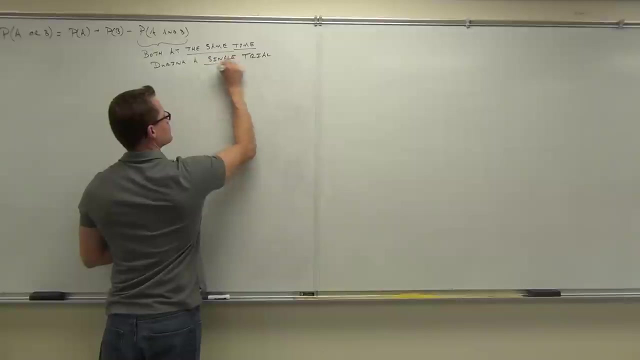 Or in other words, this is during a single trial, Both at the same time during a single trial. You see, right now we're going to get into section 4.4, and we're going to talk about something called the multiplication rule. 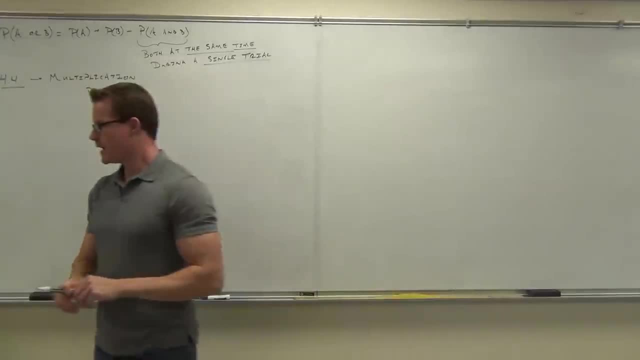 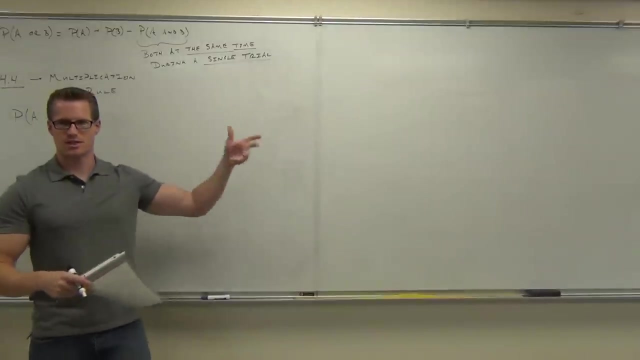 And we're going to have another word, and in just a bit- And I need you to know that there's a difference between the- and I'm going to tell you in a minute- and the and that we have from the addition rule. So here's why I made such a big stink about this, not literal stink, like a figurative stink. like you know, I didn't make a stink. 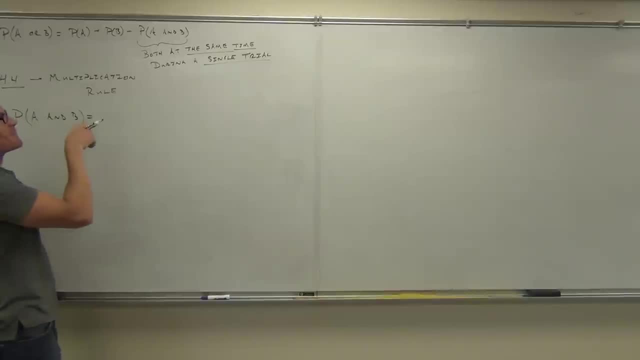 That came out weird too. So we have this: and, which means at the same time, in one trial This and for a multiplication rule. this means something different, And people get very confused about this Because in English we use and and and right. 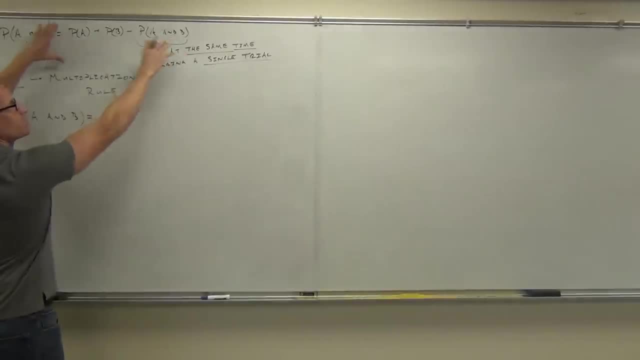 And we count this word twice Here. when we're talking about the addition rule and we're saying probability of A or B, what we mean is the probability of A happening or B happening, or they both happen at the same time. Nudge your head with me if you're with that. 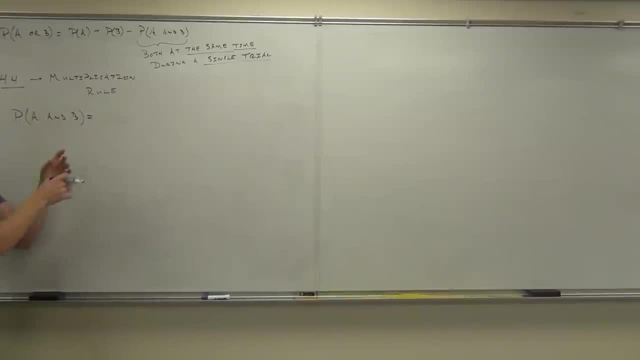 Okay With the multiplication rule, the probability of A and B. what we mean in this instance. if you just say, see probability of A and B, it's not in here, or anything. What this means is I want you to find the probability of event A happening. 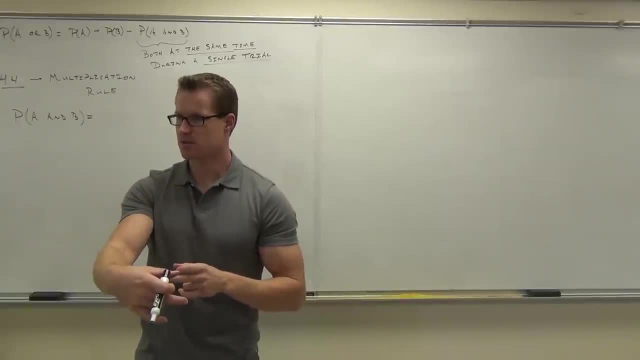 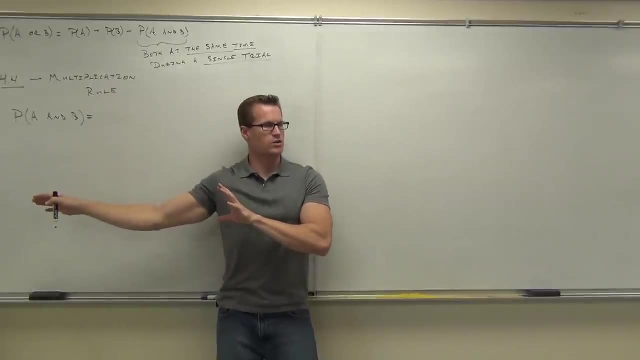 And Then event B happening right after it. Does that make sense? Two different things. This is A and B at the same time. This, right here, when we're talking about multiplication rule, says: I want you to find the probability of A happening and then, after that, B happening. 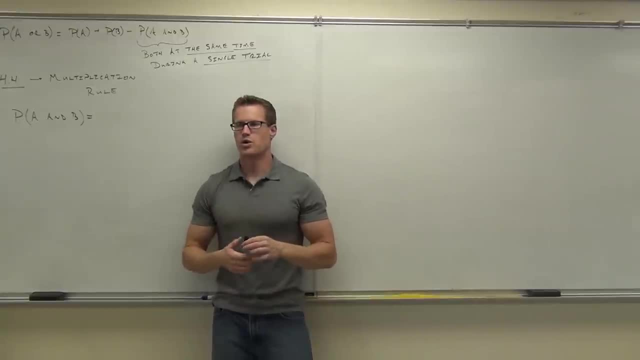 So, for instance, what's the probability that you take a dice out and you roll a five and then a three? Is that possible to do? Can you take a dice and then roll a five and then pick it up and then roll a three? 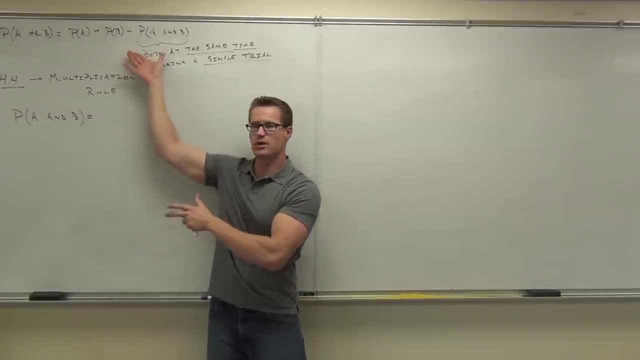 That's what we're finding the probability of here. In this case it was: what's the probability of rolling a five or a three? If you do one roll, they can't happen at the same time. But if you do successive rolls, you can roll a five, then pick up the die and then roll a three. 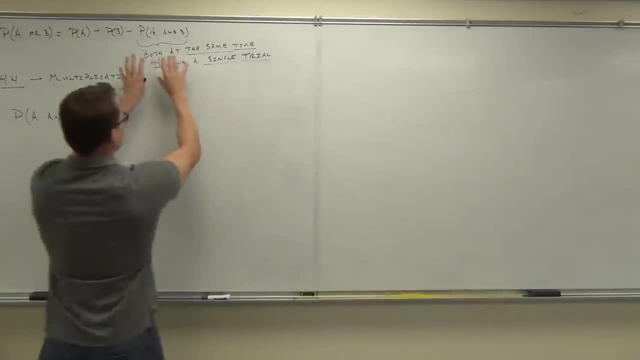 Do you see the difference in these two things? So, while this and meant both at the same time during a single trial, when you're talking about A or B, this and means the probability of A happening and then B happening in successive trials. So while this and meant both at the same time during a single trial, when you're talking about A or B, this and means the probability of A happening and then B happening in successive trials. Why I talk so long? my pen went dry. 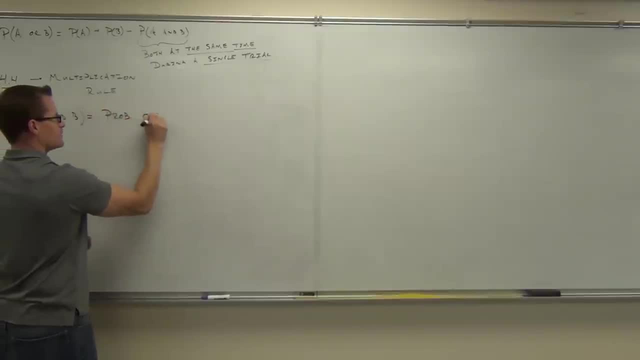 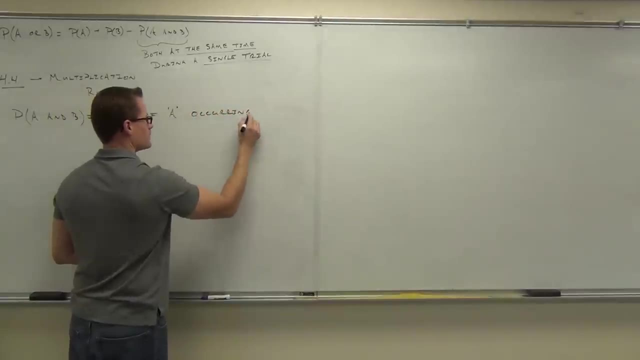 That's weird. The key phrase is: and then Not and at the same time, And then B occurring. The key phrase is: and then Not and at the same time, And then B occurring, And then B occurring In successive events or, I'm sorry, in successive trials. 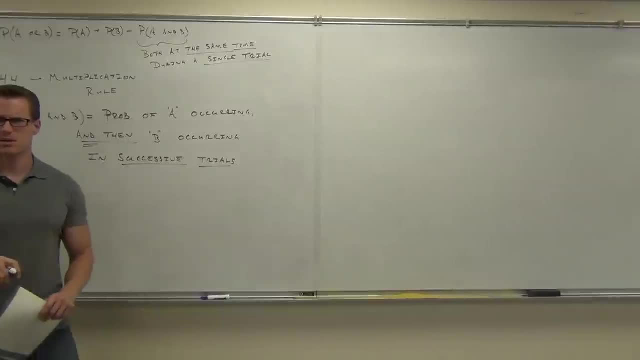 That word's successive. what's that mean, by the way? So right after, that's right. so right after each other. Would you raise your hand if you feel comfortable with the difference between the ands? So while we have two ands, they mean two different things. 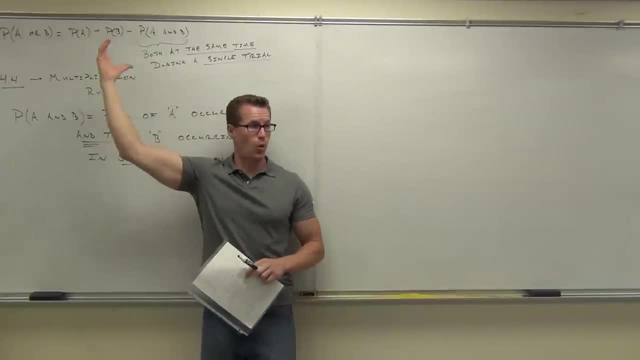 Same word, two different things. When you're talking about the context of an or problem, the and means. at the same time, When you're talking about the context of an and problem, that's multiplication rule. those trials are one right after another. 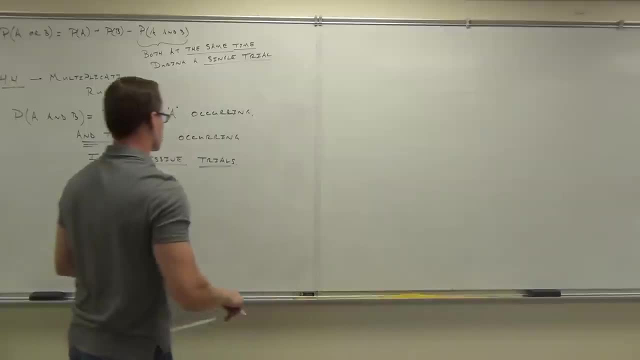 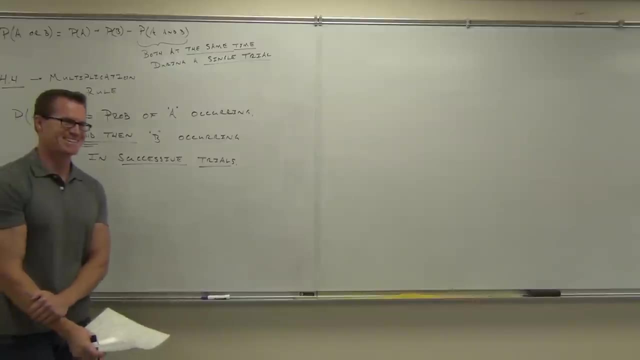 It's A and then B To kind of illustrate the multiplication rule. let's look at the multiplication rule. Let's say I give you a test, Ready for a test. Is it going to be a fun test? We just had one. 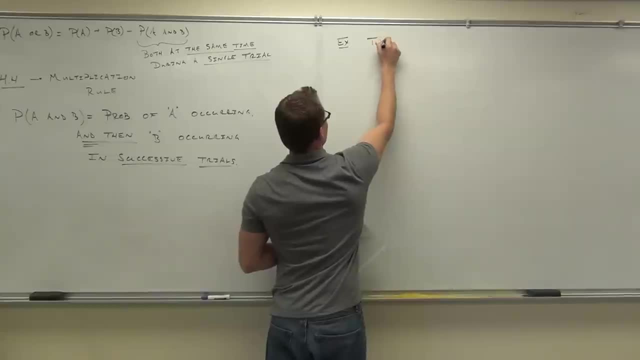 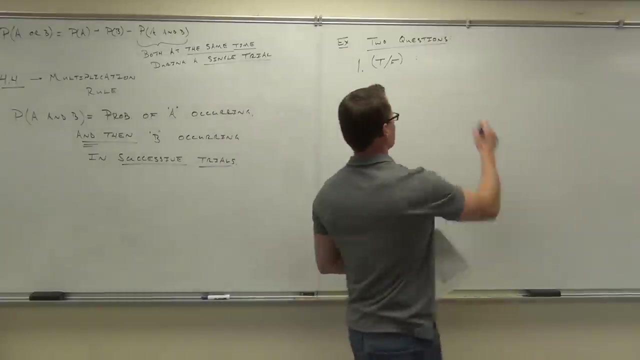 I'm a tough teacher, guys. There's only two questions on this test. Only two questions on this test. Question number one is a true or false question, And the question is: what is the answer to this question? And the question is: true or false. this or that drives an Audi. 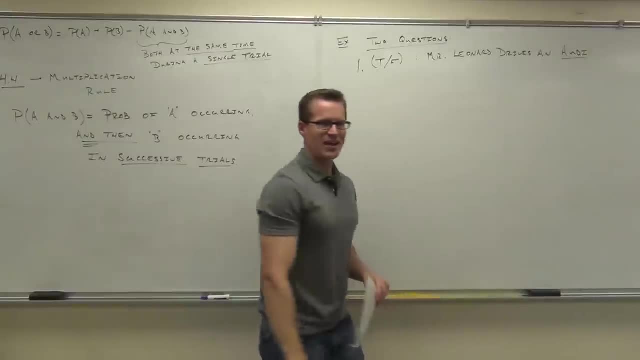 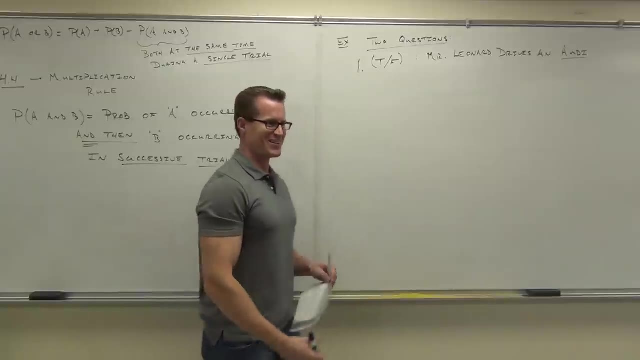 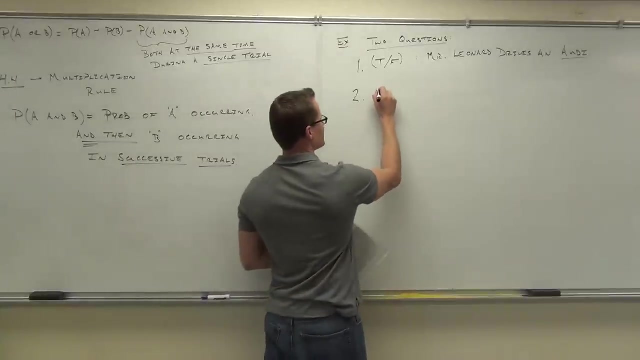 Ooh fancy. Does anyone know the answer to that question? All All right, stalkers, Whatever. How do you know? Oh my goodness. The next question is multiple choice. Someone in my other class asked Mr Leonard. 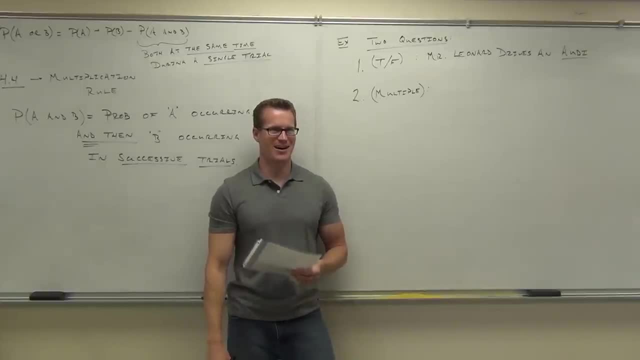 were you following me on the freeway, And I naturally my response was: well, I have no idea, It's not like that. I follow you around. And they said: oh well, do you drive a Prius? I was like: well, no, I don't drive a Prius. 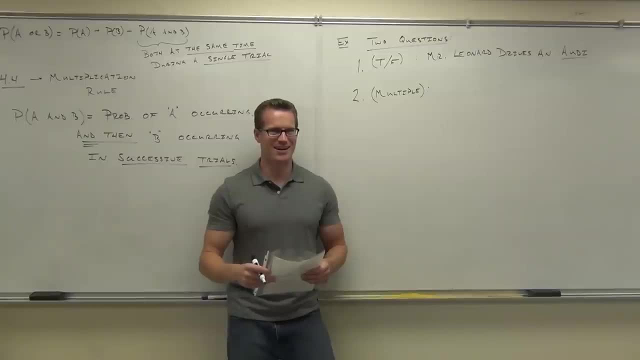 I said: wait, do I look like I drive a Prius? And the whole class was like, yeah, Okay, Did I look in the right direction? Looked in the mirror, Yeah, I look like I drive a Prius. 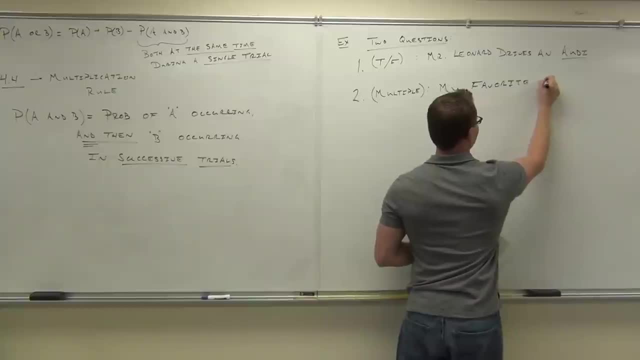 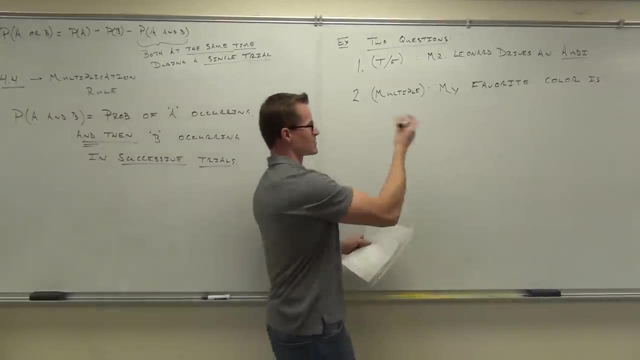 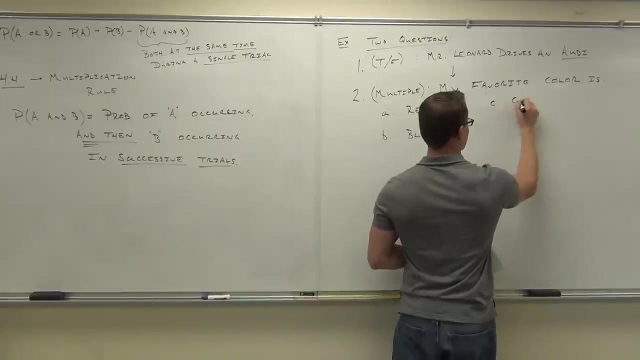 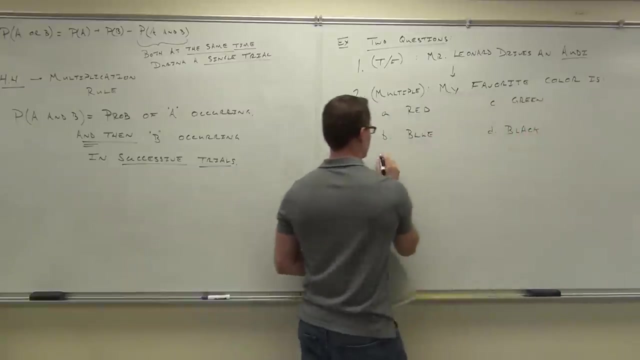 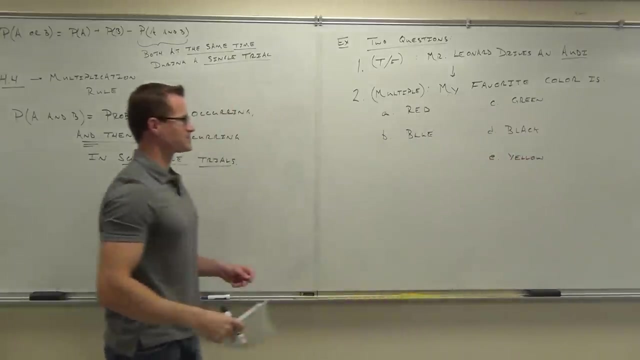 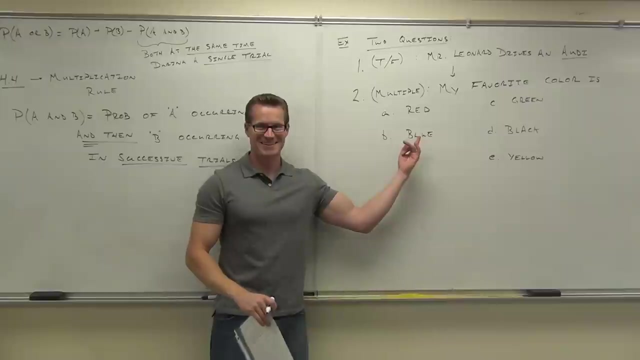 I don't, And my favorite color is: this is Mr Leonard's favorite color. Let's see, You have a choice. We did it All right. All right, Okay, I see how much you like it. Does anyone know the answer to this question? 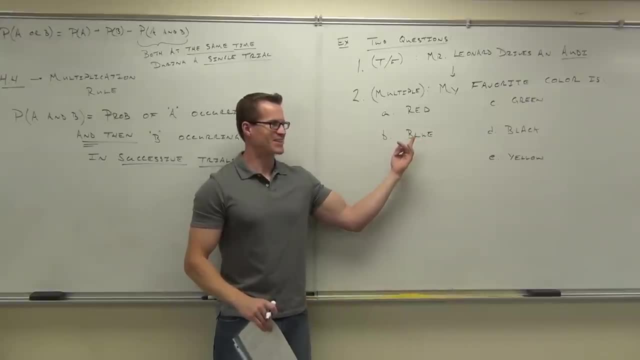 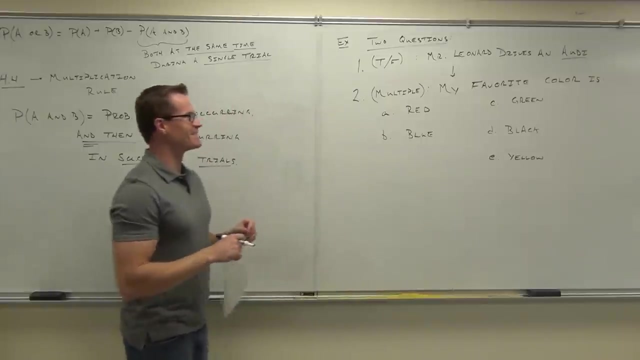 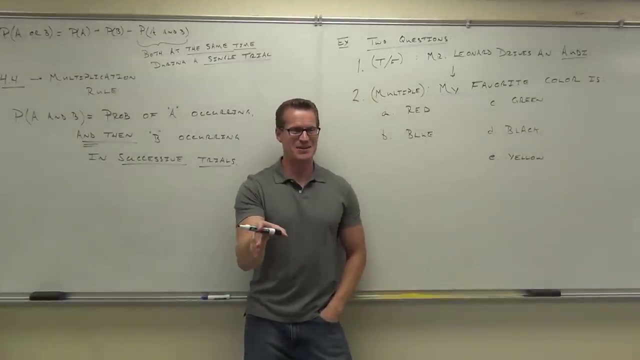 Let's pretend that Adriana doesn't know the answer to this question. Let's pretend you didn't know the answer to this question. I just made these up randomly. Let's say that you didn't know whether or not I drew an oddy. 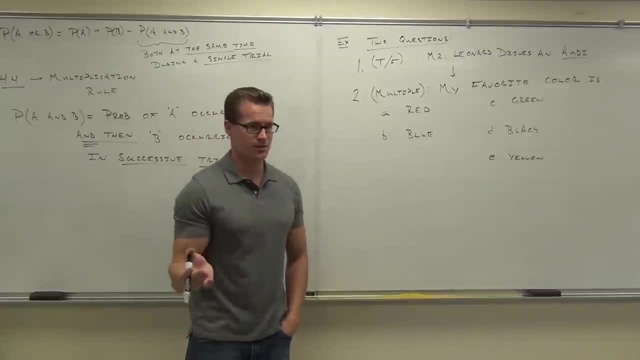 and you didn't know what my favorite color is and you are going to take a random guess at this. What I want to know is, if you guess randomly, what's your probability that you are going to find the right answer? We are going to discover that. 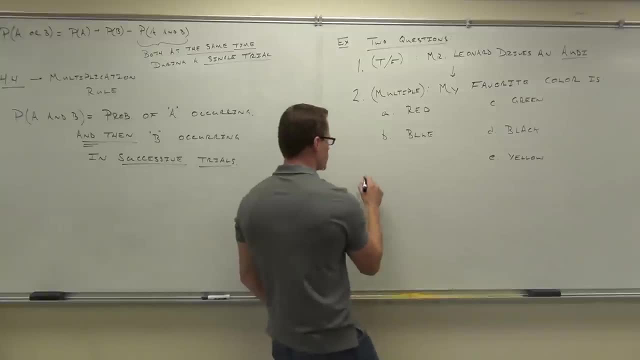 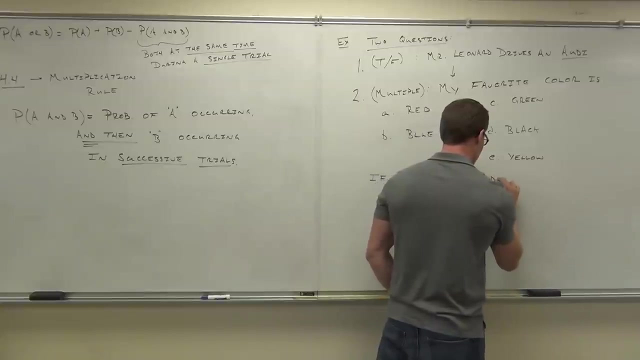 and we are going to start with an easy example that will lead us into the multiplication rule. If you guess randomly- which most of you are going to have to do because you don't really know anything about me- thankfully, If you guess randomly, what's the probability you will get the right answer on both questions. 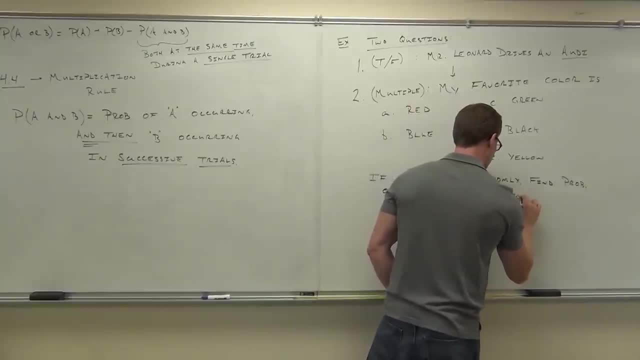 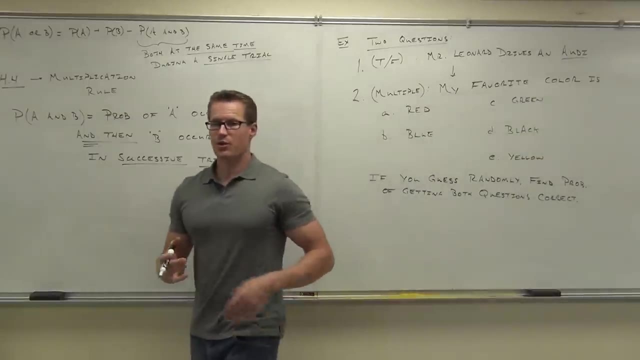 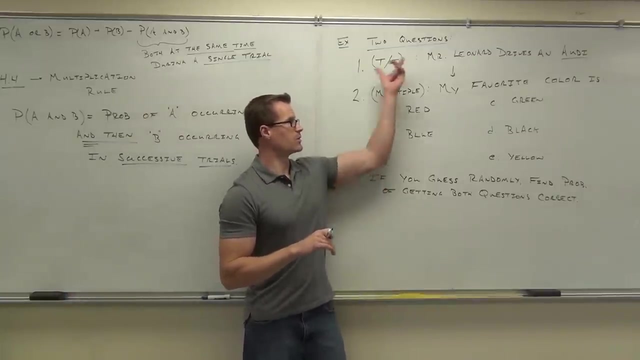 Now I want you to notice that we are not in the addition rule any longer. I'm not asking what's the probability of you getting either this one right or this one wrong. I'm not asking that This one right or wrong. 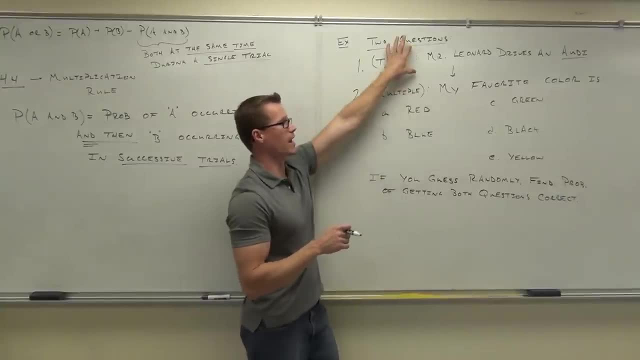 I'm not asking that. What I'm asking is: find the probability that you're going to get this one right and then you're going to answer this one too right. Find the probability that you're going to get this one right and then you're going to. 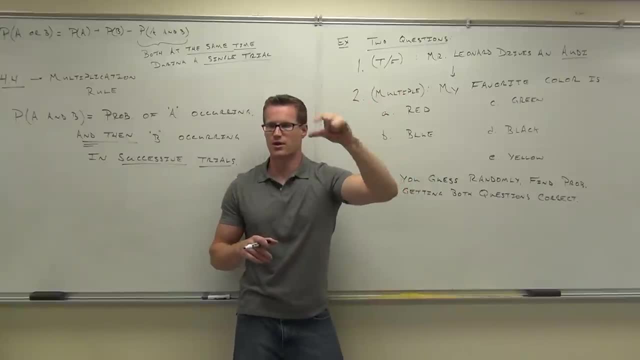 get this one right. Notice how we're talking about successive events, one right after another. An event would be answering the question, So you're going to answer this one, then you're going to answer another question. That's this one That, right there, tells you that we are in an and type of probability. 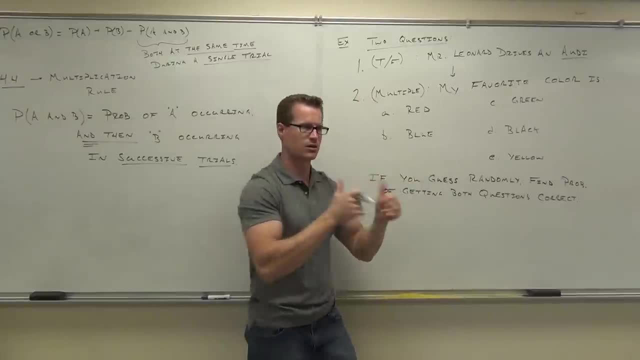 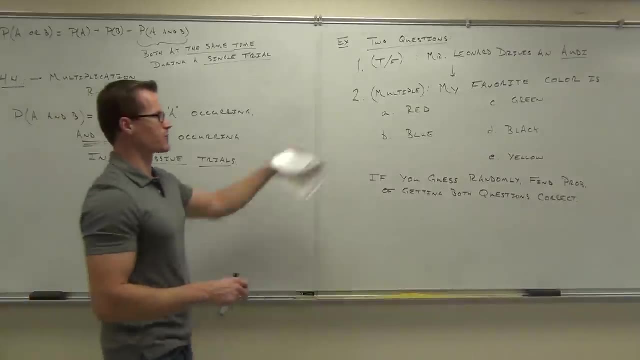 We want the first one right and the second one right Now. are you going to be clear on that? Good, All right. What needs to happen for us to get both answers right? Well, you've got to answer the first one right and then you've got to answer the second one. 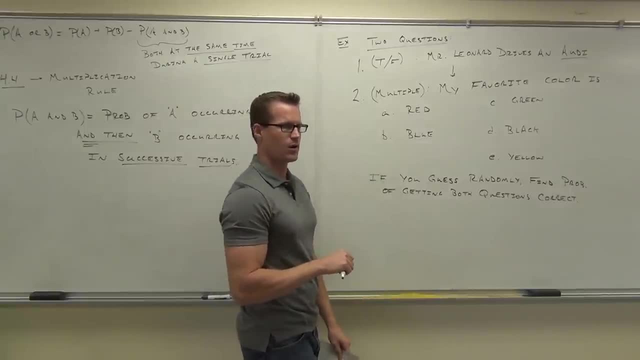 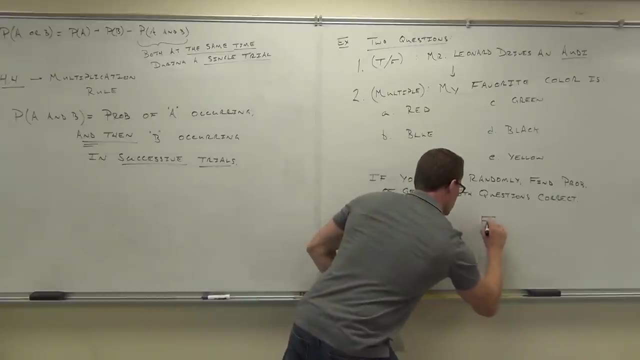 right. How many choices do we have? How many choices do we have to choose from? How many choices do you have? for the first one, Two, Yeah, because you could do either true or false. You could do either true or false. 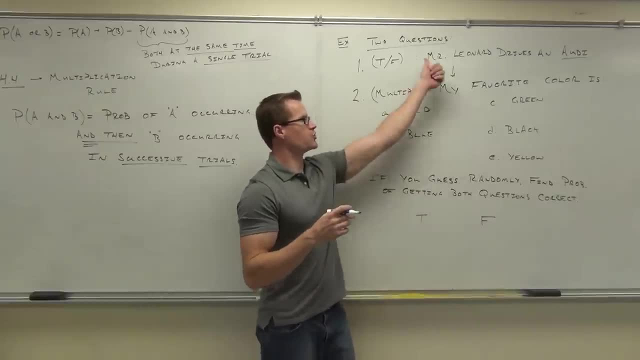 Now, if you pick true, does it determine what you're going to pick for this answer? So you could pick true and then pick A, couldn't you? Or true, and then B True and then C True and then D True and then E. 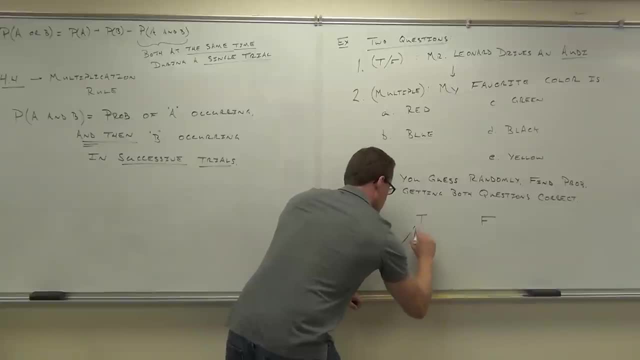 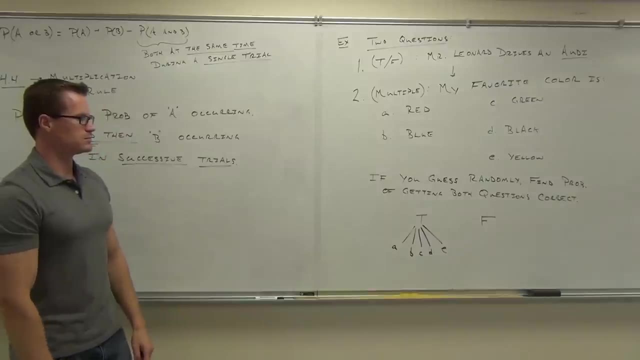 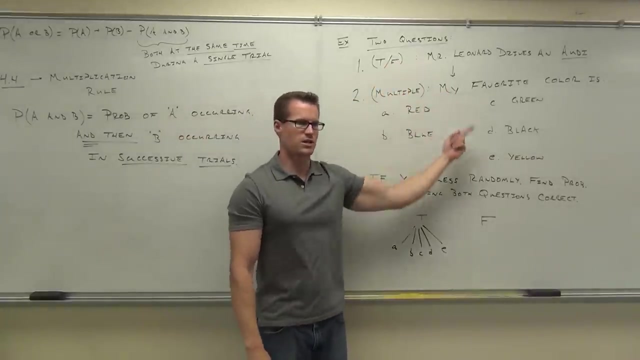 Now it gives you for each T, A, B, C, D and E to choose from. Now what if you choose false? Could you choose false and then choose A, False B, false C? It gives you the same five choices for choosing false as well. 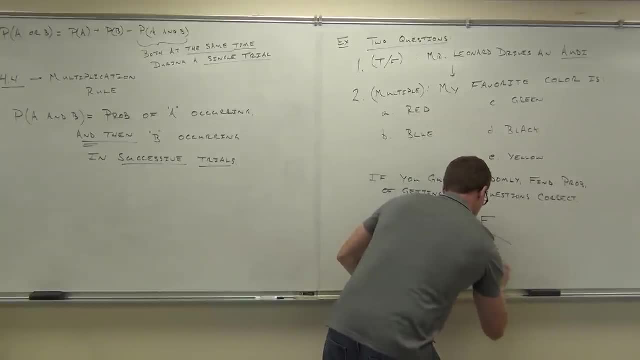 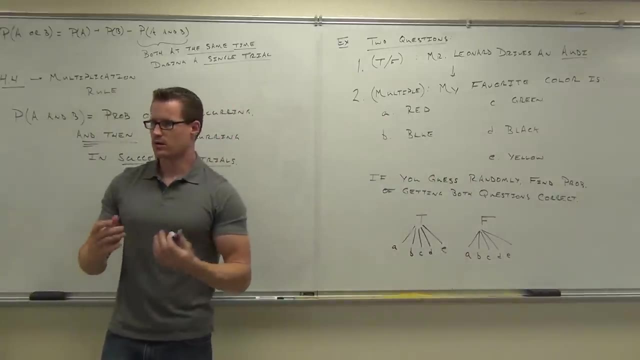 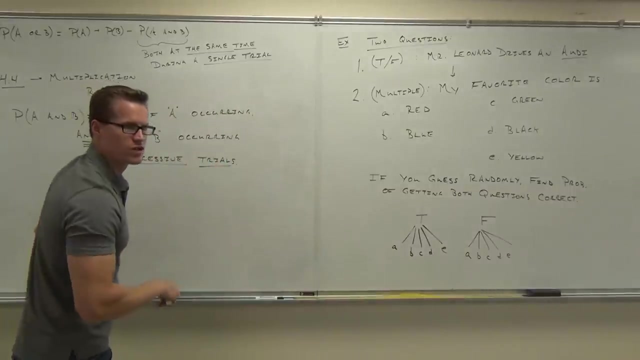 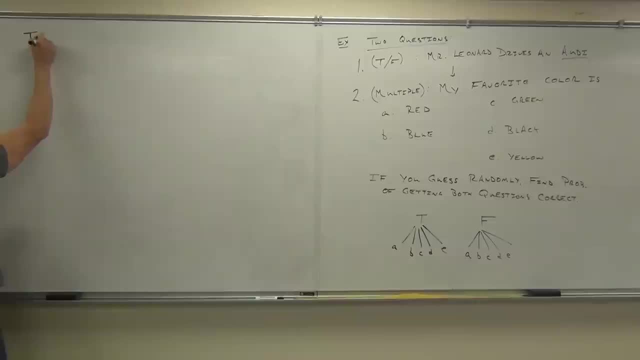 Let's talk about our sample space for our choices here. Remember, sample space is everything that you can happen from your procedure If our procedure is answering these two questions randomly, one right after the other. I'm just going to list it out because I wanted to kind of go over sample space again. 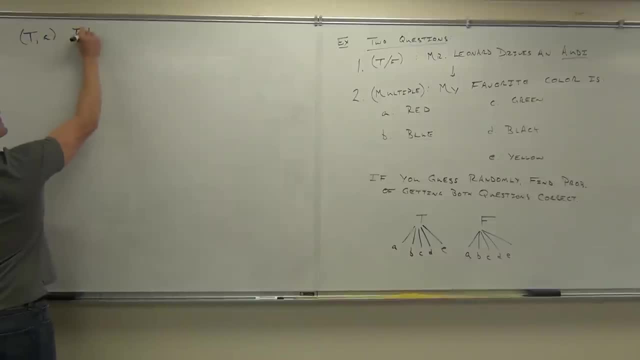 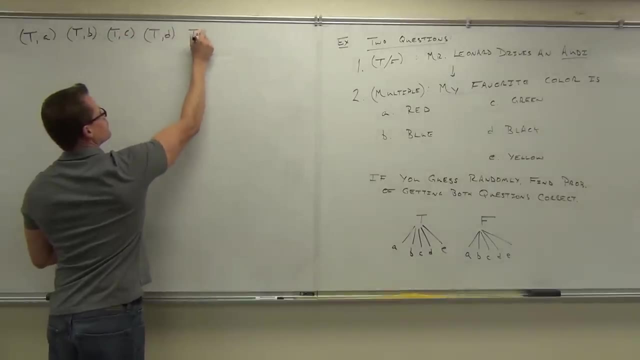 Our sample space is true, and then A- that's one that we could get, We could get true, and then B, that's another one True, and then A True, and then B, B, true and see and so forth. would you agree that this is everything that? 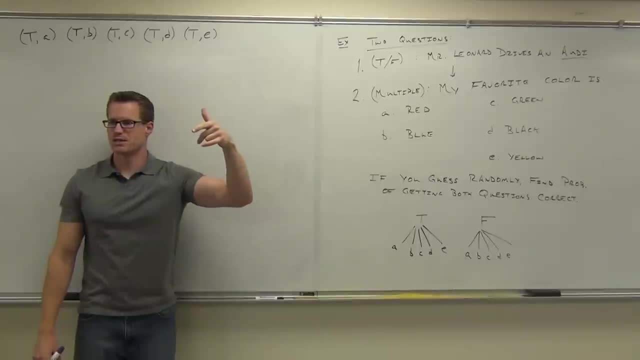 starts with the T. notice how we're kind of going on the same idea, as are the boy, girl thing that we did the three boys, two boys, one girl. here's all our true, true comma, multiple choice answers, and our false ones look almost identical is just, instead of the T's, like that. 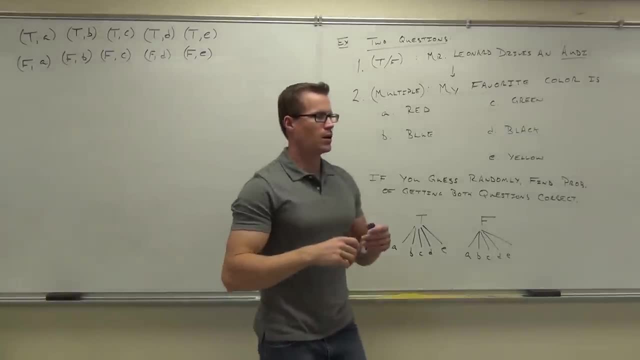 okay, here's the question: how many right answers are there up there? how many correct answers this going to answer correctly? one minute, two, three, four, five, six, seven, eight, nine, ten, ten, twenty-two, twenty-two right. I don't have more than one favorite color. this can only be answered. 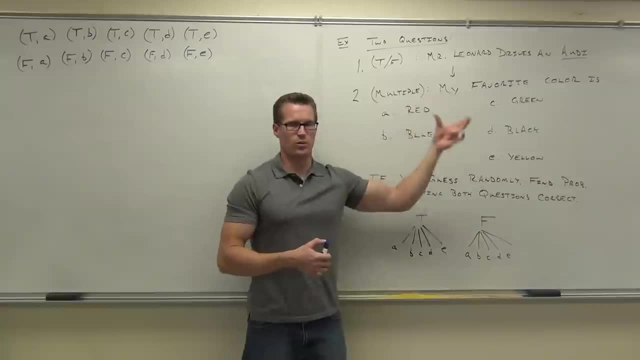 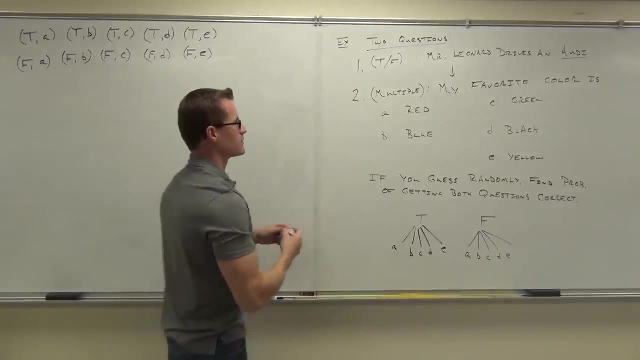 one right, one way as well. so together, there's only one way you can answer this correctly. one of these choices is correct. in fact it's- uh, it's this one. that's the correct answer, right there. so that's the correct answer. how many total choices do you have? you didn't know that, did you? you all thought it's an old body. 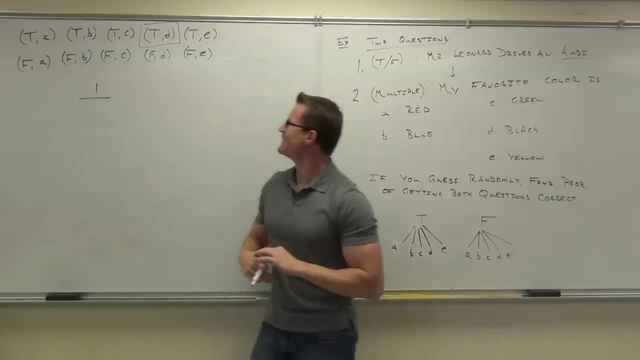 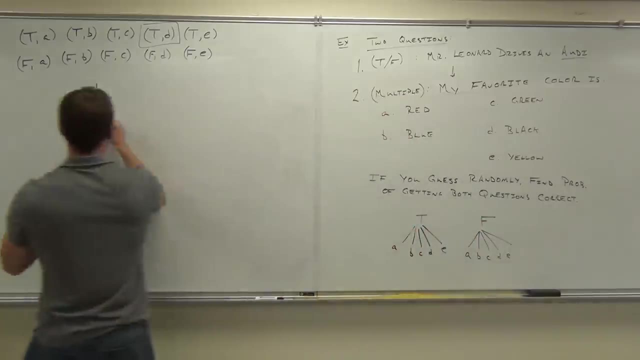 but so how many total choices did you have to choose from? there's ten ways you can answer the question. only one of them is right. so that's of one and ten chance you're going to get both of these things correct. so the probability of getting both right is the probability that you're going to randomly select true and 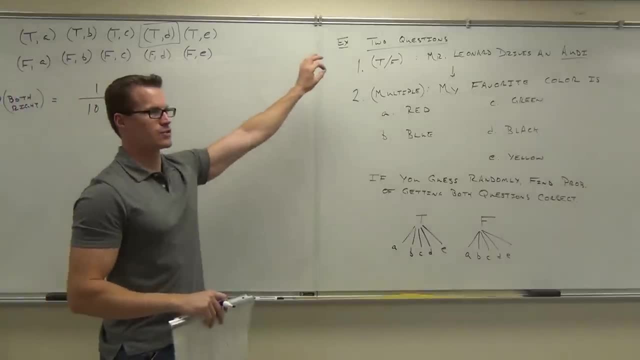 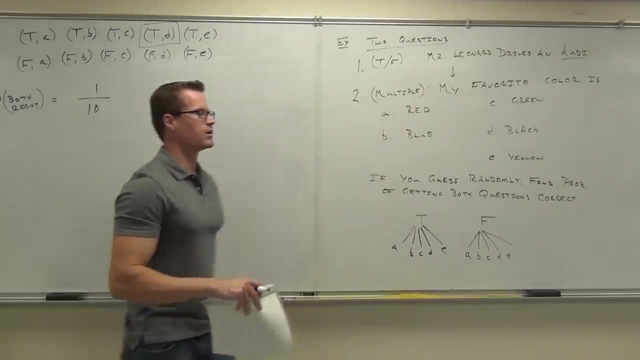 that you're going to randomly select D. that's half a chance. hope we not have a chance. you have a chance: 50% chance for the top one and a 20% chance for the bottom one. is there a way that we can kind of come up with a better way to do? 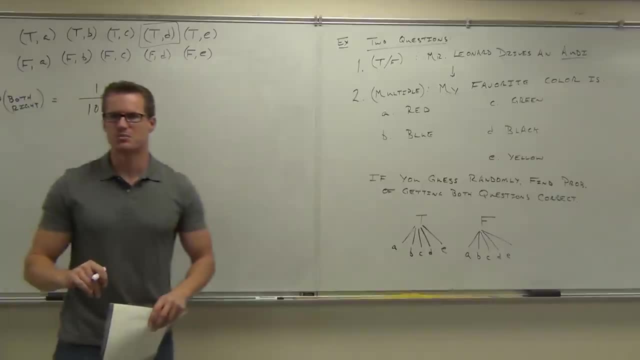 this and just sit, listen out. sample space answers. yeah, we're going to cover to just a bit. before we do that, I want to give you one more example, though the other example is going to go back to your guilty, not guilty table. see me remember the numbers from those. pretty sure this is 11, this one was nine. 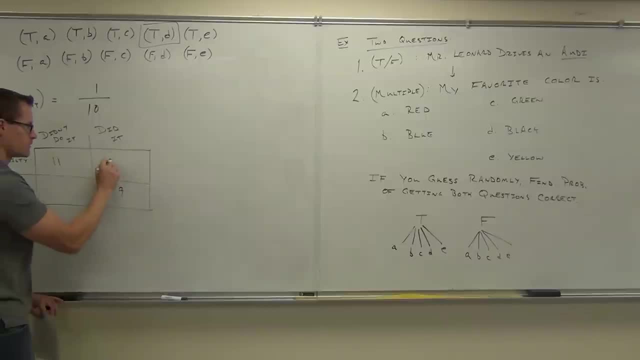 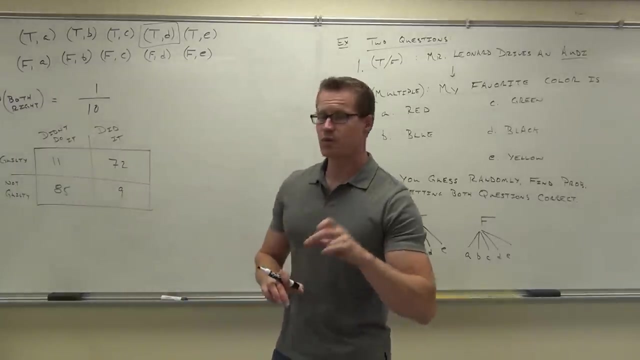 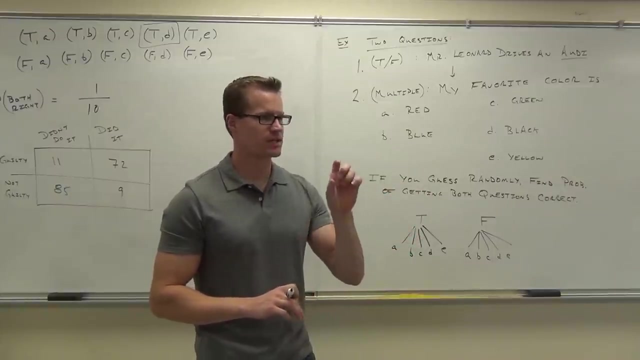 so we do sweet. I was easy. here's what I'd like to do. I want to find the probability of selecting someone who is guilty and then selecting someone who is not guilty. so I want to find the probability selecting someone guilty and then without replacement. that means I don't put that person back in the in the mix, almost like someone who's. 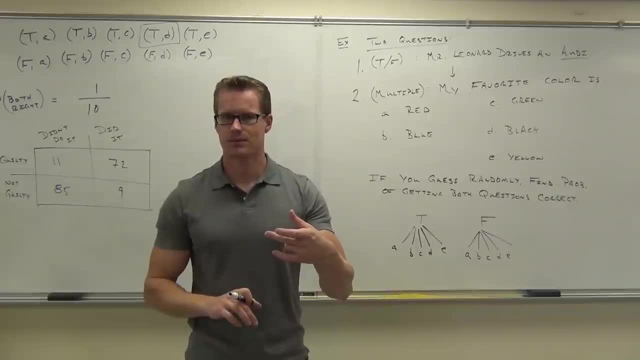 not guilty. so how many people am i selecting? how many people I'm selecting one person who is guilty and then selecting another person who's not guilty. how many people in total? two people notice how we have two trials now one trial is happening and then another one's happening. so the probability 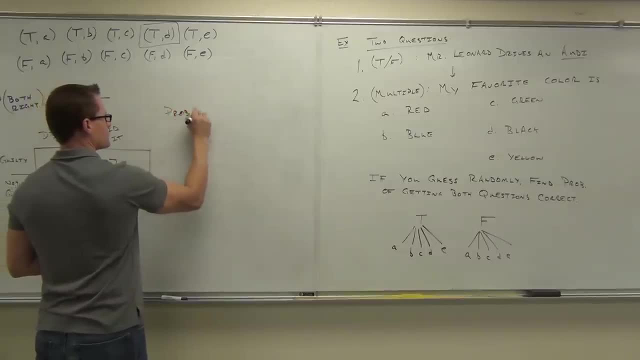 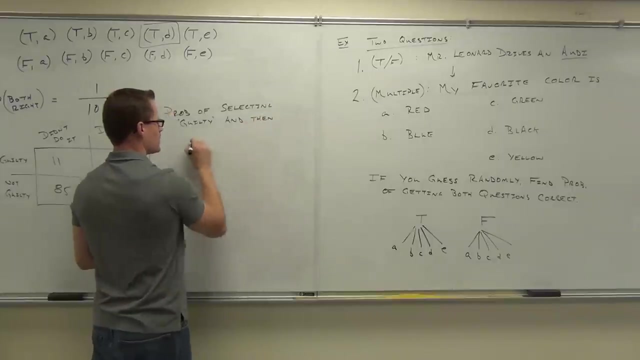 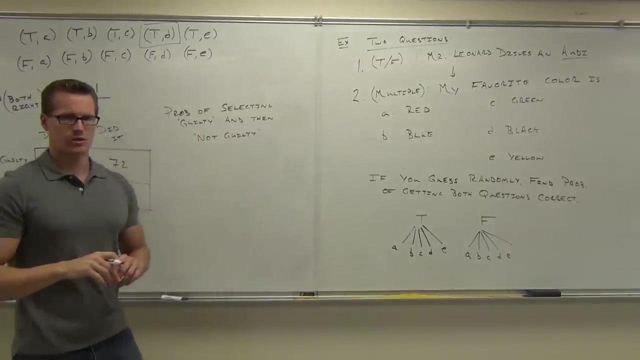 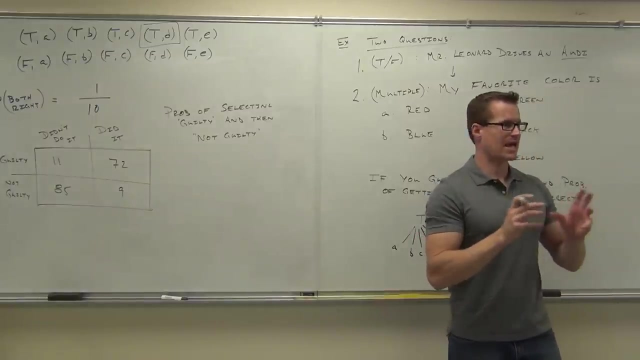 of selecting guilty and then not guilty. that and in the multiplication rule that we just talked about, that said this and means in successive trials that really should be written and then a and then so if you want to put a little and then that would separate them for you, that's. 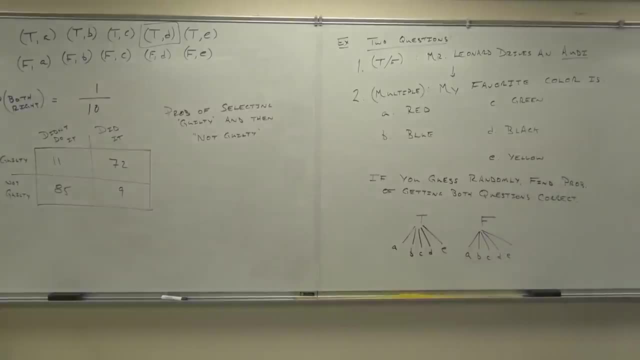 what we really need is the and then, so finally probably selecting guilty and then not guilty. let's talk about the guilty: you. what's the probability you're going to be found guilty in this group of people? how many guilty people do we have? how many people were found guilty? it's not. 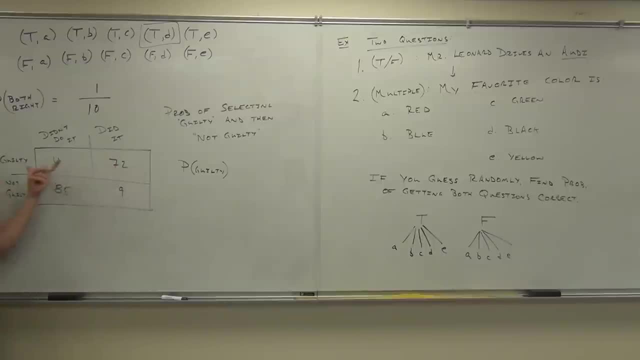 just 72. right, it's not just 11. this is my guilty column or my guilty row. I have 83 people. 83 people were found guilty. out of how many? how many guilty people were found guilty? out of how many guilty people were found guilty? out of how many. 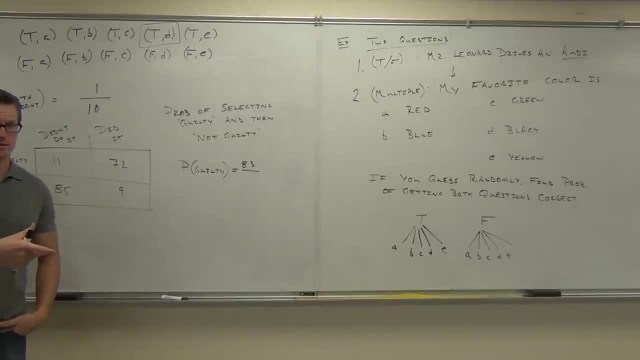 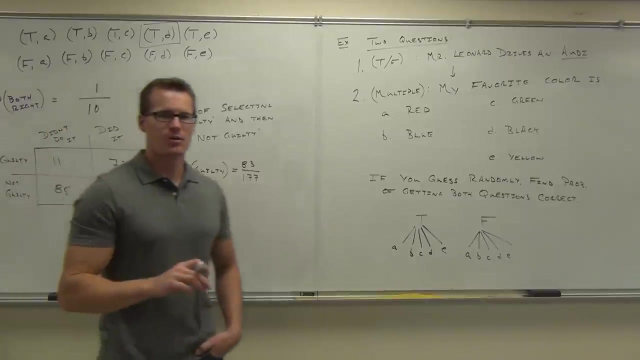 okay. how would you find out how many? add them all up? how much was it? oh, I'll, oh I'll, to get all four. all four is everybody 177, I'll believe you. Are you okay that the probability of being found guilty is 83 out of 177?? 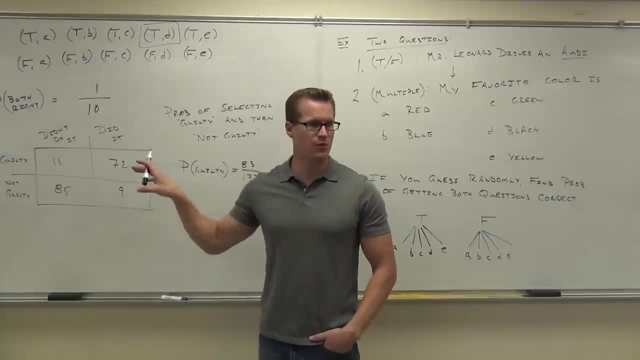 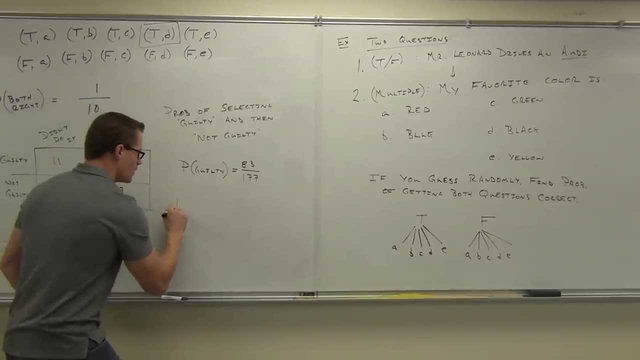 There's 177 total people in this. 83 of them were found guilty. True, Now here's the idea. This is the big part of this in the last few minutes here And then implies this: This is the key point. 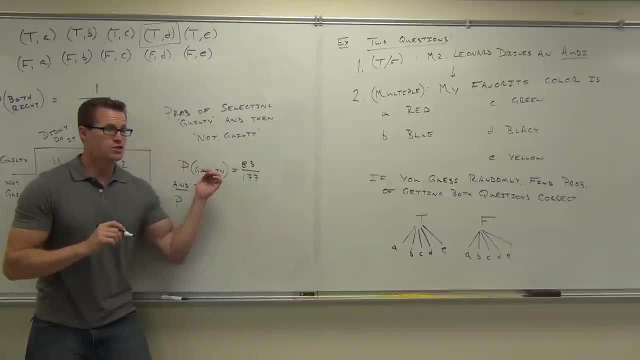 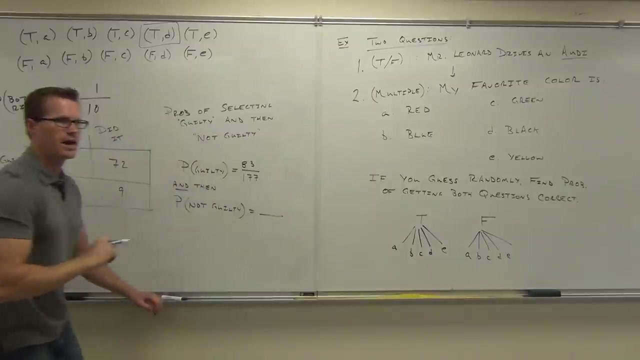 And then the and implies- let's assume that this actually happened- You found someone who was guilty. You took them out of the mix. Can you please tell me how many not guilty people we have to choose from? 94.. 94 people. 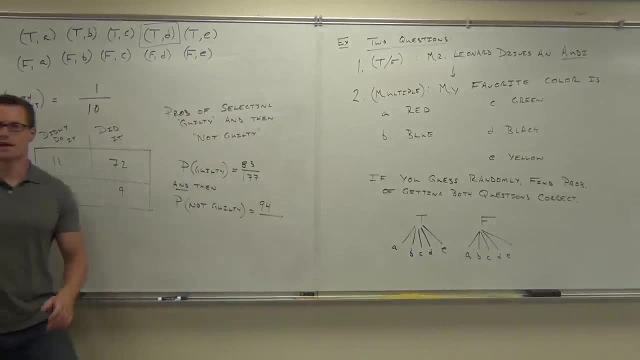 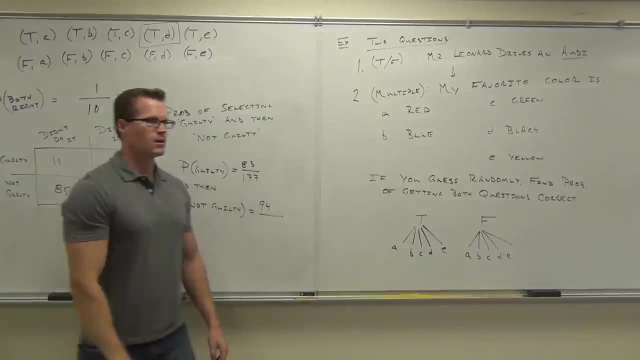 Out of how many? total people? 177.. Okay, hang on, Say that again. How many people? 176.. Why not 177?? 102.. Oh, one guy is now in jail, right, So we pulled that guy out. 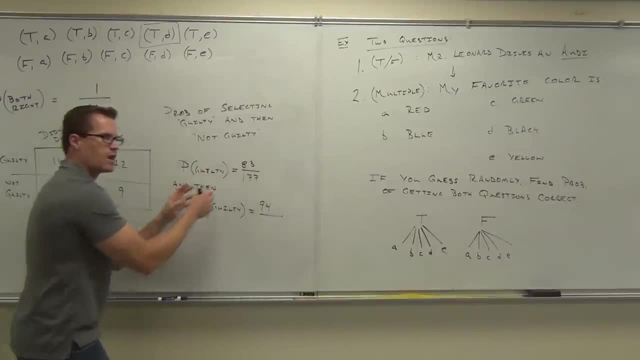 He's gone. We now have instead of 177 people, if we assume. listen, if you're pulling out two people in a row, if you pull out the first guy- and he was guilty- your 83 drops to 82.. 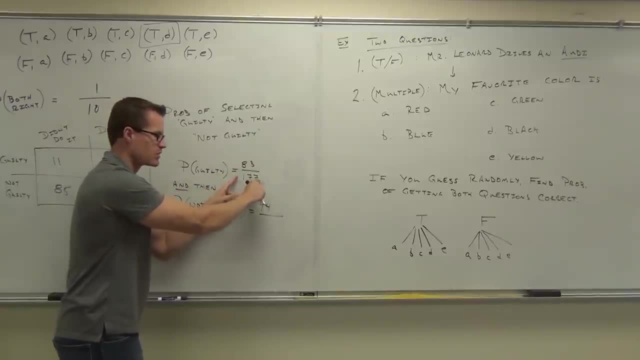 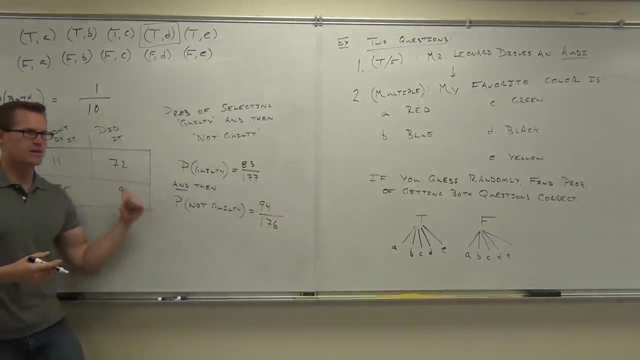 You also pulled one guy out from the 177. So this total drops down. This is now only 176.. You pulled someone out. Now our 94 stays 94.. We didn't pick out a not guilty guy. We picked out the guilty guy. 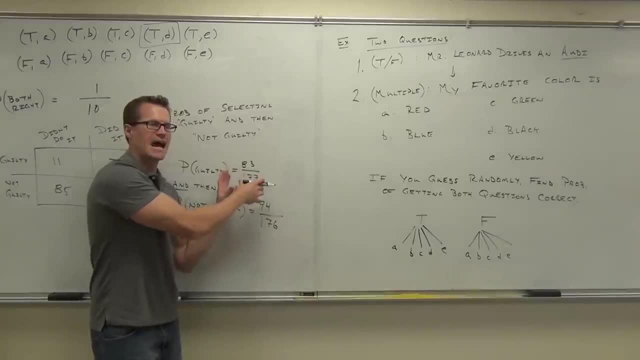 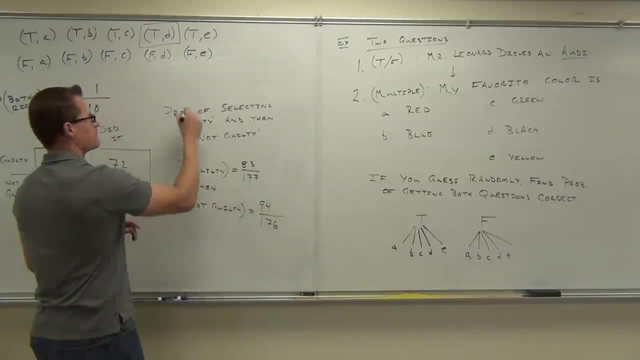 So again, when you're talking about and then notice how your probability can actually change as you go through and do more and more events, Do you guys see what I'm talking about? This would be without replacement. Make sure you know that. 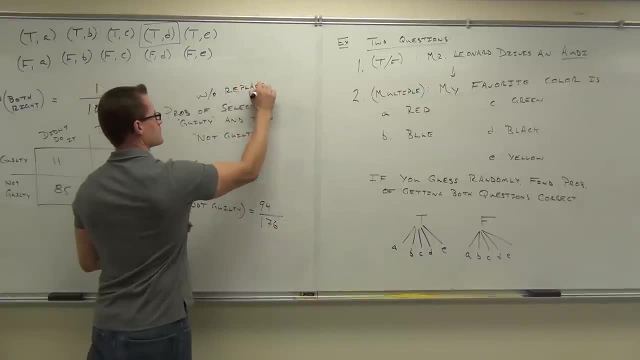 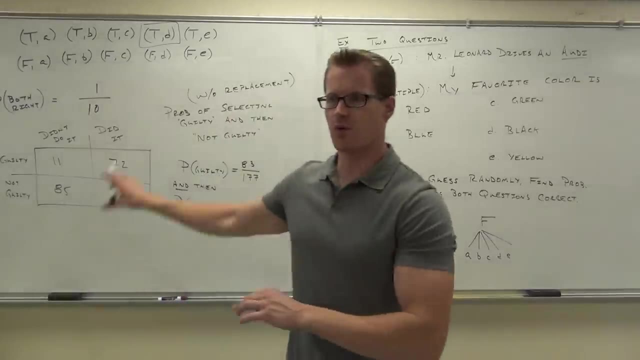 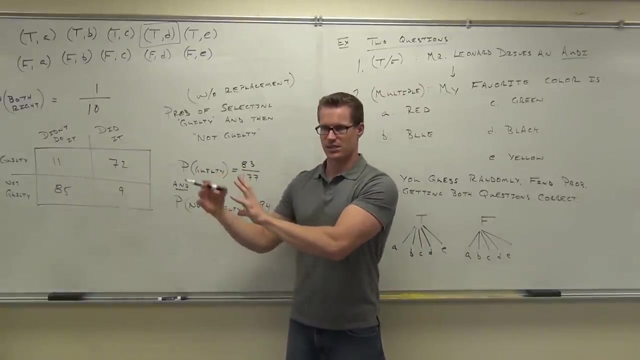 Without replacement. Remember this idea for Friday, because we're going to talk about conditional probability. It's all based on this. For right now, the key things we need to know are that and means, and, And means, and then, like the successive events, probability of one occurring and then another occurring. 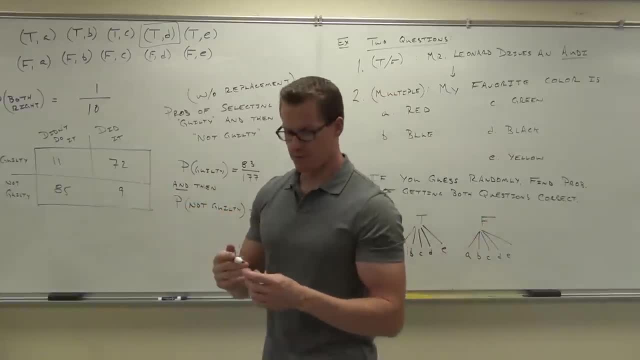 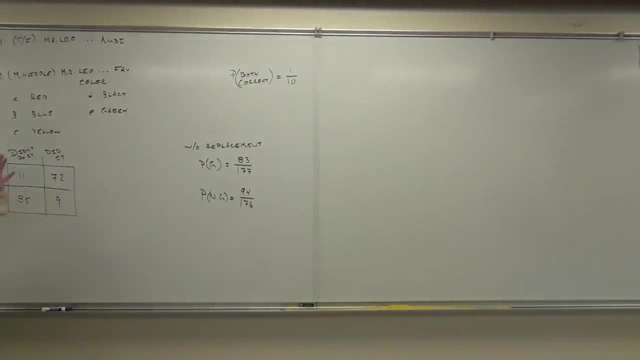 It's different than the addition rule that we just accomplished, And we'll talk about the rest of this stuff next time. So we're talking about this probability And we've realized that, and in this instance means in successive events. So we want something and then something else. 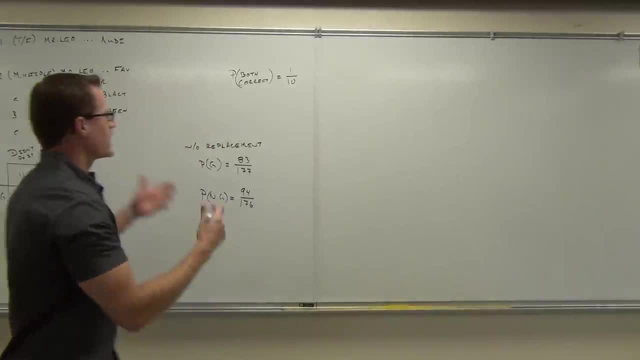 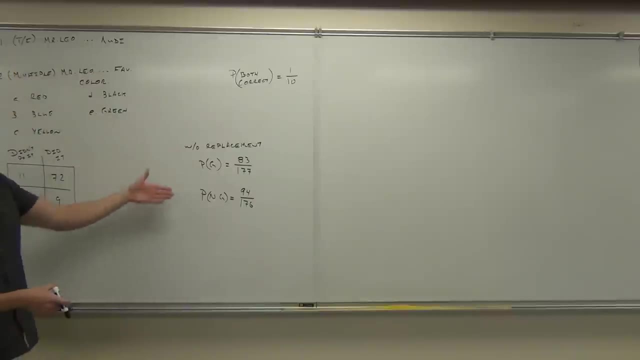 Really the and in the multiplication rule should be. and then- And here we had our probability of answering both these questions right. We figured out last time was 1 tenth Probability of selecting someone guilty we have here and not guilty there. Now, what this leads to, I want you to look at this. 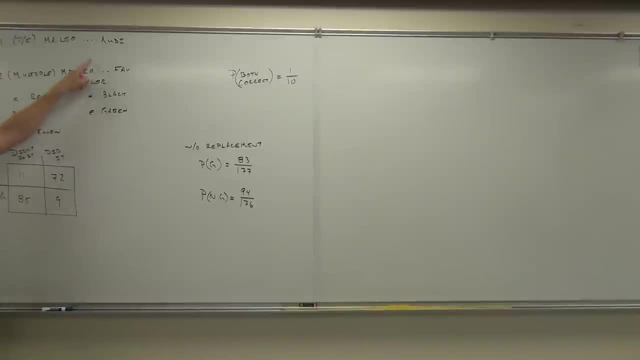 Did this probability of getting this question right or the probability of getting this question right affect the outcome of this question? Did these two questions affect each other? Basically, does answering this question- right or wrong- have anything to do with answering this question right or wrong? 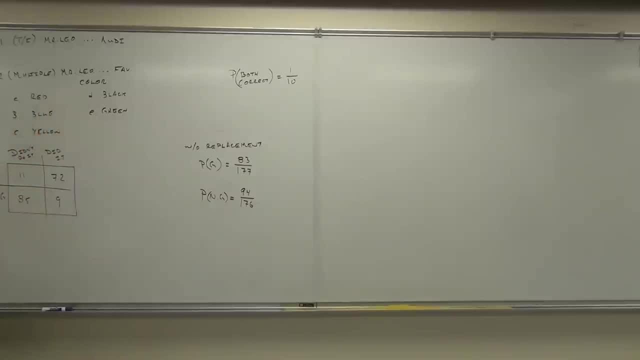 Or getting this the probability of selecting this one right or wrong? That's your question. No, These have nothing to do with each other. However, when you look down here, look at this: Did the probability of selecting someone guilty affect the probability of selecting the next person as not guilty? 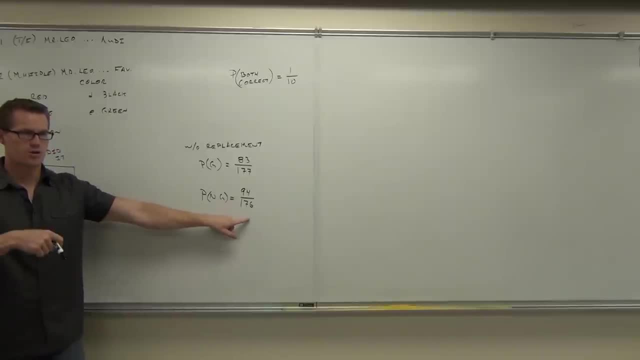 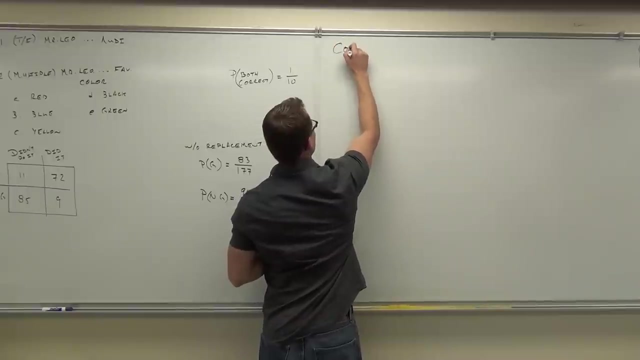 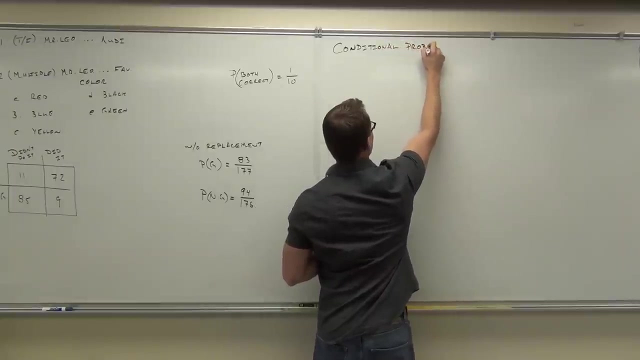 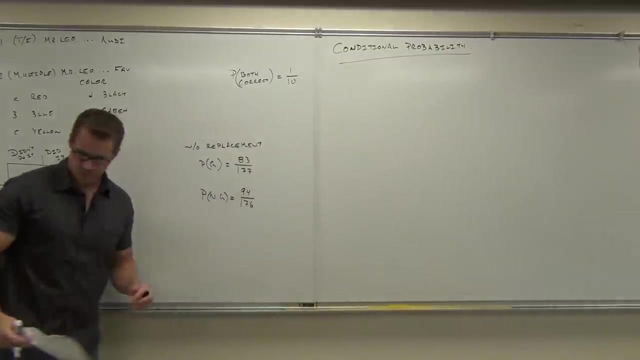 It did, because that number dropped. We took out a person from our sample here. Does that make sense to you? This leads to an idea called conditional probability. We're going to talk about that right now: Conditional probability. Here's what conditional probability is. 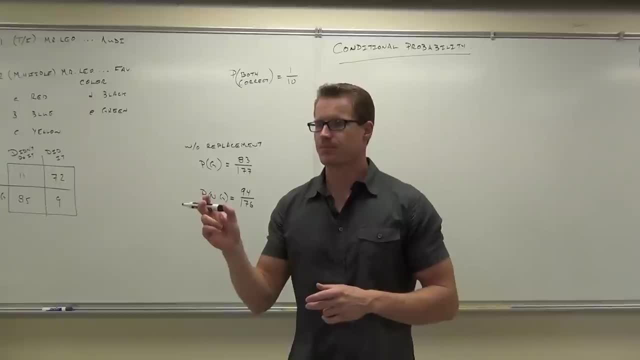 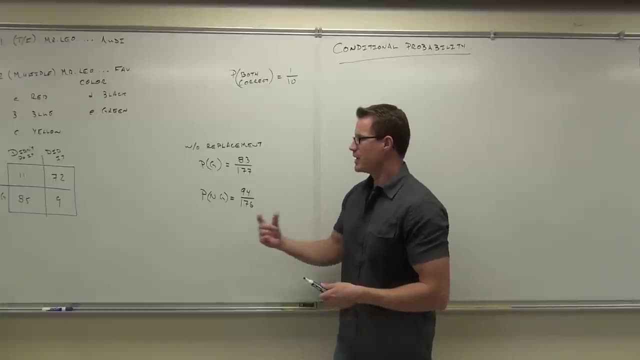 It's the probability of some event occurring, given that another event has already occurred. So in this instance it was: what's the probability of selecting someone who is not guilty, Given that you just selected someone who was guilty? Does that make sense to you? 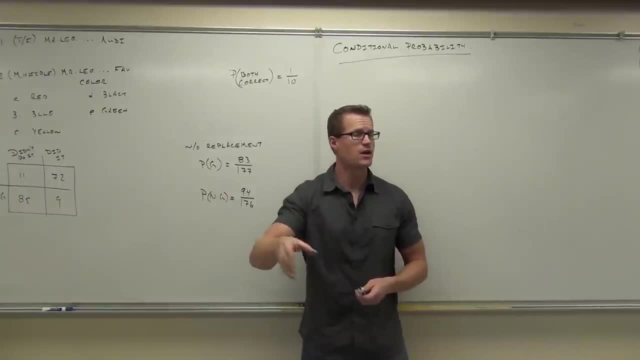 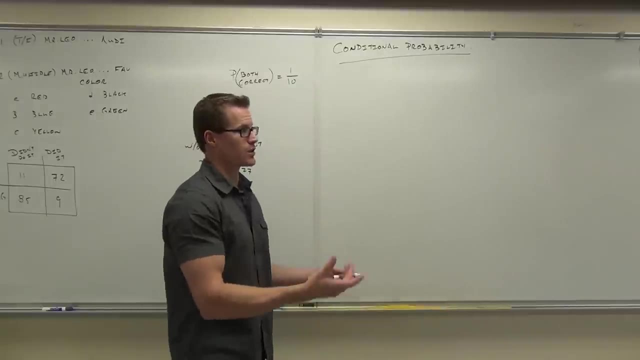 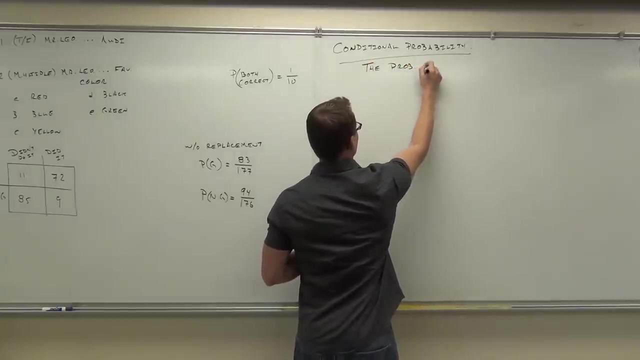 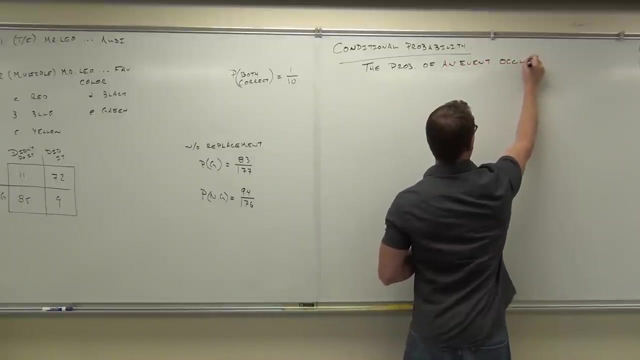 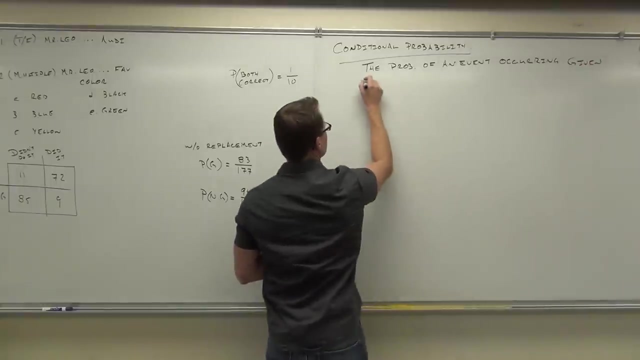 It's conditioned upon some previous event. So when we say conditional probability, we mean the probability of an event occurring given that some other event has already occurred. We know that some of the events occurred in this instance is not guilty, So once again, we're going to look at the probability of selecting someone who is not guilty. 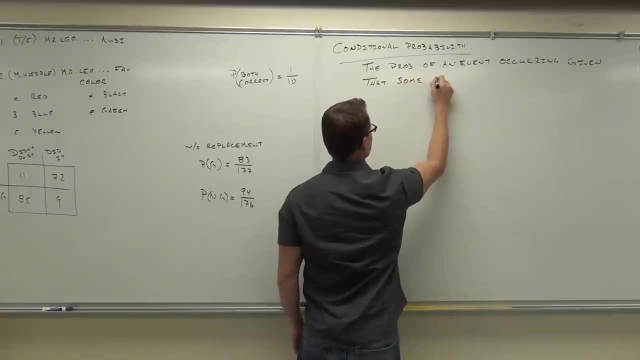 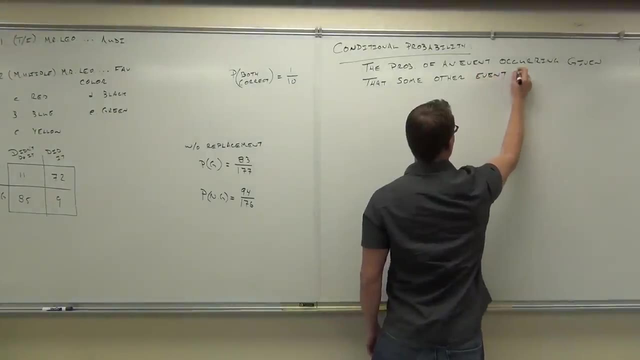 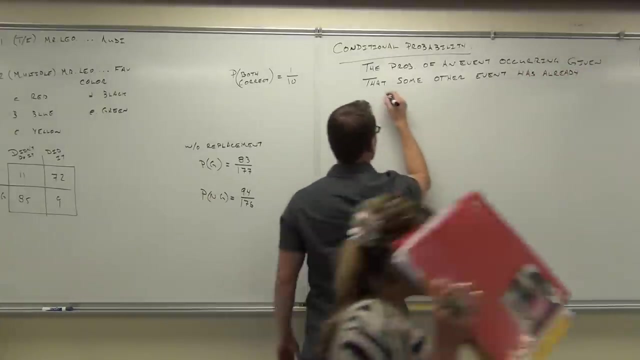 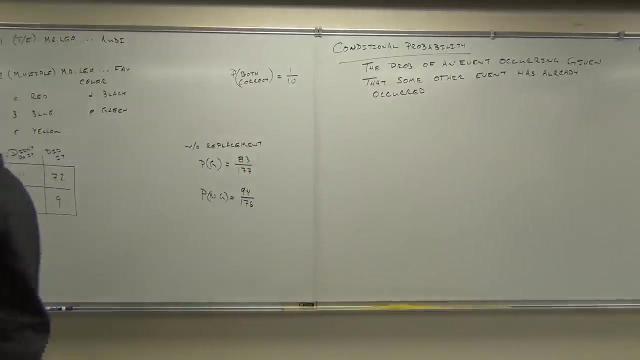 That's the probability of that probability. So in this instance, some of the events occurred in the instance of selecting someone who is not guilty. given that some other event has already occurred, I'm going to go back and find these probabilities individually. 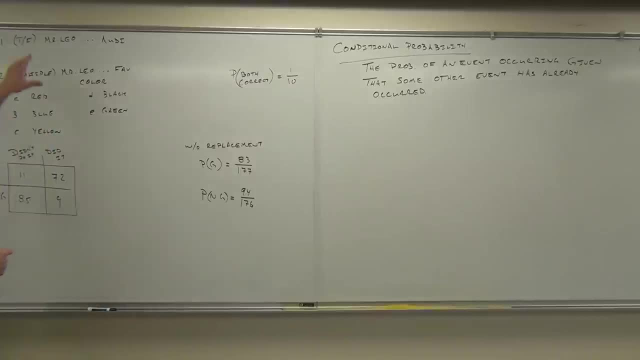 We're going to kind of draw some conclusions from this later. Look up here with me on example number one here. Can you please tell me what's the probability of getting this question correct by guessing? I mean, I told you the answers to these, so you should get 100% on all this, right. 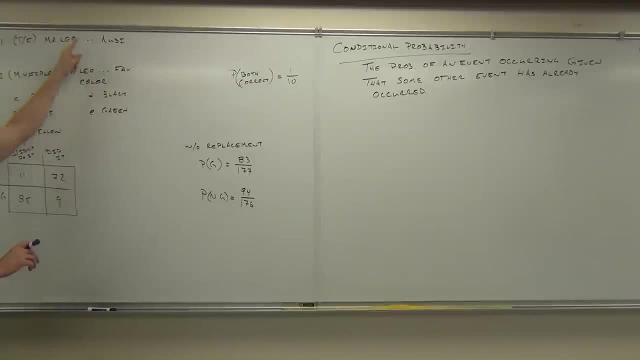 because you know everything about me now, But what's the probability of guessing and getting this answer right? Mr Leonard drives an Audi. Sure, Why? Because there's one correct answer out of how many choices? Sure, What was the probability of guessing this one correct? 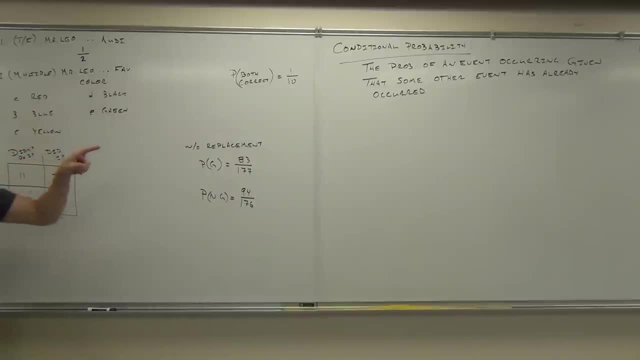 How many choices are right? How many total choices do you have to choose from? Okay, Now, does getting this one right affect this one at all? Okay, so this? we're going to learn about this in just a second. This probability would be one-fifth. 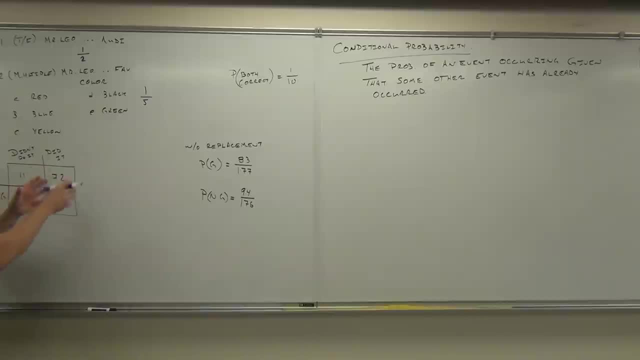 Okay Now in this case we had the probability 83 over 177.. That came from: we had 83 guilty people out of the 177 total. That would be our probability of getting someone guilty. Let's pretend that this didn't happen right now. 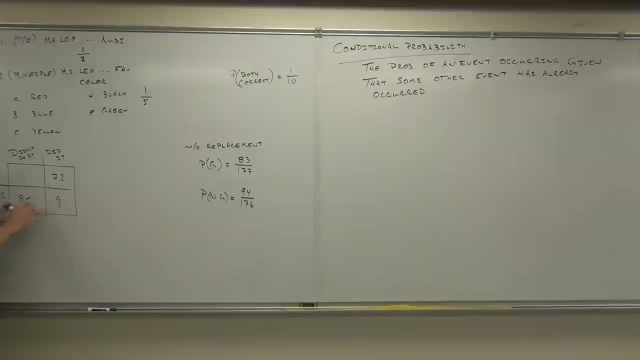 I'm just looking at the probability of not guilty. What I would have is 94 out of 177.. If I just found the probability of selecting one not guilty person, are you with me on that? But after I say this, do this after selecting the guilty person, then that probability drops. 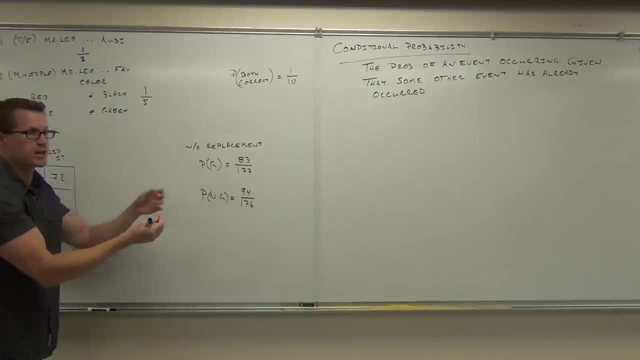 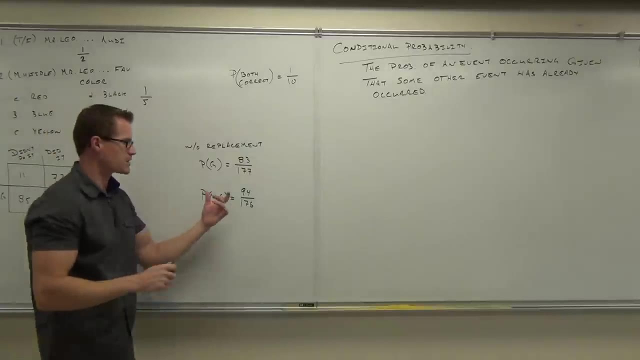 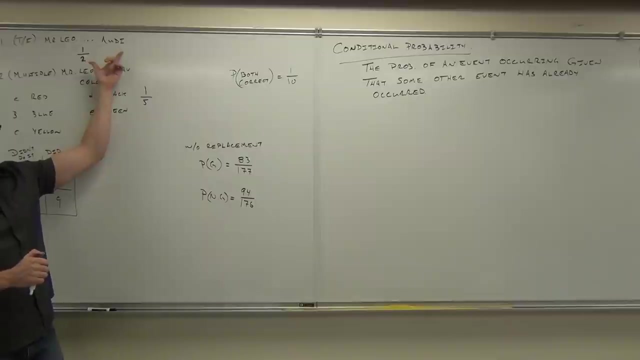 It's conditioned on the fact that you just pulled out a person who was guilty and you kept them out, because we're talking about without replacement. That's the idea of conditional probability. It's that sometimes a probability is dependent on a previous event. Here, this probability really wasn't dependent on a previous event. 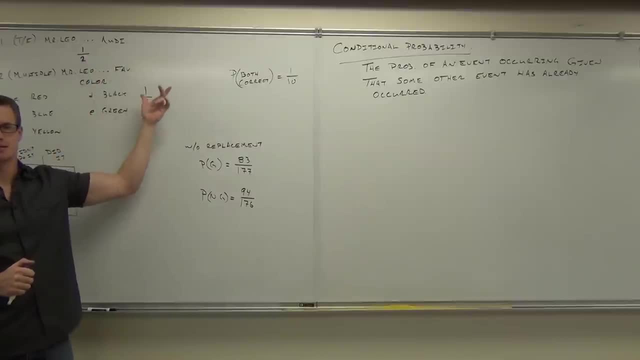 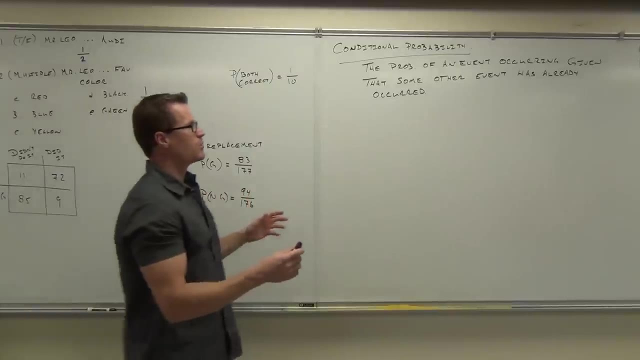 We're going to talk about independent and dependent in just a second. This would be an independent event Here. this one depends on what happened first. right, This is an example of a dependent event. So conditional probability is looking at two probabilities happening and find the probability. 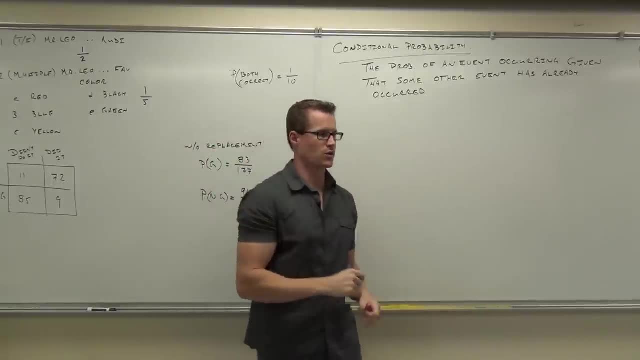 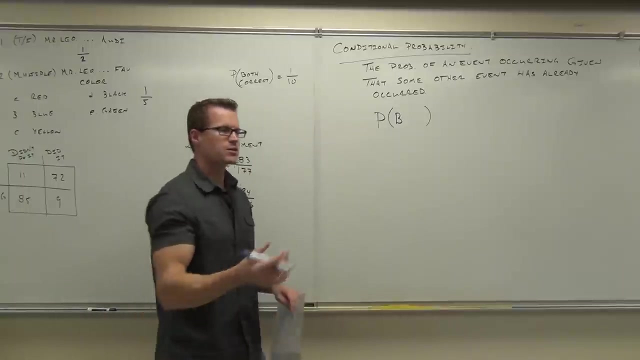 of an event, given that a previous one has already occurred. The way you write that out, it's still a probability, It's just conditional probability. It looks like this: You're going to have some event like event B. You have this vertical line. 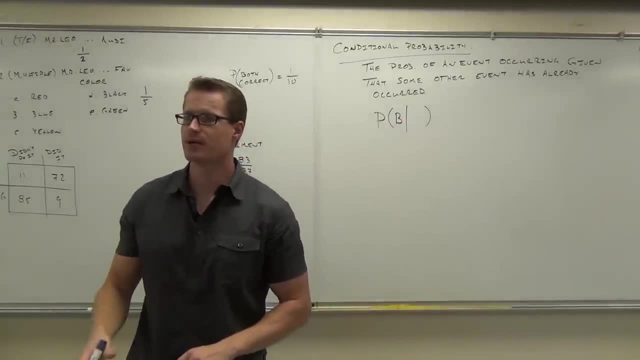 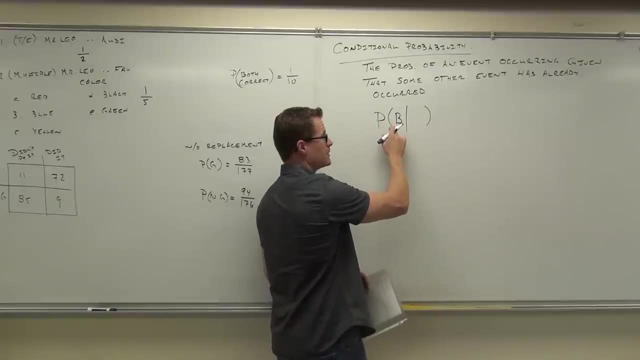 and what this vertical line stands for in statistics and probability is given that. So what this probability says is the probability of event B happening, given that A has already occurred. This is the probability of event B occurring, given that event A has already occurred. 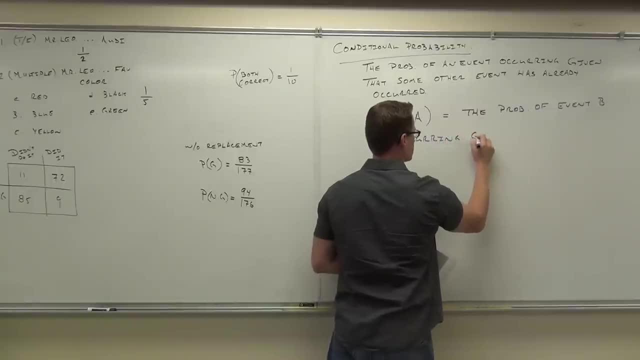 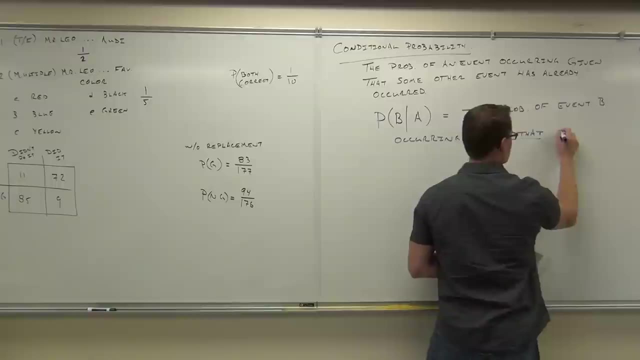 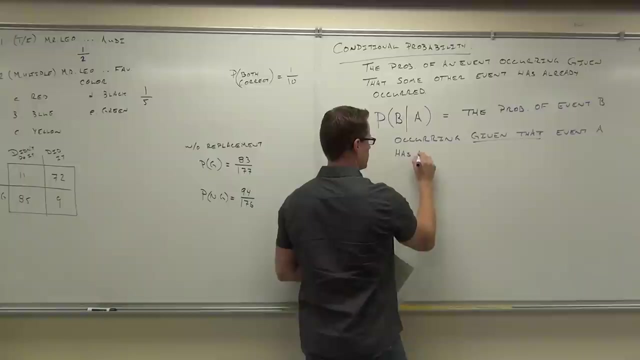 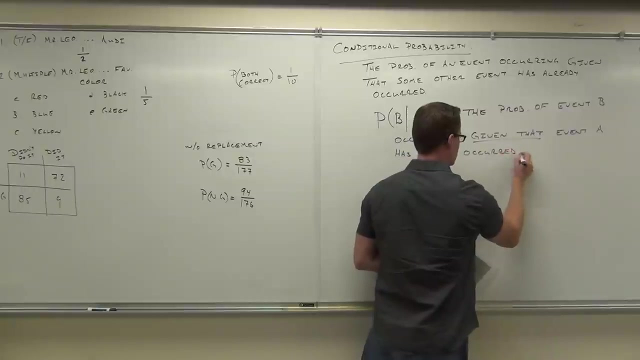 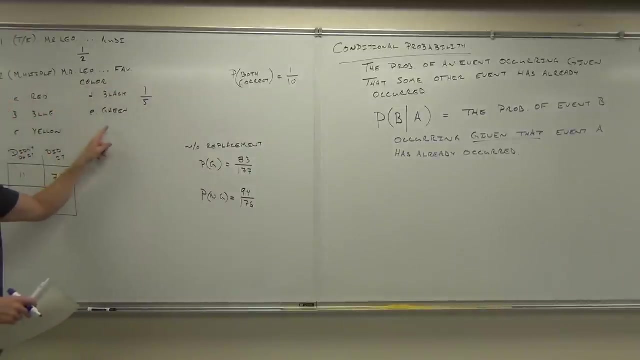 This is the probability of event B happening, given that event A has already occurred. That's what we have in these cases. This is find the probability of getting the color question correct, given that you already got the Aughty one correct, Now the Aughty one doesn't affect the color one. 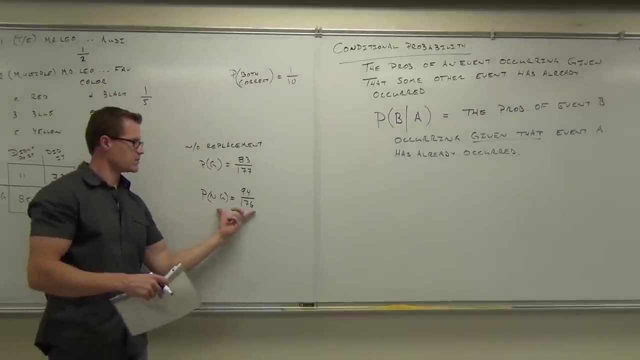 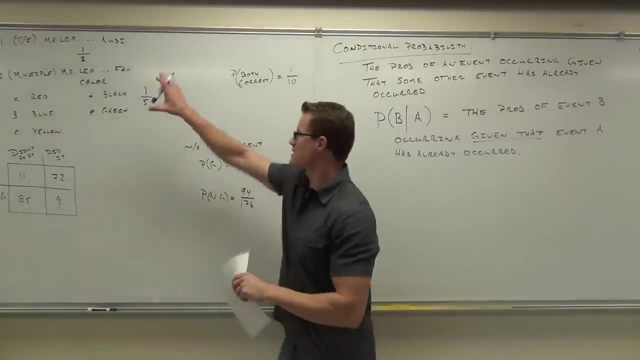 That's not a problem. But here let's find the probability of selecting someone who's not guilty, given that you just selected someone who's guilty And that does affect the probability. So I need you to see the difference. Do you see the difference between this type of problem? 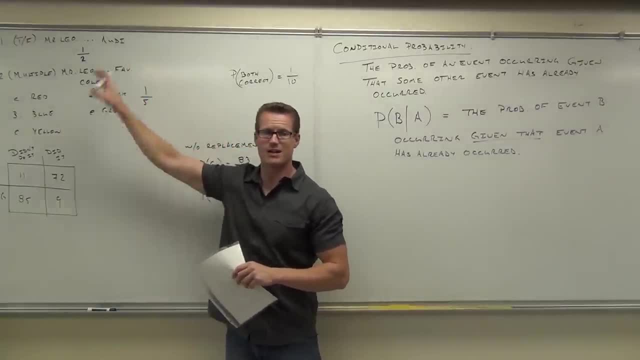 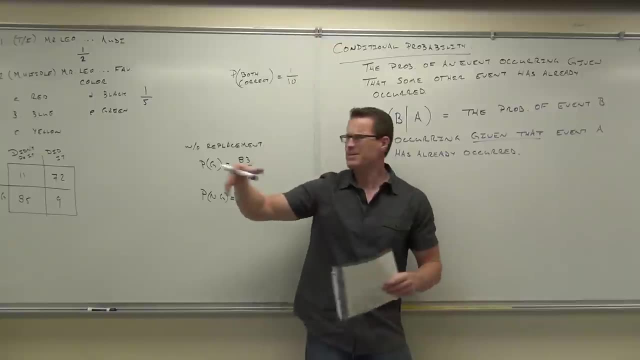 where the one probability does not affect the other one, where one event does not affect the other one and this one where one event certainly did affect the other probability. How many people see that difference there? So sometimes, yeah, we have probabilities. 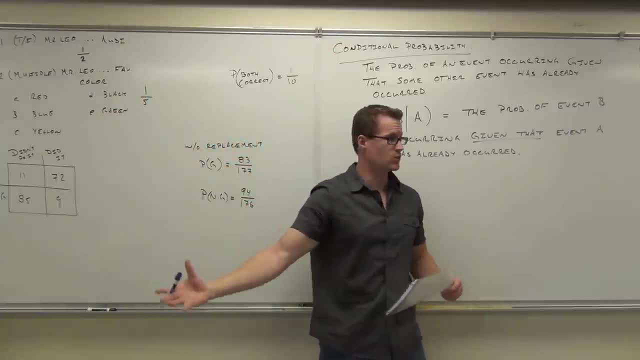 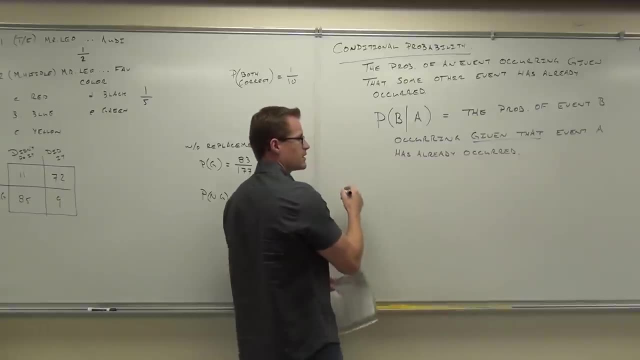 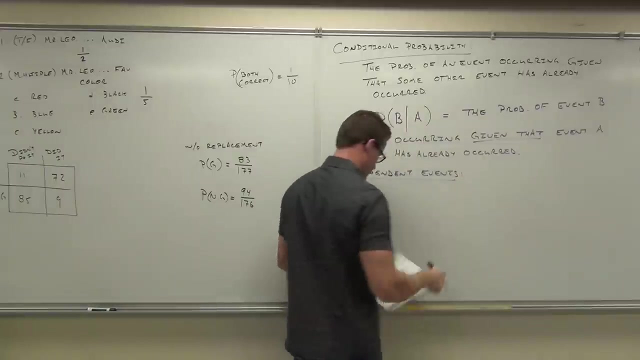 that don't affect each other. Some events don't affect each other at all. Other times we do This without replacement here- certainly affects the second probability. This gives us a definition for what's called independent events. Here's the basic definition for it. 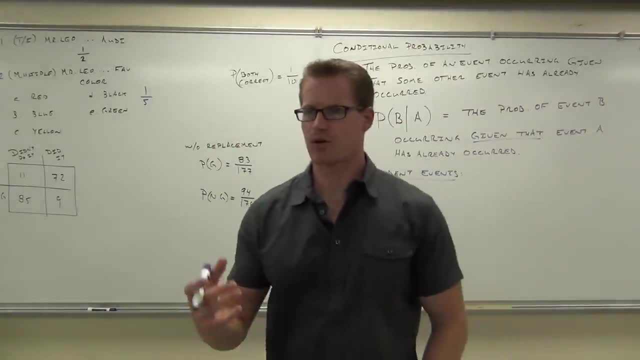 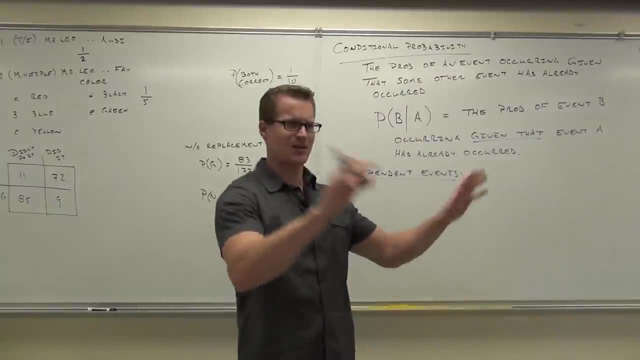 Independent means like if you're independent, you stand alone, right. Independent man or independent woman, stand alone, don't need anybody else, nothing affects me, right? That's kind of what independent means in kind of English, right. 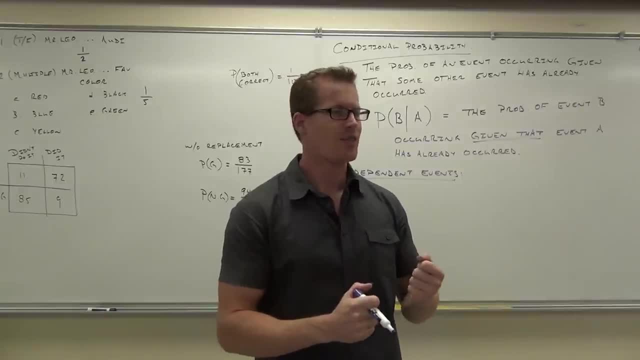 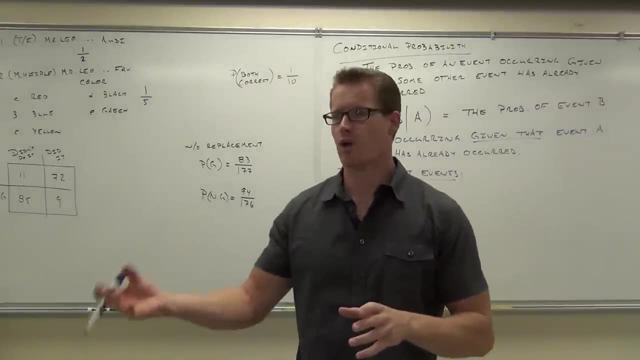 You're by yourself, you don't rely on anything. That's what independent means for probability two: An independent event or events which are independent says the occurrence of one event does not affect the occurrence of another event. Those things would be independent. 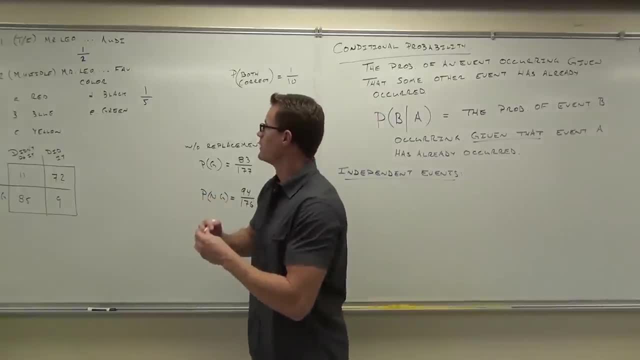 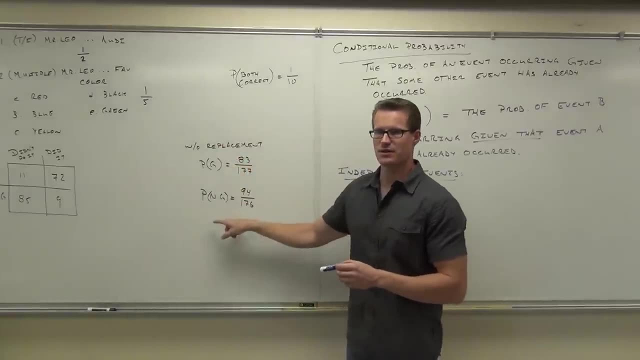 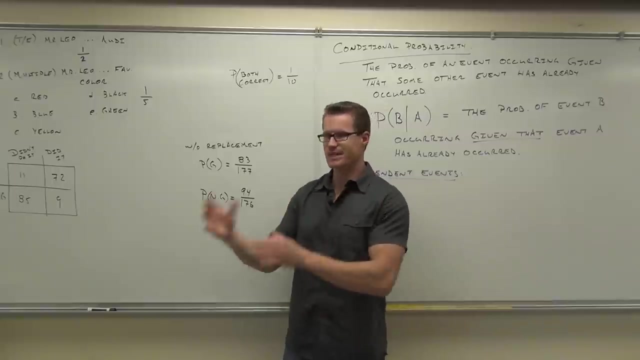 Here's the example I have for you. Okay, It's back here. Does this event affect the outcome of this event? Does this event affect the outcome of this event? That's the difference between dependent and independent. Events which are not independent are dependent. 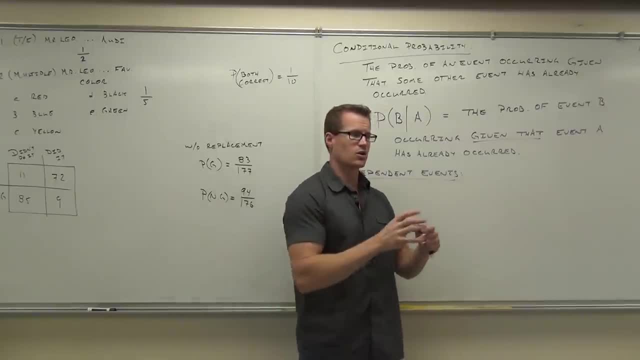 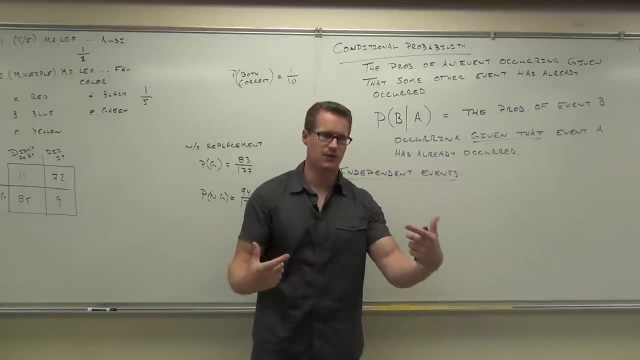 You have to do one or the other. Okay, So, independent events: the occurrence of one event does not affect the occurrence of another. Dependent events: the occurrence of one event does So when we're talking about independent events. that's what we're going to write down. 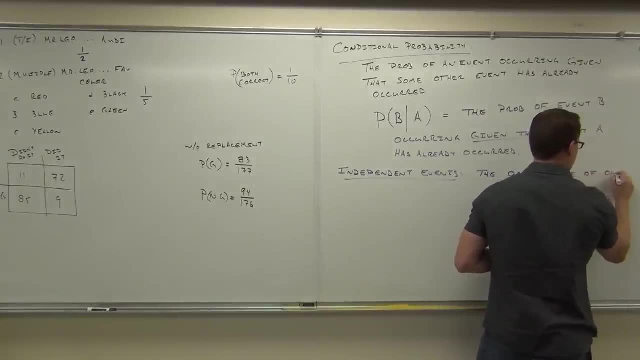 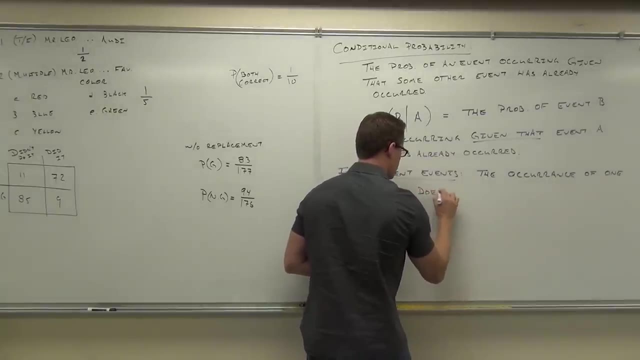 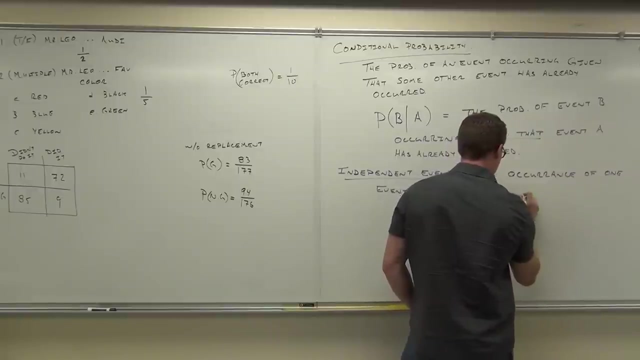 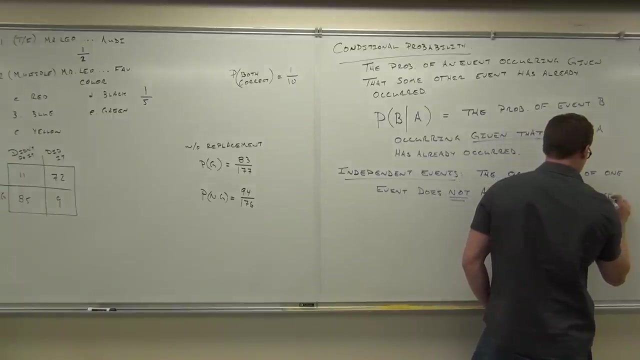 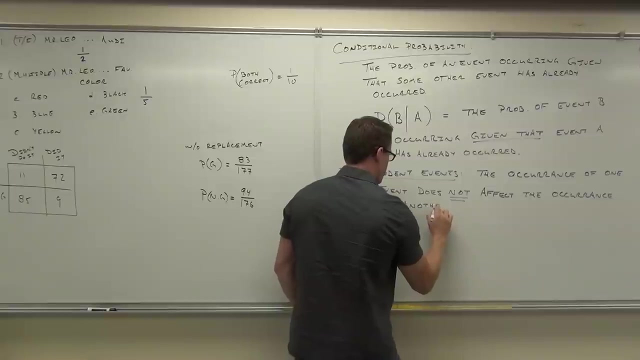 The occurrence of one event Does not affect the occurrence of another event, Or I should say probably subsequent event, one after the other. One of them doesn't affect the other one. Okay, Okay, Okay, Okay, Okay, Okay Okay. 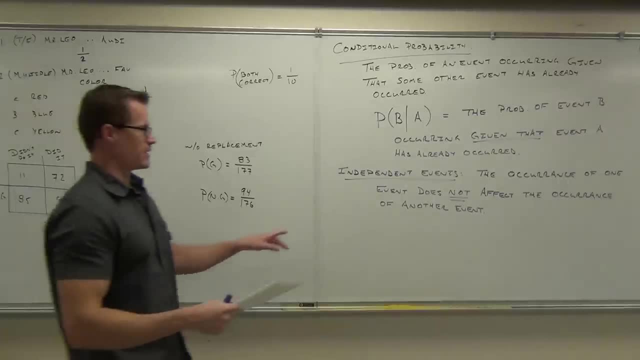 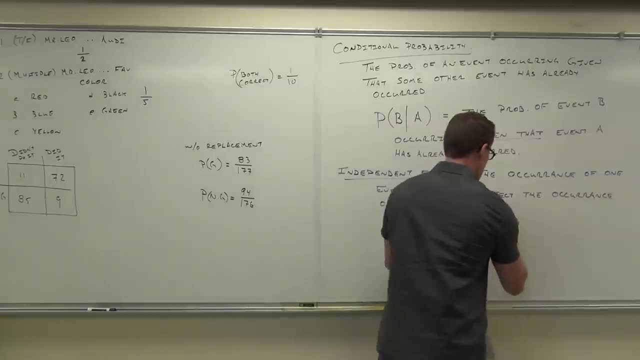 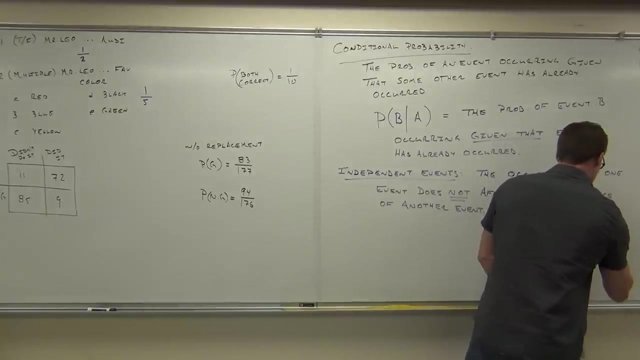 You have to be in one class or the other. So non-independent events are dependent. Wait a minute, leave early. you wouldn't get your money's worth if it was early. Pedro, Come on, man Tuition's going up. 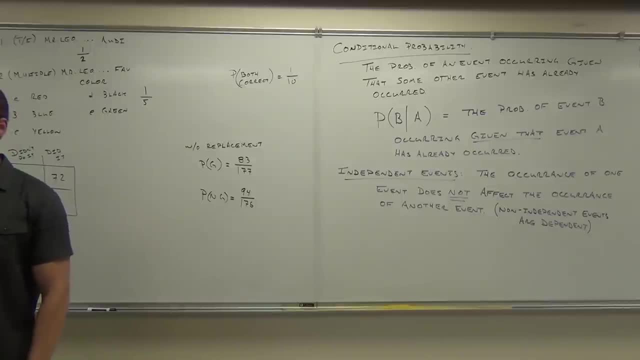 You should be getting even more bang for your buck, right? Say yes, Yes, Yes, That means we should stay here later. obviously, That was a good try, right, Good try, Okay. so independent events don't affect each other. 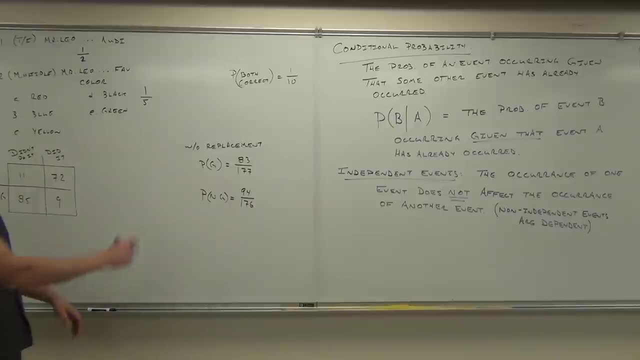 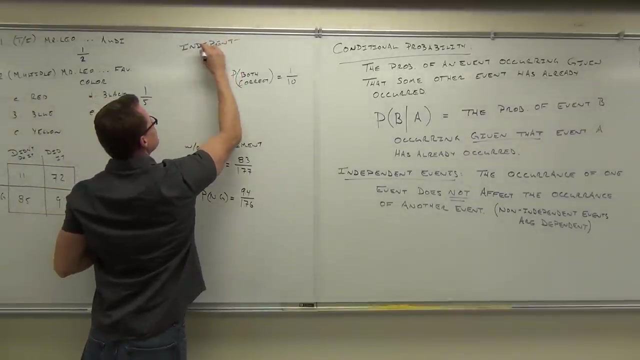 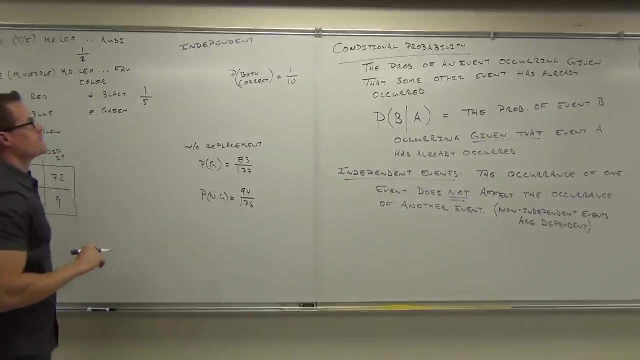 Independent events do affect each other. Again, we're going to list these out over here. This is definitely independent as far as the events go. These do not affect each other. The outcome of this one did not affect the probability of this one. 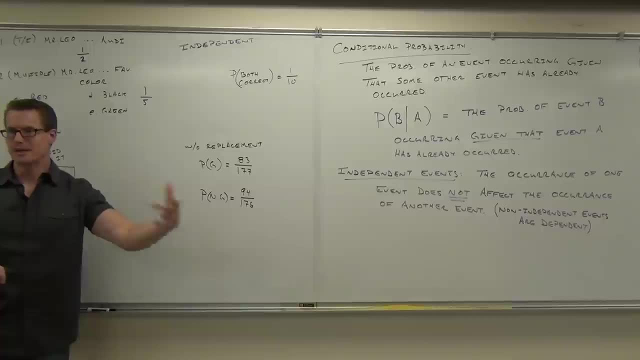 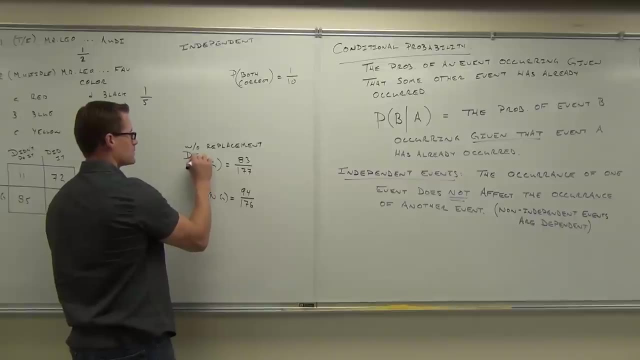 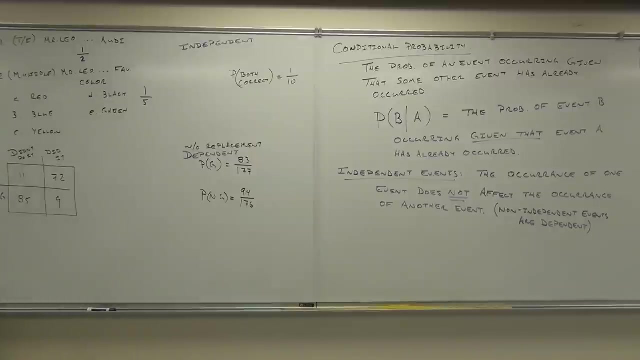 Down here. it definitely did. That's what that was, Okay. so the general replacement generally means they're dependent. You're taking one away from your sample. I mean the probability is going to change. This is definitely dependent. Hey, by the way, one little note. 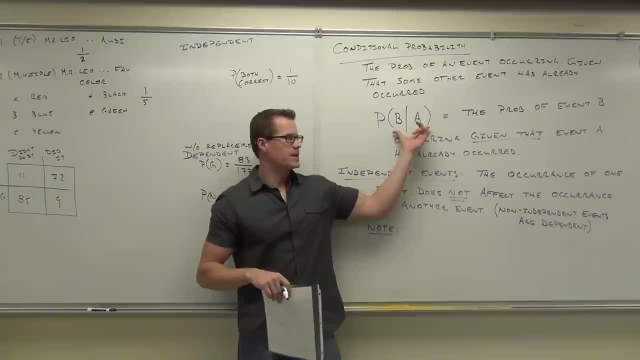 Let's suppose for a second that A and B are independent. Remember, this means the probability of B occurring. given that A's occurred, Let's say they're independent. Let's say that they have nothing to do with one another, like this example. 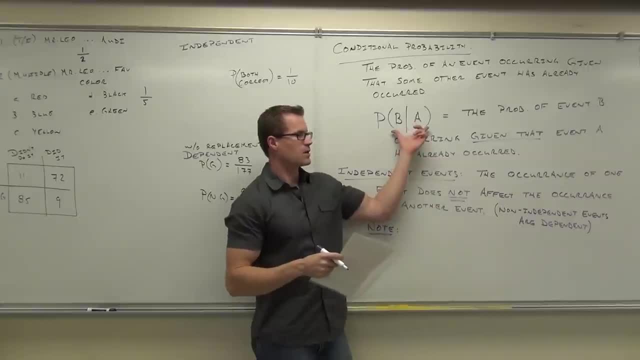 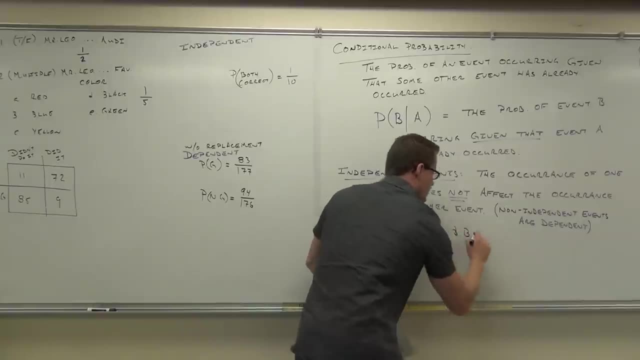 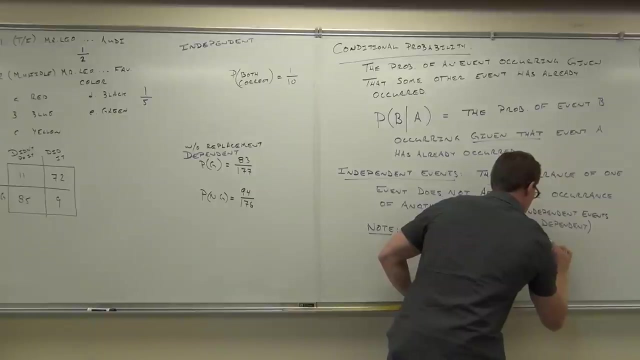 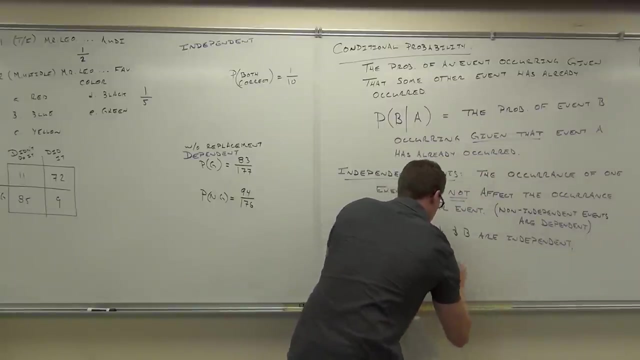 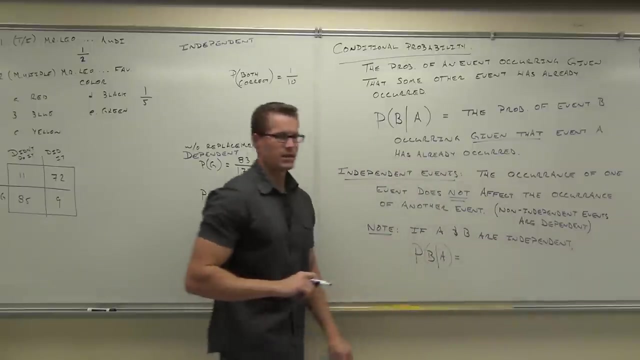 where number one didn't affect number two. If these things are independent, if A and B are independent, if A and B are independent, tell me what that equals. Think about it. Does A, if events A and or? you understand that independent? 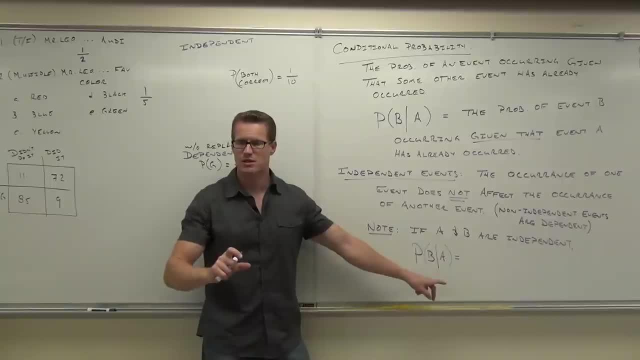 if things are independent, does A affect B? Okay, so here's the question: If A does not affect B, what's the probability of event B happening, given that A's already occurred? If you're not quite catching on to this, let me answer this question. 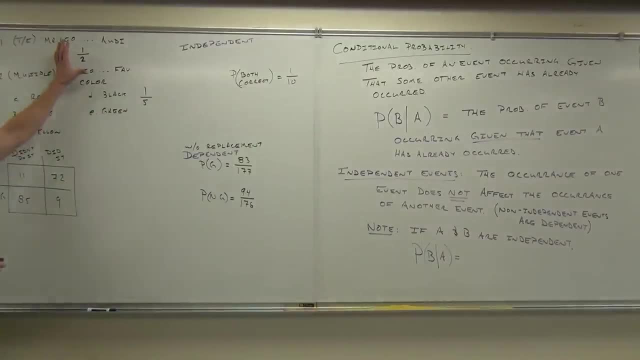 All right, You're answering these questions in order. true, You're going to answer this one, then you're going to answer this one. Let me ask this, Let me answer this. Let's see, you did this in order and you say, okay, I answered this one. 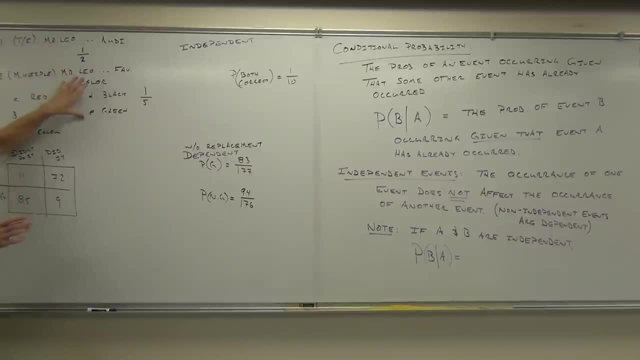 Got it right. got it wrong doesn't matter. Does it affect your outcome for this one? What if I just asked you this one? if I asked you this independently, just by itself? forget problem one if I asked you this by itself. 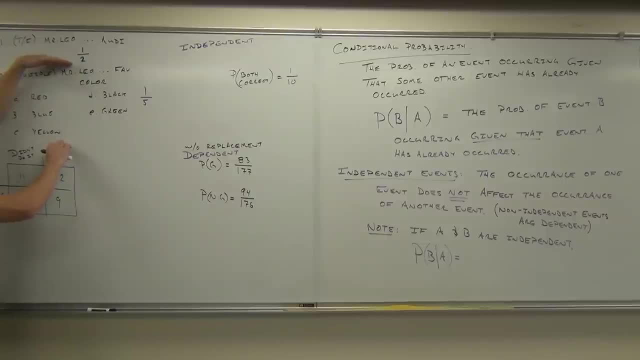 what would the probability be that you get it right? Say that again: One out of five. One out of five. Are you all okay with that? This is one out of five. There's only one right answer. There's five choices. 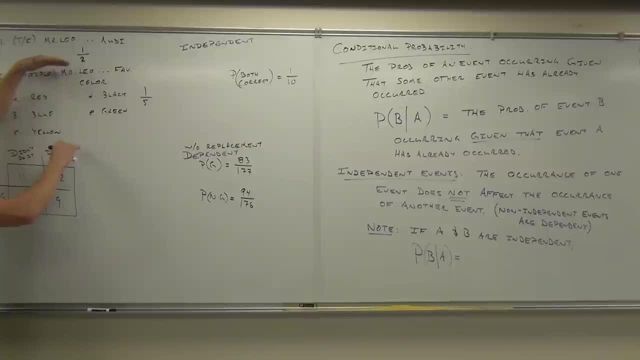 One-fifth is our answer. This is not a hard probability. Don't overthink this. The probability of just getting this one right is one out of five. It's one-fifth true. Now do this. What's the probability of getting this one right, given that you just got this one right? 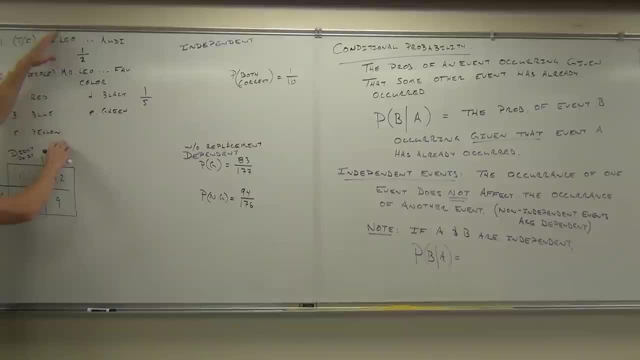 One-fifth. Is it still one-fifth? Did getting this one right change this probability? So apply that to this concept. What's the probability of getting this one right? given that you got this one right, It's the same thing as just getting this one right. 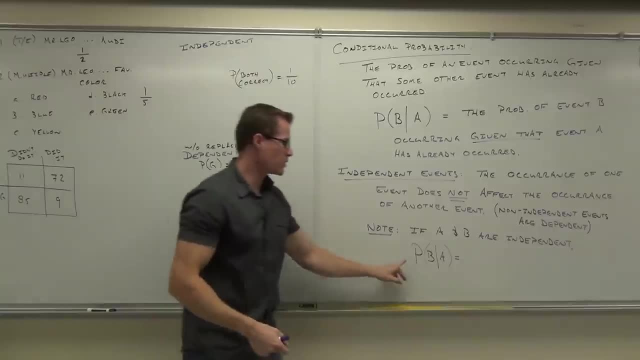 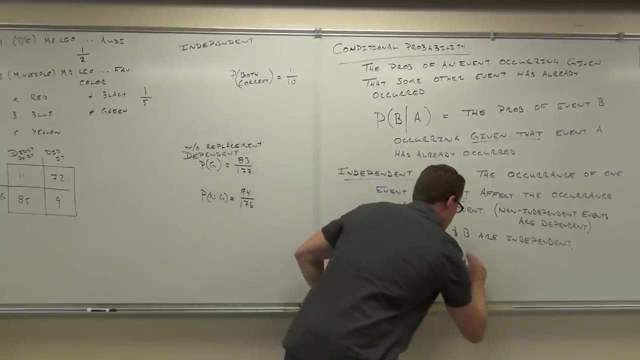 Does that make sense? They don't affect each other, They're independent. So what's the probability of B, Given that A has occurred? if these things are independent, The probability of B? Say that louder. Probability of B, It's the same thing. 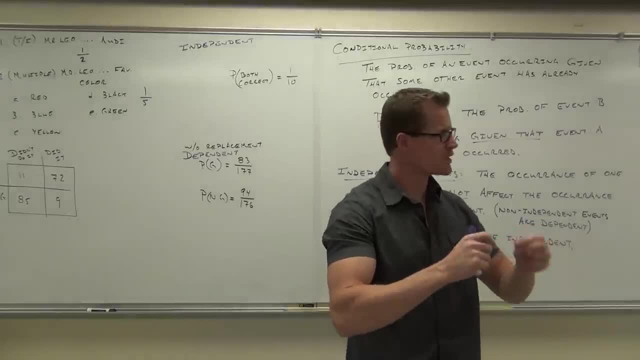 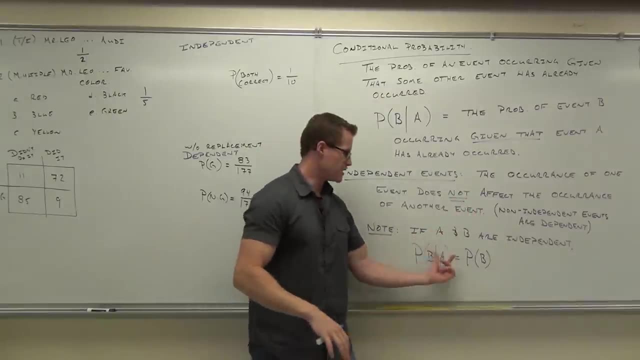 Let that sink in a little bit. That kind of has to make sense to you, Otherwise you really don't understand the idea of independence. So if two things are independent, they don't affect each other at all, right, So what's the probability of B happening, given that A has occurred? 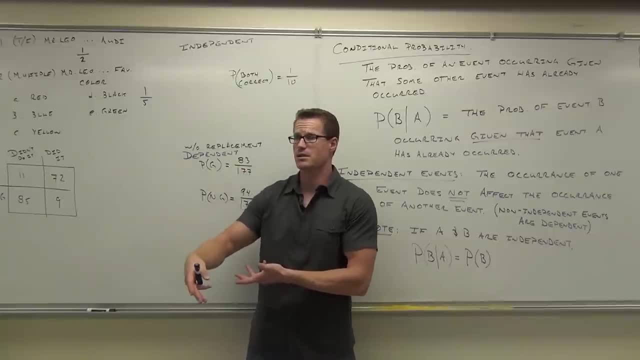 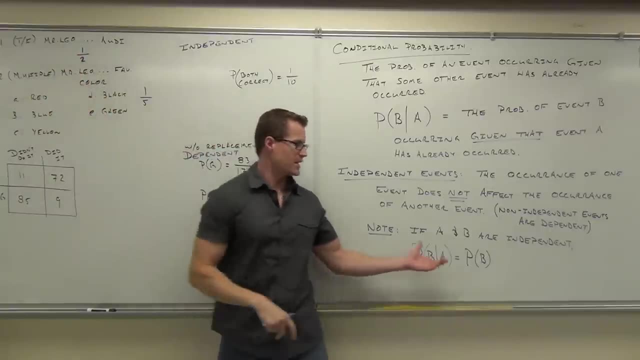 It doesn't even matter if A has occurred or not. right A is not affecting B. It didn't even matter that you got this right or wrong. It's not affecting number two. Does this make sense to you? So in this case, if you have independent events? I hope you're seeing that. 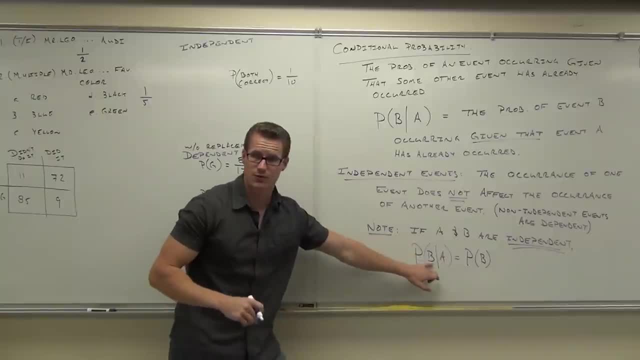 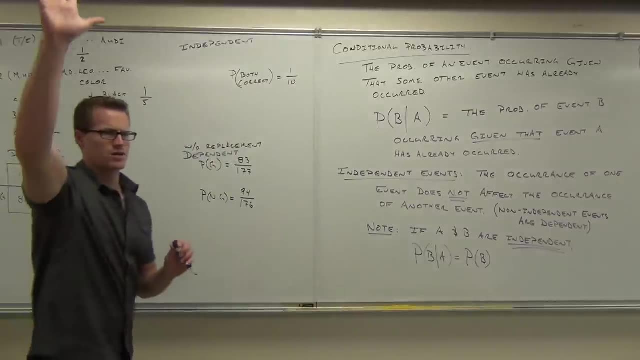 If you have independent events, this one is not affecting this one. Therefore, the probability is just B itself. It's not being influenced by A, That's if the events are independent. How many of you understood that? Raise your hand if you are. 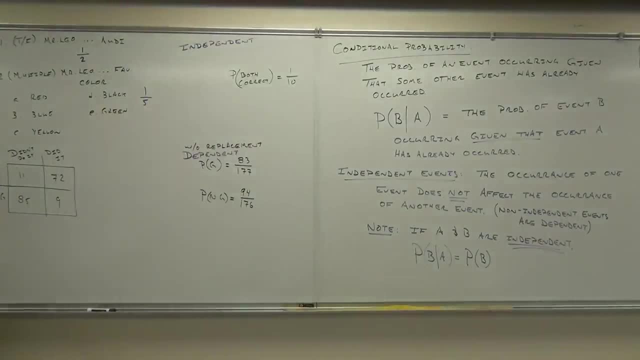 Good, All right, Let's try a couple of examples here just to illustrate this. I'm going to come back on this side of the board and we're going to kind of make up the multiplication rule just by looking at this. So I'm going to erase this. 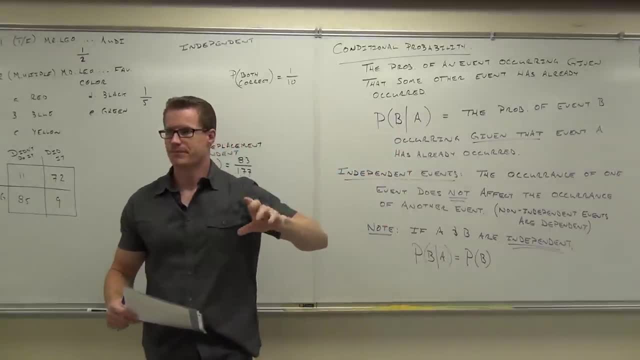 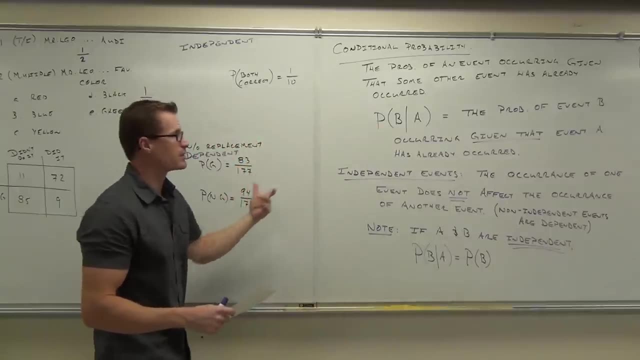 Are there any questions on our conditional probability? So conditional probability simply means that the probability of one event occurring given that some other event has already happened. that's written like this: This means the probability of B occurring, given A has already happened. 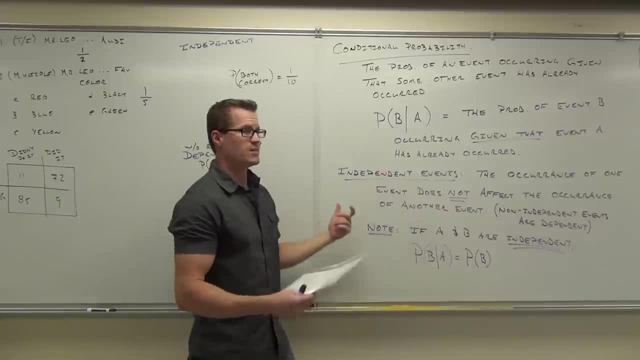 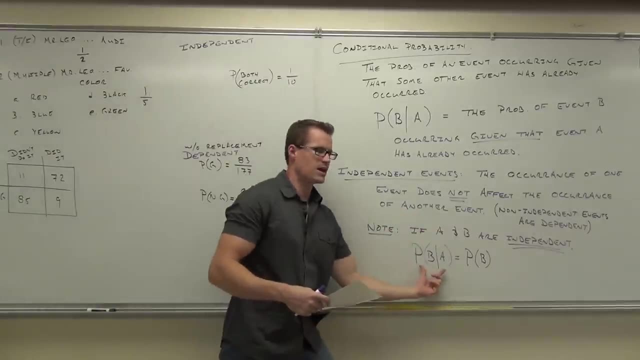 This is what that means: B given A. If they're independent, if they're not related in any way, if one does not affect the other, such as this case, then the probability of B given A is just the probability of B, because A is not. 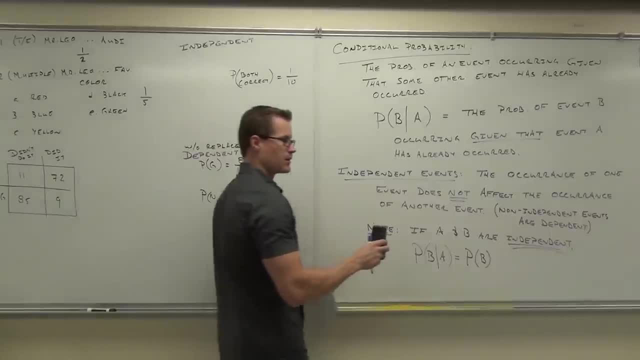 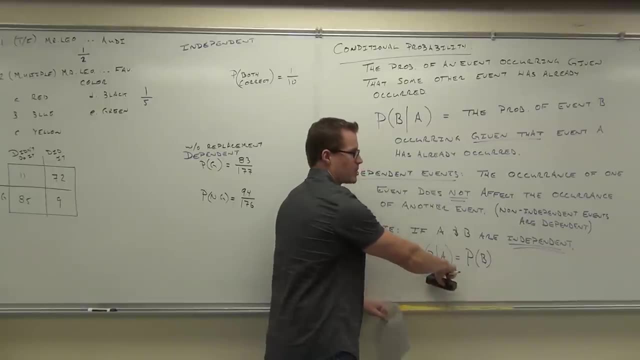 Now let's go ahead and look at a couple of examples. Is it also the probability of A? or just Wait for this one? Yeah, No, this is talking about the probability of this event happening. This one's already happened. 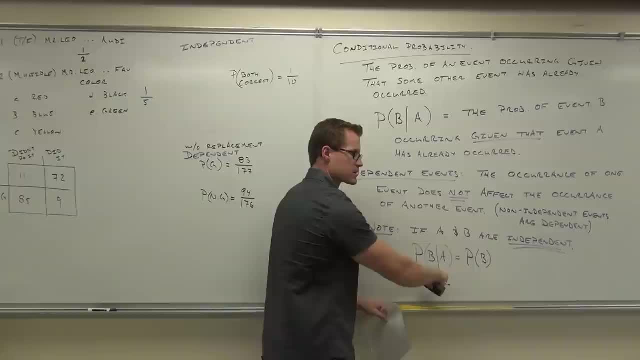 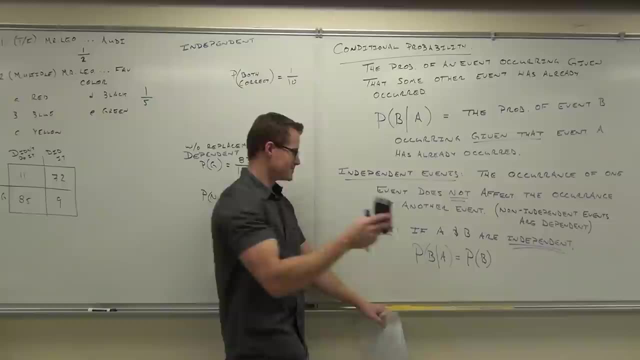 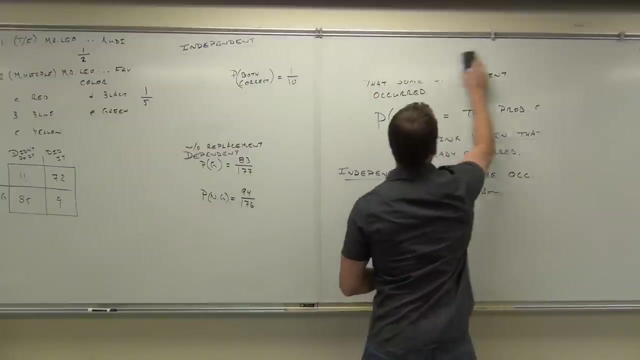 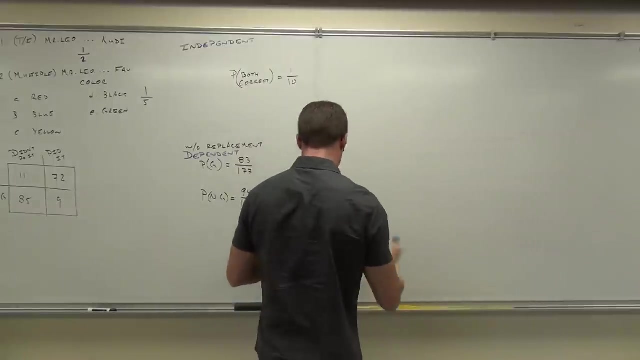 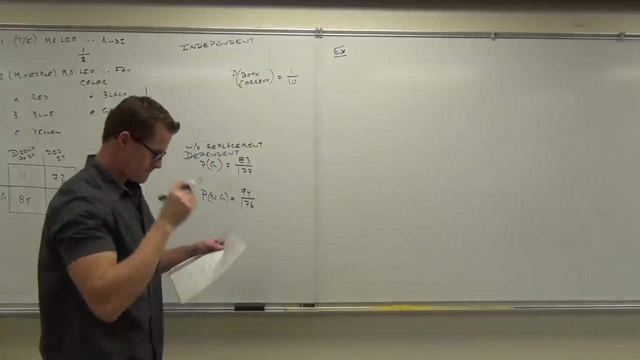 This is in the past, Okay, So we're looking really for event B in this case. That's a good question. Any other good questions before we move on? Any other bad questions before we move on? Okay, We're going to roll a die. 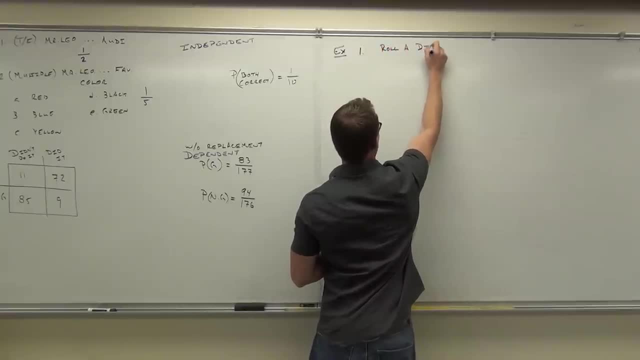 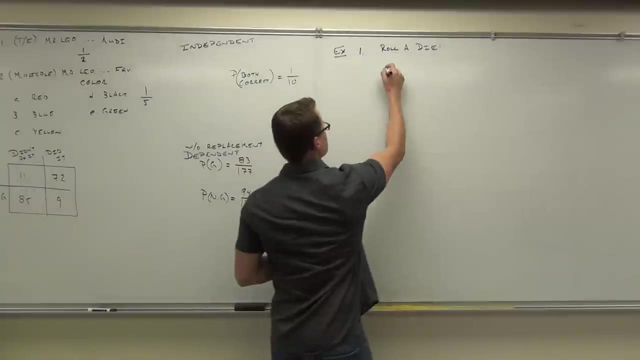 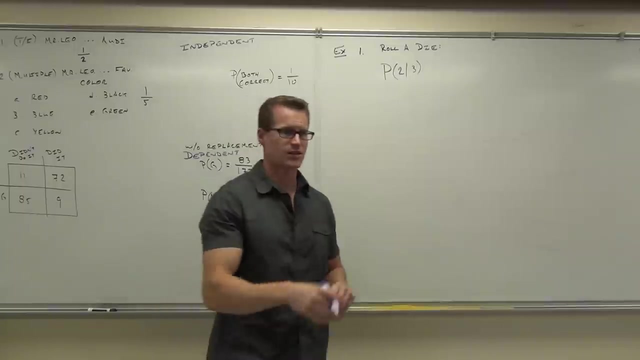 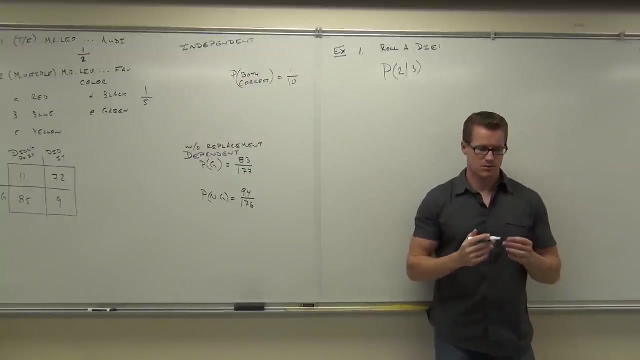 First thing I need you to understand is what this means. If we're rolling a die, this is in the context of a dice roll or a die roll. This says: read that aloud to me. What's that say in English? Probability of B- to have a probability of B happening. 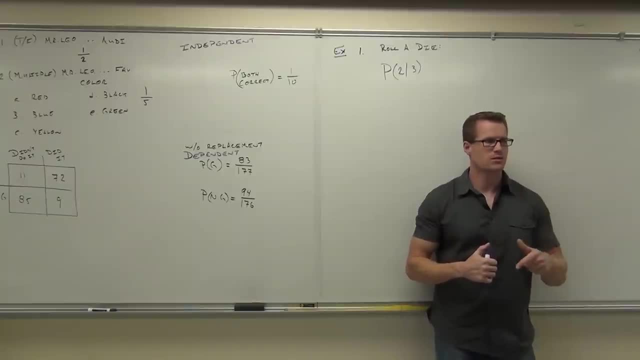 Good, Say that louder so I can hear you. Probability of B to have a probability of B happening. Probability of B to have a probability of B happening. Okay, Perfect. Probability of rolling a 2, given that you just rolled a 3.. 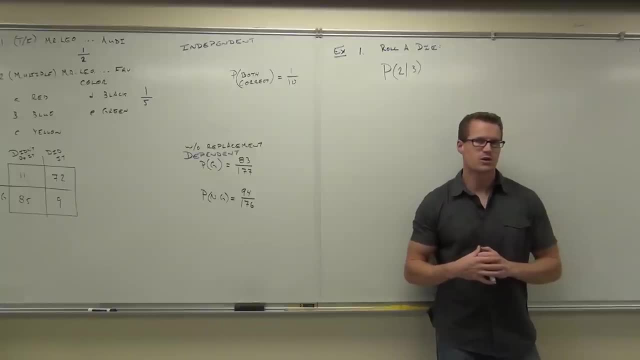 Which one happened first in this case? Did you roll the 2 first or the 3 first, 3.. So here's what happened: You took out your die and you rolled it, And what'd you get? 3.. 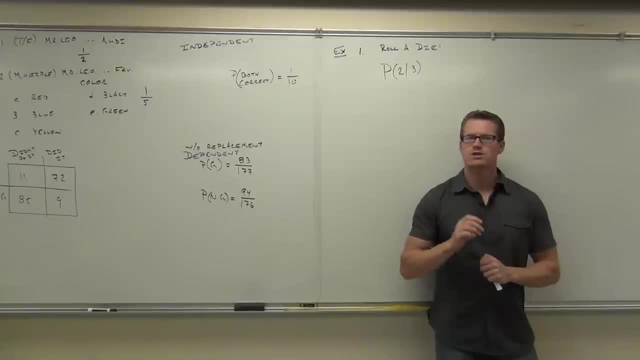 Now you pick up that die again and you're rolling it again. What's the probability that you're going to get a 2?? What's the probability that you're going to get a 2, given that you just rolled 3?? 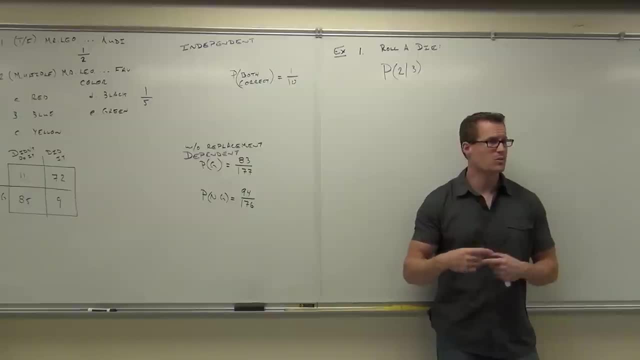 Did it change? No, because you can roll a die as many times as you want to, The probability's always the same, right, That's the same. That's why die are so nice. The probability stays the same, no matter what. 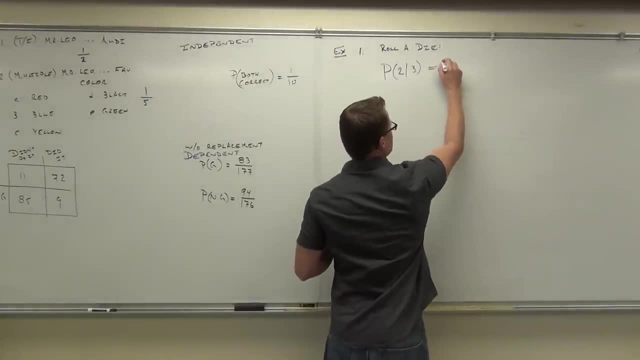 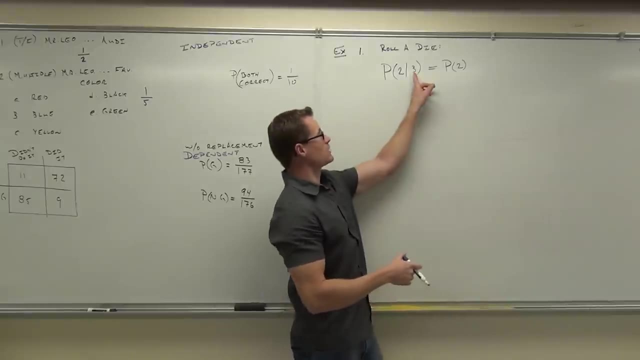 So this is the same thing as just the probability of 2.. What does that tell you about these events? Are they independent or dependent? Independent: Good, Did the 3,? did rolling a 3 affect the probability of rolling a 2?? 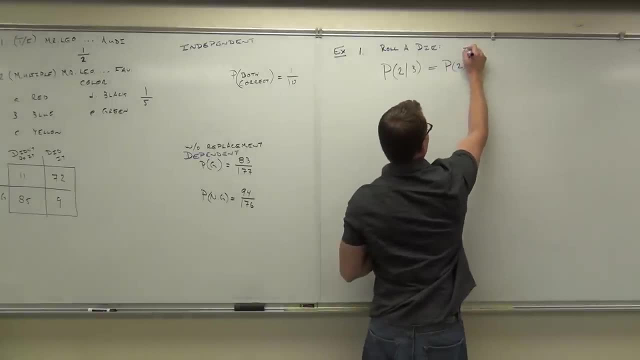 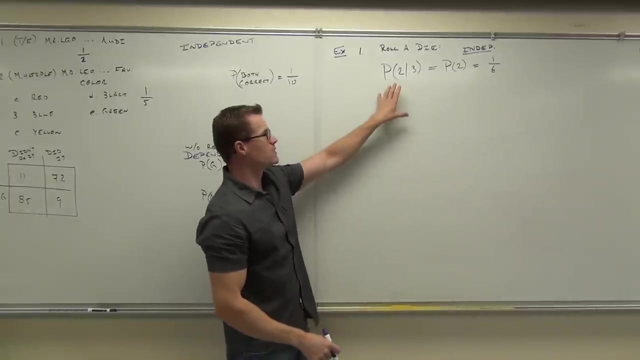 No, No, That means they're independent. That's a weird looking N Independent. So we just have 1, 6.. The probability of rolling a 2, given you rolled a 3, it doesn't change, It's still just 1, 6.. 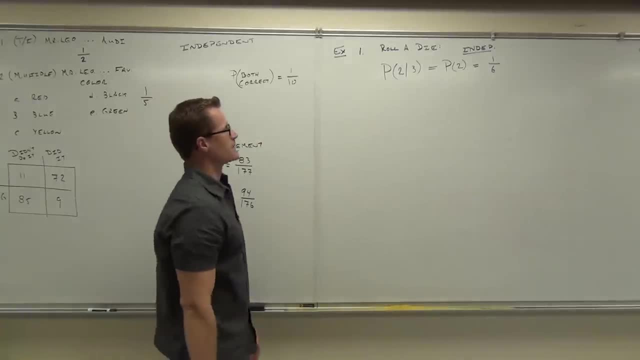 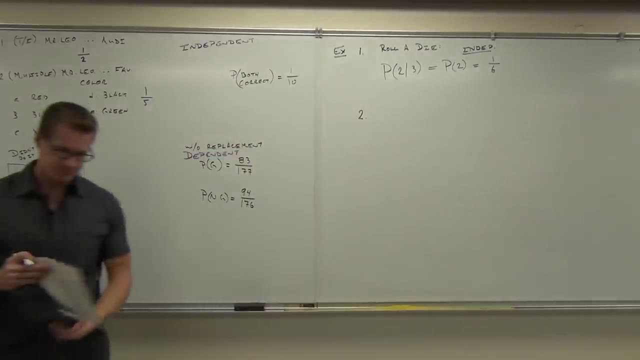 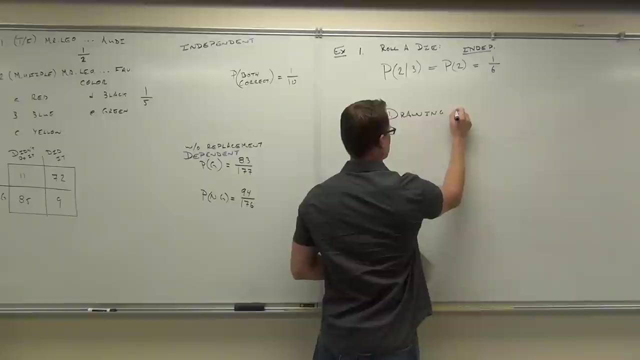 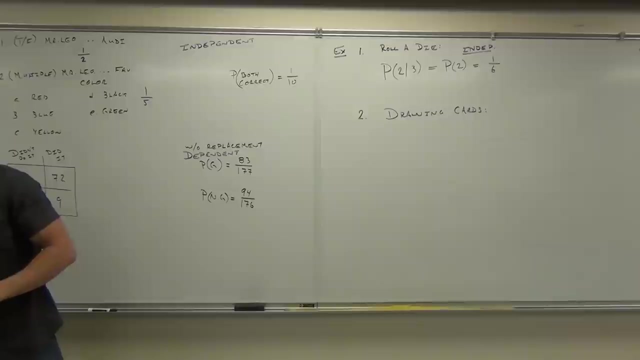 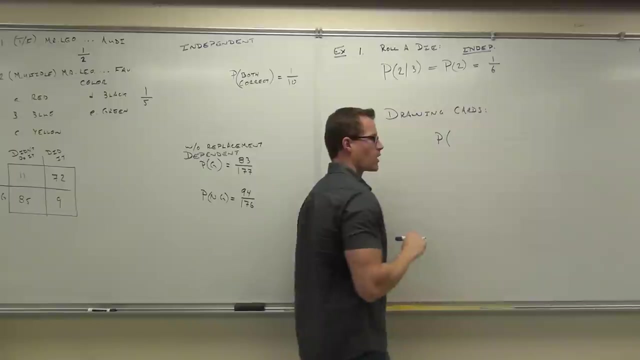 You have 1, 2 out of 6 possible choices. That's it. Now we're going to go to the standard deck of cards. again. We're going to draw some cards out, okay. What I want to find out? what's the probability of randomly selecting a queen in this case? 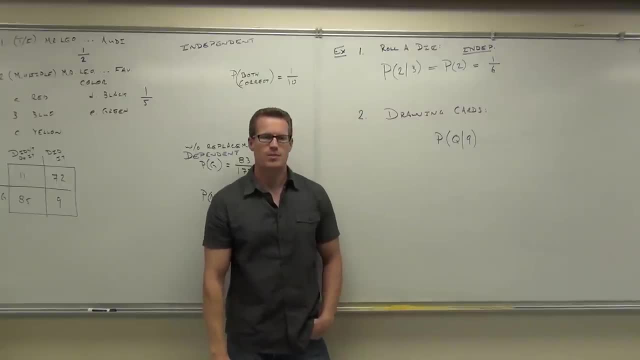 Hey again, which happened first? Did we select the queen first, or the 9 first, The 9.? So what this says is: what's the probability of randomly drawing out a queen? The 9., The 9., The 9.? 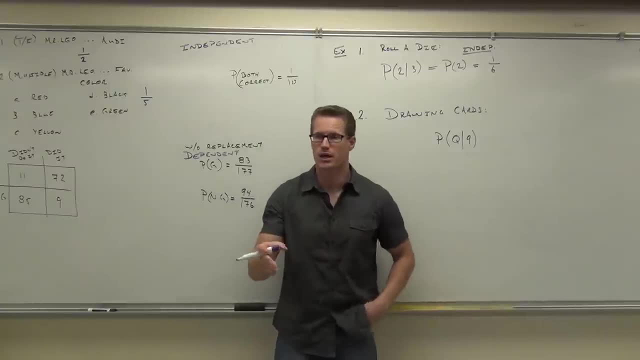 Given that you just drew out a 9.. So here's what happened. okay, I give you the deck of cards and I say you are going to select how many cards? One, One. You know the whole thing. you're going to select two cards. 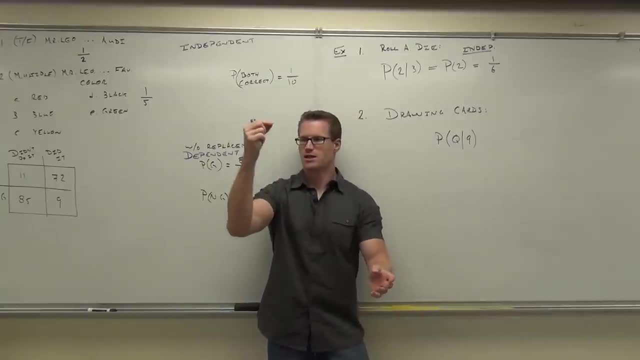 So I say, pick a card, any card, and you go, oh, here's a 9, and you put it in your pocket or you put it back in the deck And I said I reshuffle it and all that stuff and I now pick another card. 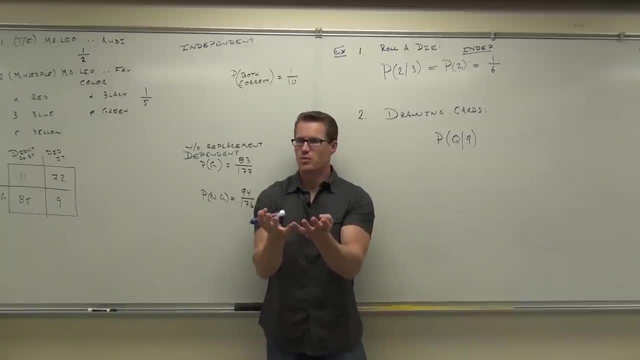 So you've had your 9, right? So now I'm asking: what's the probability of selecting the queen after you've found that you've selected that 9.. So you're drawing out two cards, The first one given that, given that the first one had to be a 9.. 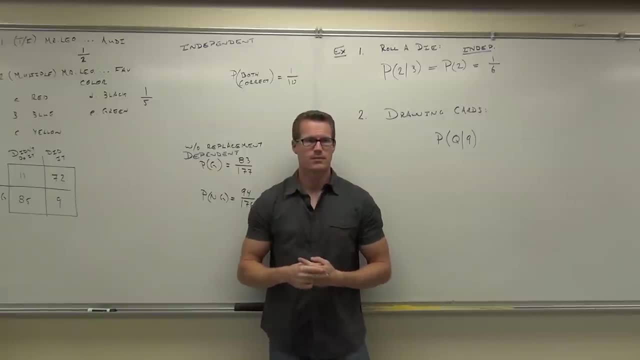 Now what's the probability of selecting that queen? Did you put it back in or did you keep it? Ah, there's the question. So do you see how that would make a difference If I put the 9 back in or I keep the 9 out? does that change my probability? 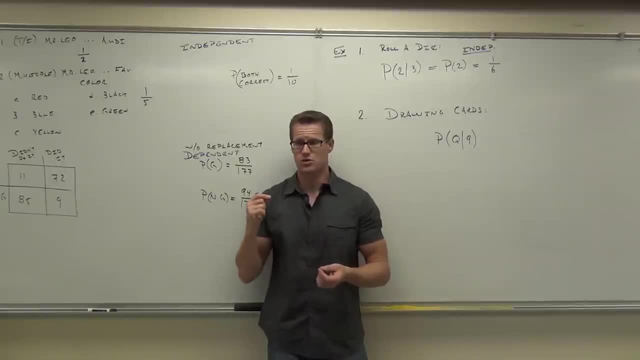 So in one case you're going to be dependent, In the other case you're going to be independent. Which one would be independent- putting back the card or keeping out the card? Well, I heard two different answers there. I heard keeping it back. 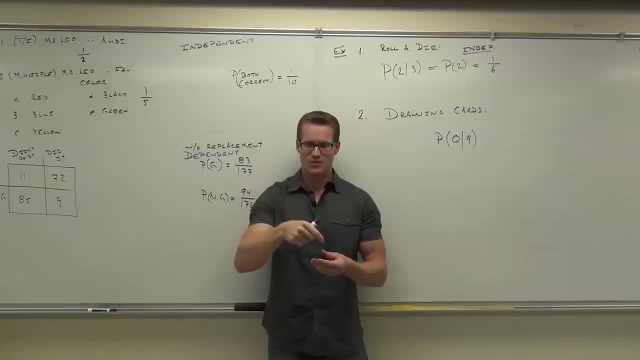 Okay, let's try this again. If you, what did I say? Did I say put it back in or keep it? Did I ask you for independent dependent? Okay, which one is independent: putting the card back in or keeping the card back out? 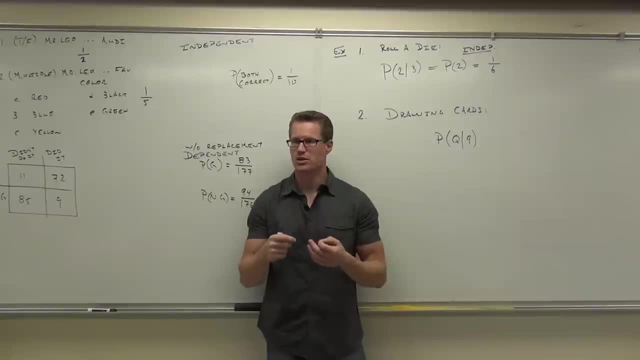 Here's what this translates, to, Which one is not going to change. the second probability: putting the card back in or keeping the card out. Keeping the card back in? Okay, let me ask this. okay, if it's not, if it's independent, doing this and doing this? 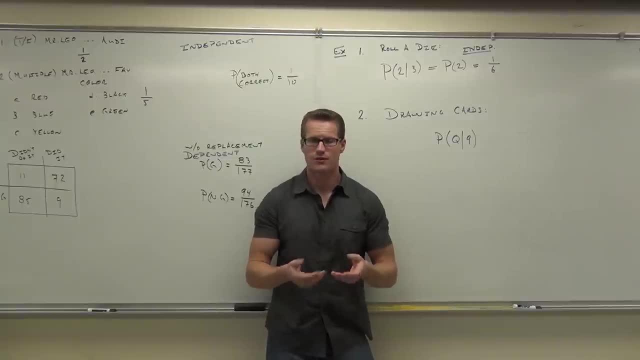 after this should make no difference. okay, that's what independent means. So if I just had a deck of cards and said, draw a card, what's the probability of getting a queen? Hopefully you're thinking four queens. 52 cards is 4 out of 52.. 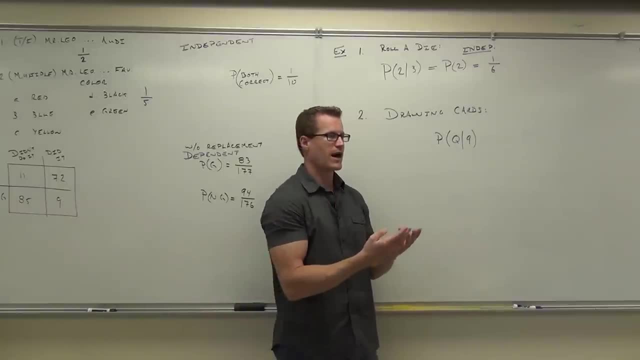 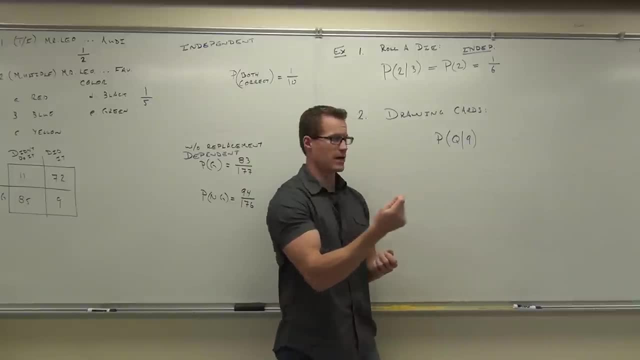 Yes, Yes, Yes, Yes, Yes. Then that's called independent. if you keep the 9 out, That's without replacement. okay, If I replace the 9, so you draw the 9, you put it back. What's the probability of drawing the queen out? 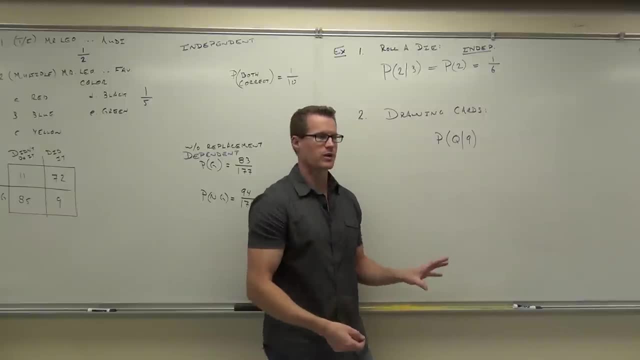 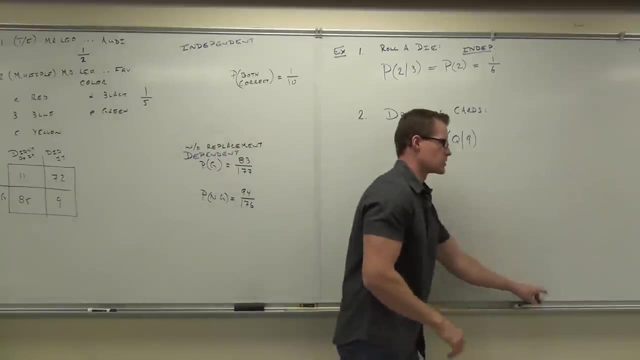 Well, there's still 52 cards now. right, You put the 9 back With replacement. if you always put the card back, you always get the same probabilities. That's independent. So I have to ask you two different questions here. 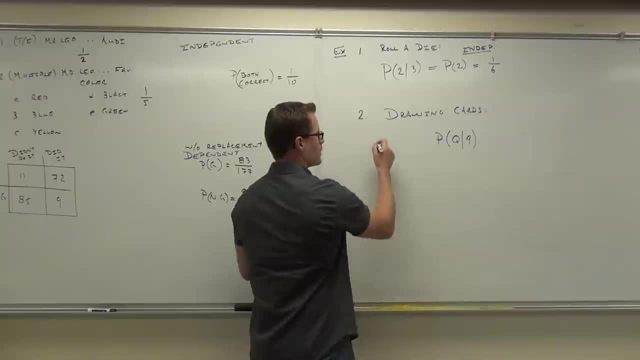 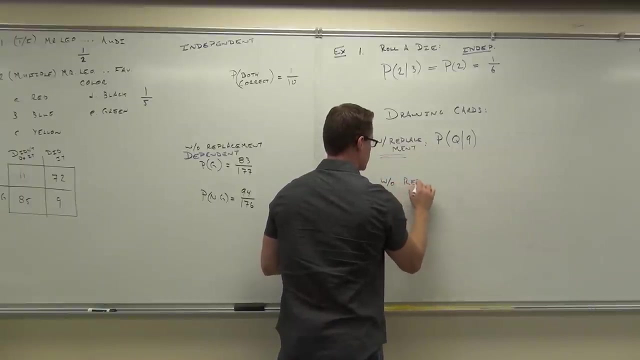 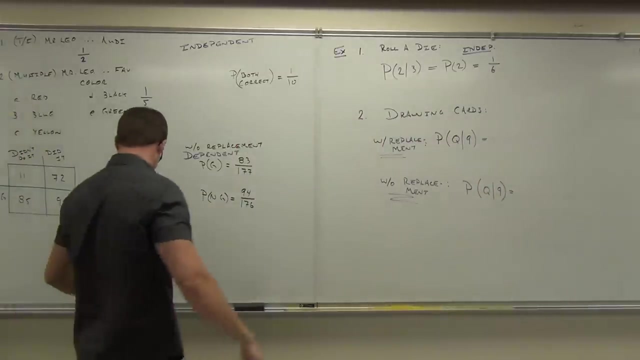 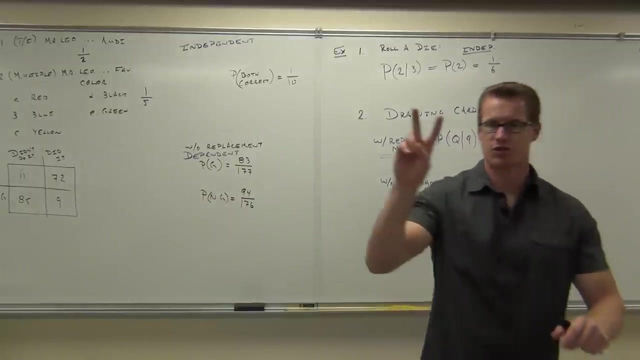 The first one is: let's say, we're doing this with replacement, Without replacement. Okay, with replacement. then what that means is: you draw out the nine. you've, of course, drawn the nine out, right. In either case, you're drawing the nine out. you're drawing two cards. 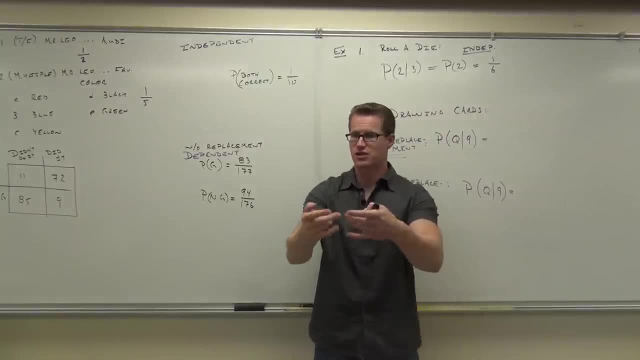 First one was a nine. I say with replacement. I say give me that card back. I put it back and I shuffle it up, right? Is that dependent or independent? again, Independent, Definitely independent, because you're going back to the same number of cards you started. 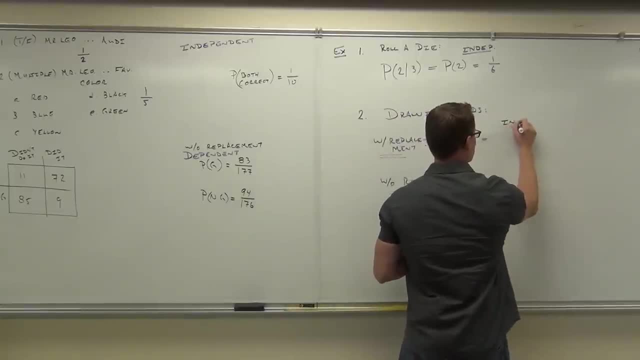 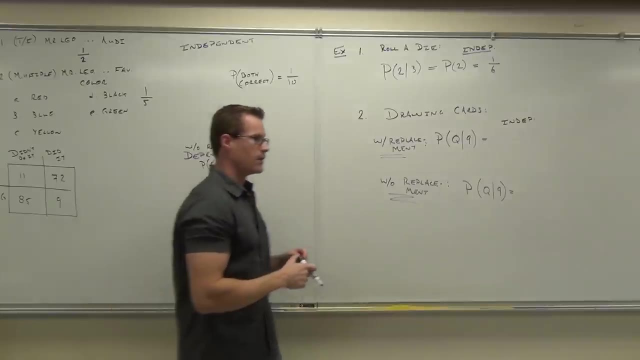 with. So this is for sure going to be independent. What's the probability P of three? All right, Okay. How many queens do you have? Four, How many cards do you have Fifty-two? Why fifty-two, not fifty-one? 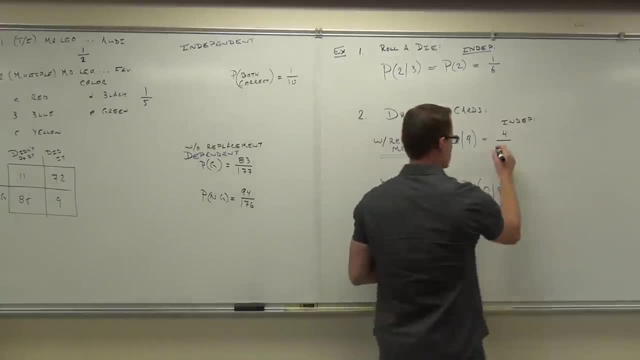 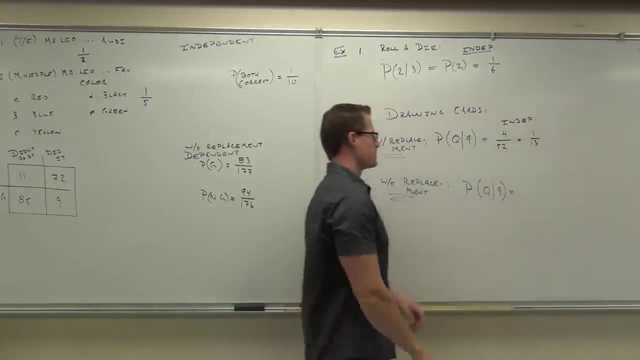 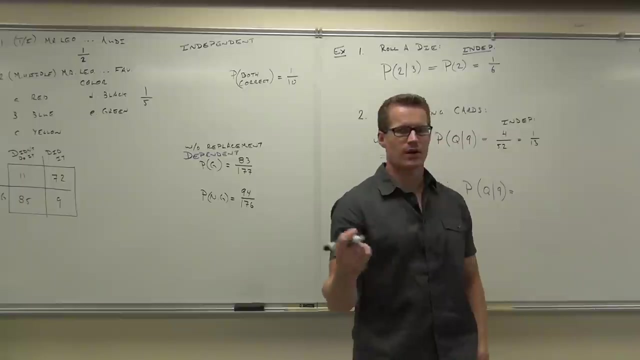 Because you only have fifty-six. That's very good. Fifty-two, that should be one-thirteenth Or some decimal. if you've got it, Let's talk about the with replacement. So again, you're drawing two cards, you draw one out, it's the nine. 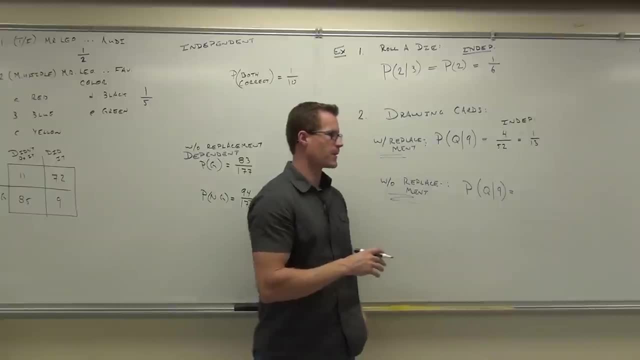 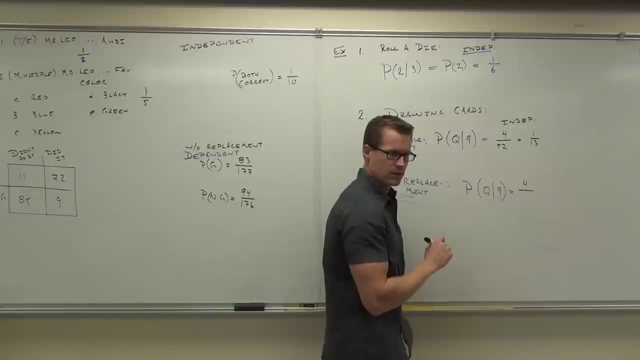 So, given that you drew the nine out, you put that nine in your pocket. how many queens are left? Four? How many cards are left Fifty-one? Why fifty-one? Because you have the nine in your pocket. So does selecting the nine affect the probability of selecting the queen? 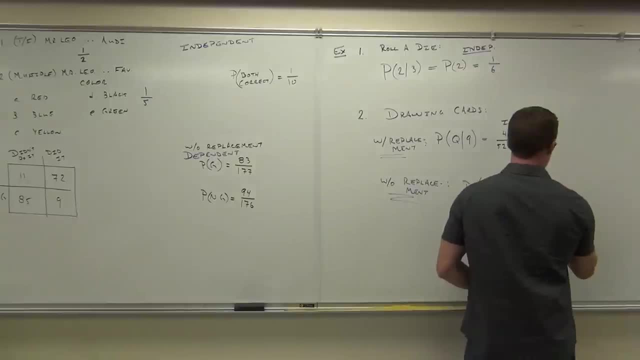 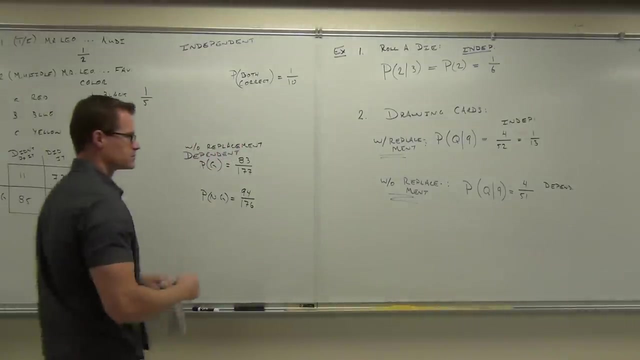 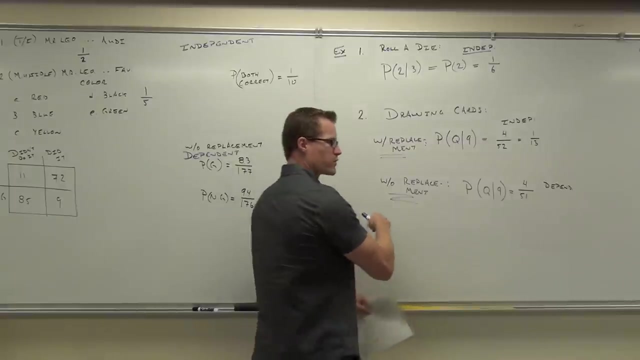 Definitely This is a dependent circumstance. Okay. Okay, Let's try one more. see if you really get the hang of this. Maybe two more. Let's do it on your own. Okay, Try one with replacement, one without replacement. 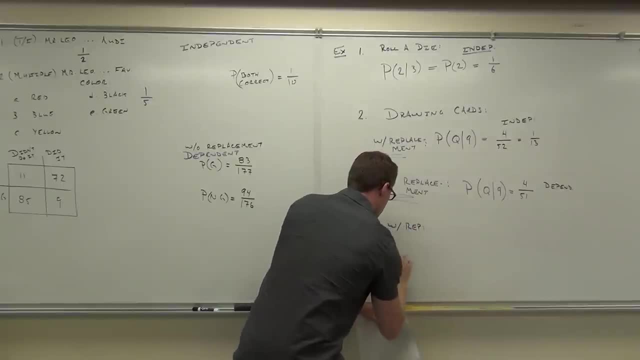 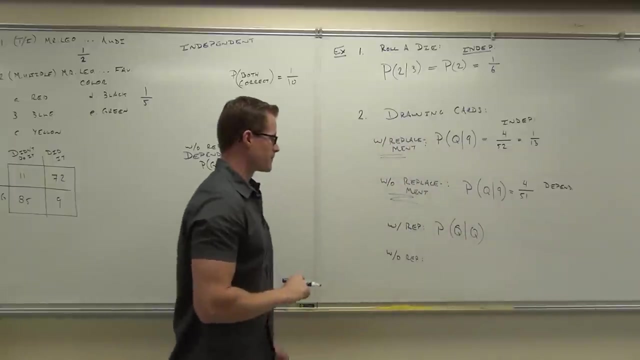 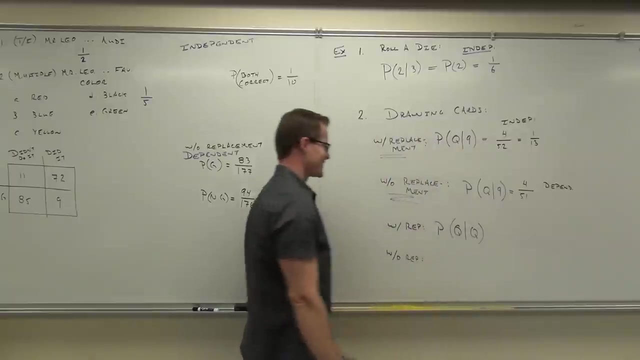 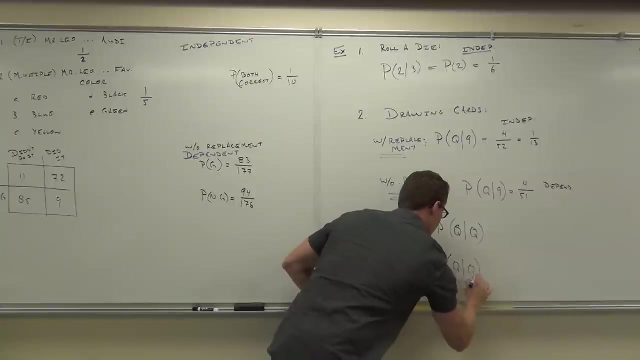 Let's say probability of selecting a queen. Let's see, Let's try it. Let's say probability of selecting a queen. Oh, look at you kind of. Look at your smiley face. I told you we'd have fun. 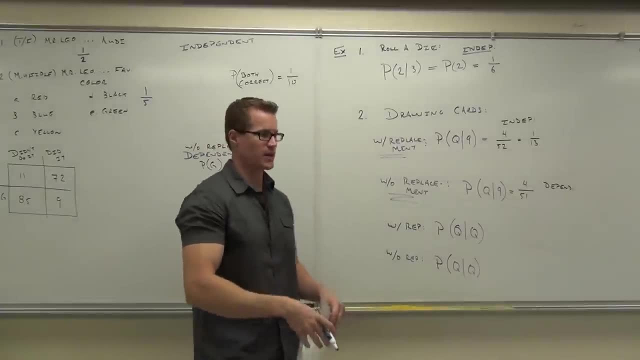 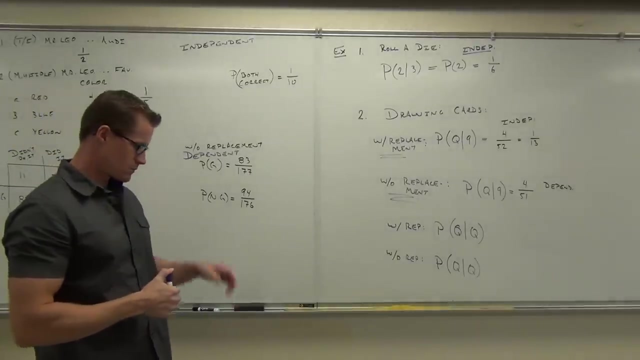 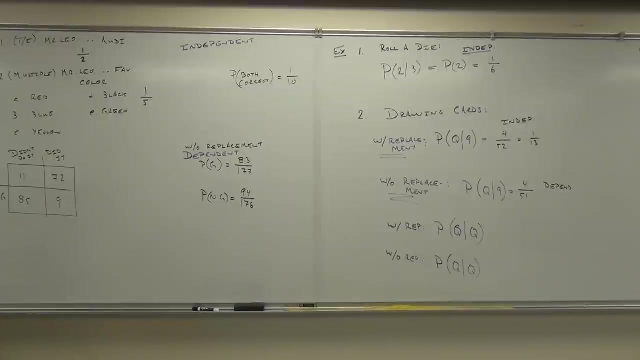 So these problems are going to look identical. You really have to know: with replacement, without replacement, Dependent, independent. You've got to know that. Figure this out, that, Figure those out. If you're done with that already, I'll give you one more kind. 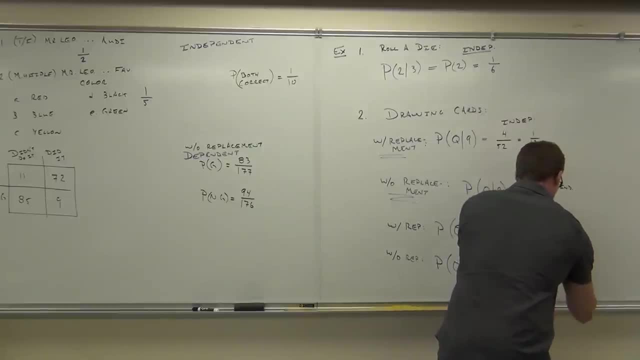 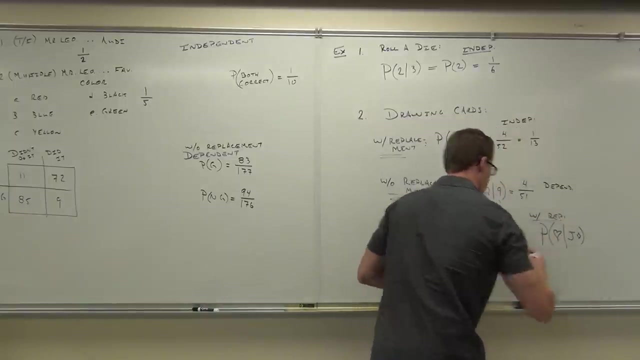 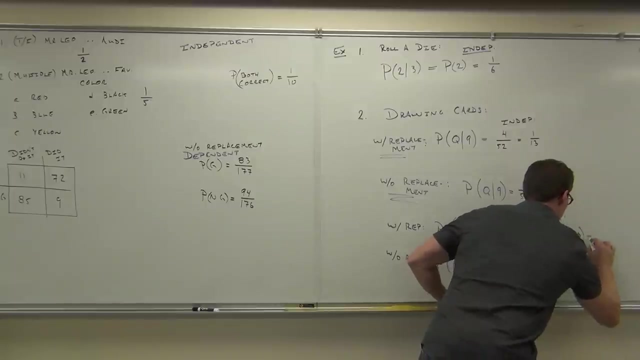 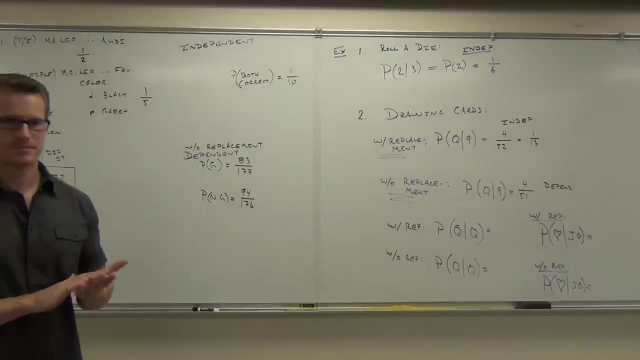 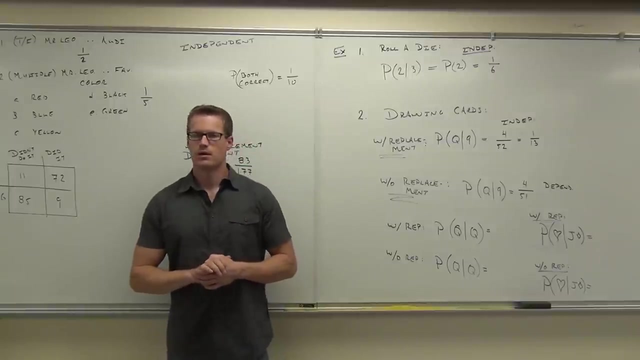 of challenge problem, That's Jack of Diamonds. Are we doing that one with three places? No, without. Do it both, Do it with and without 13.. That's 13 of every suit, four cards, four of every specific card. One card, one number. 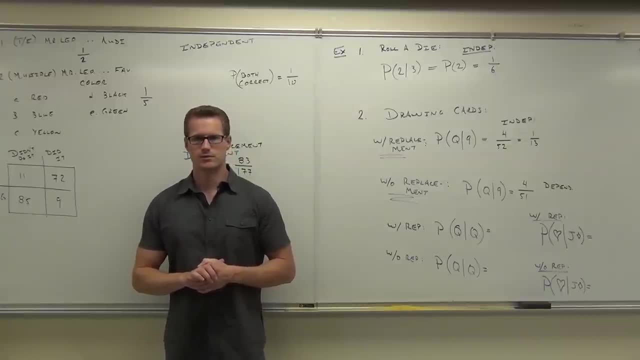 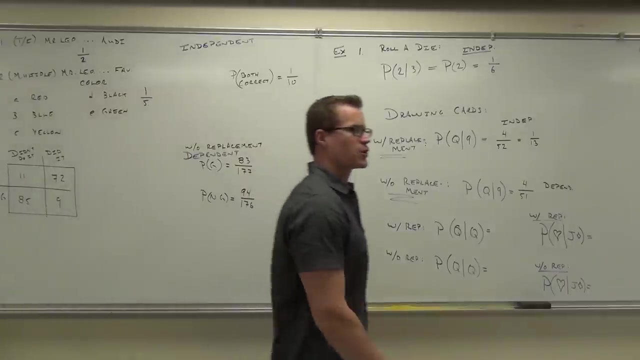 per card per suit. So like there's only one, Jack of Diamonds, Bless you. Oh, here's some homework to pass back. Make sure this goes around quickly. All right, let's discover what we got out of this thing. So, with replacement, you're. 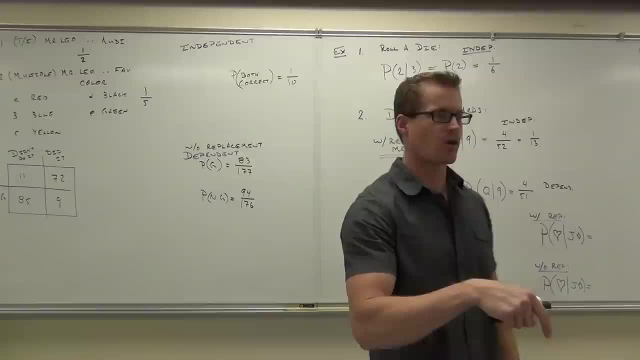 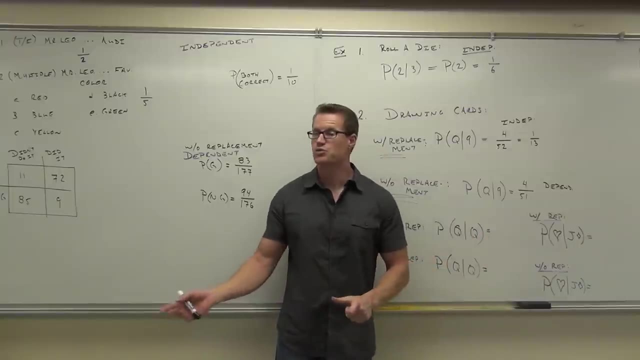 going to notice that with replacement doesn't affect your probability. So if you're always putting the card back, this second part is, honestly, it's irrelevant, right? If you're always putting the card back, it doesn't change anything. So with independent events, if it's. with replacement, it doesn't affect your probability. So if you're always putting the card back, this second part is obviously. it's irrelevant, right? It's always putting the card back. you're going to notice that with replacement it doesn't matter. So what's the probability? 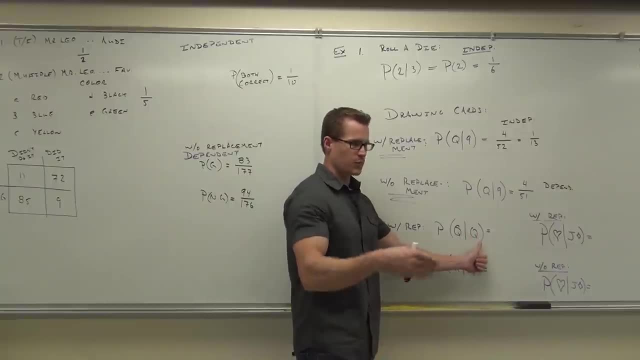 you've selected a Queen. given that you've selected a Queen, if you've replaced the Queen, Good, Yeah, there's still four Queens because you put the Queen back. There's still 52 cards because you put the card back. Did you get that? Good, Let's try this one. What's? 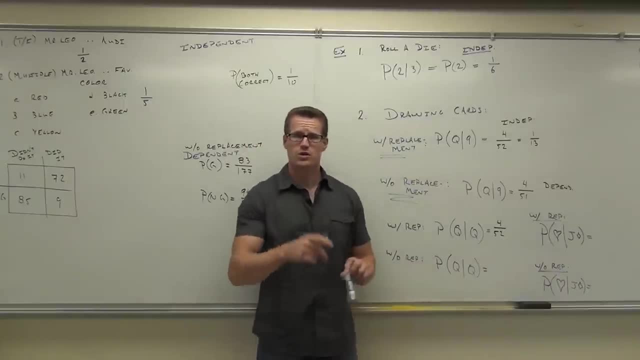 the probability of selecting a Queen, given you've selected a Queen without replacement. So you selected one card and it was a Queen. you put it away. I say: what's the probability you're going to get your next Queen? Why three? 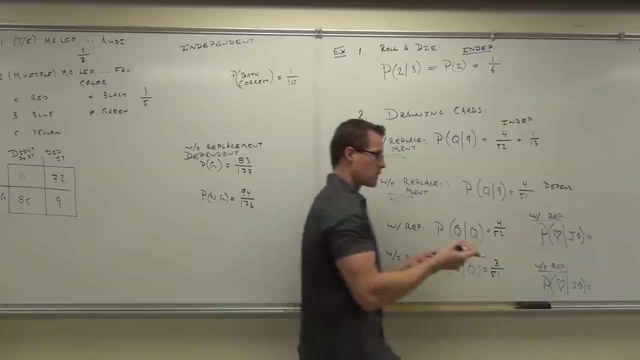 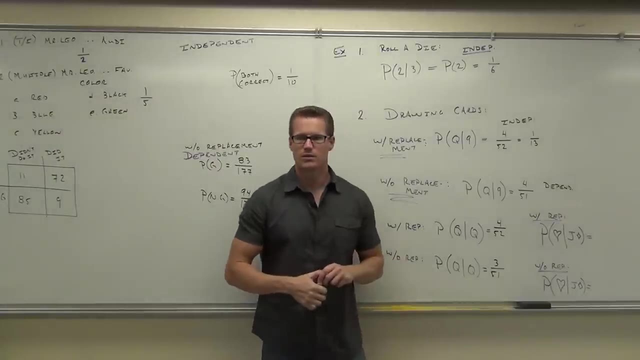 Ah, you kept that queen out 51, you kept the card out. Good job, you got that one right. That's great, that's fantastic. Hey, could I keep going? Could I say, find the probability of selecting a queen? 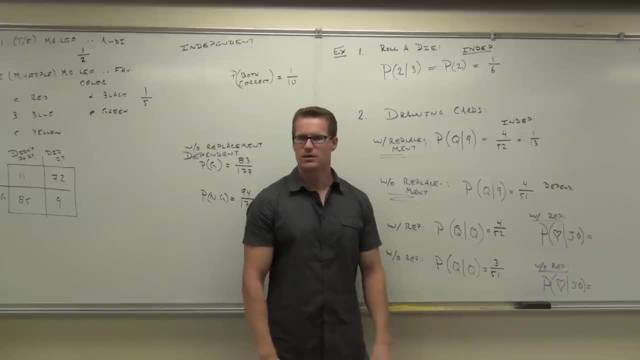 after selecting a queen, after selecting a queen, after selecting a queen, It'd be only one out of 50, whatever you do, You'd count that down. This concept can be extended. How about the probability, oh, of selecting a heart? 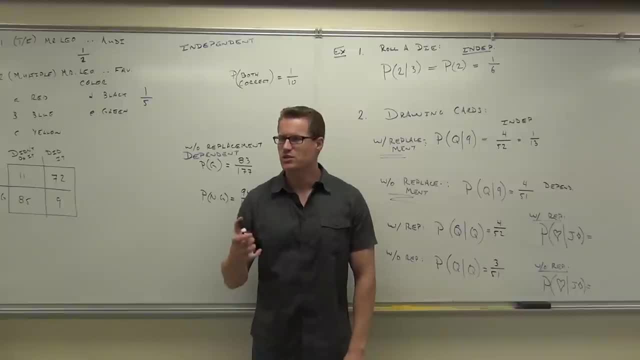 given you selected a jack of diamonds, I can't ask you what's the probability of selecting a heart, given you selected a jack. Because a jack you don't know, Was it a heart, was it a diamond, was it a club, was it a spade? 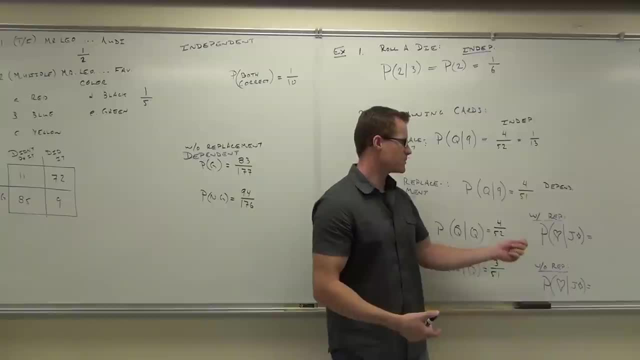 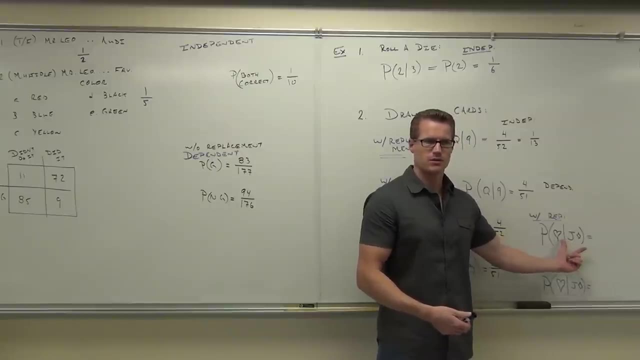 So I had to tell you a specific suit. So, with replacement, what's the probability of selecting a heart, given you've already selected a jack of diamonds? with replacement 52, you've replaced that card. Good, there's 13 hearts. 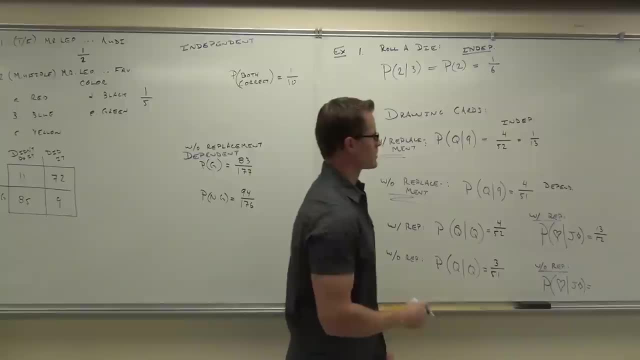 Out of 52 cards because we put that jack back. Now, let's say we don't put the jack back without replacement Probability of selecting a heart. given you selected a jack of diamonds, jack of diamonds, Why 13?? 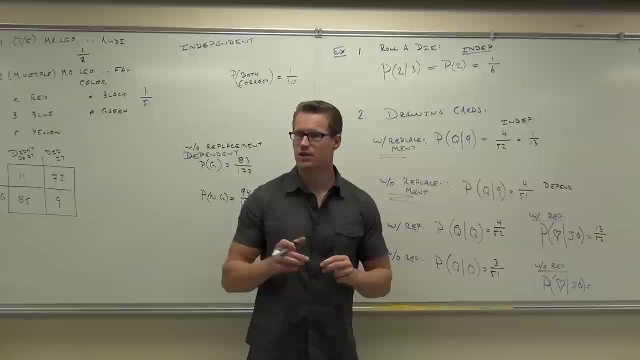 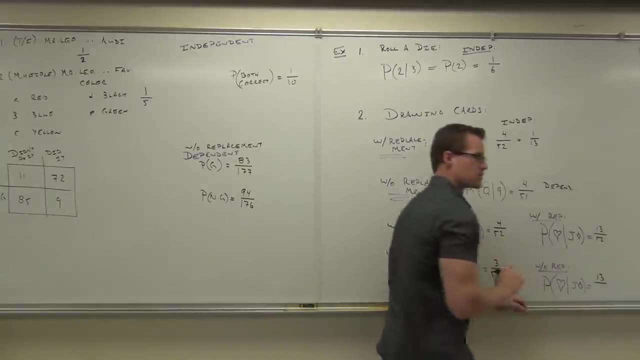 There's still 13 hearts. We took out a jack of diamonds, right, So we didn't touch the hearts. There's still 13 of them. How many cards? 51. Could you do this If I said that was a jack of hearts? 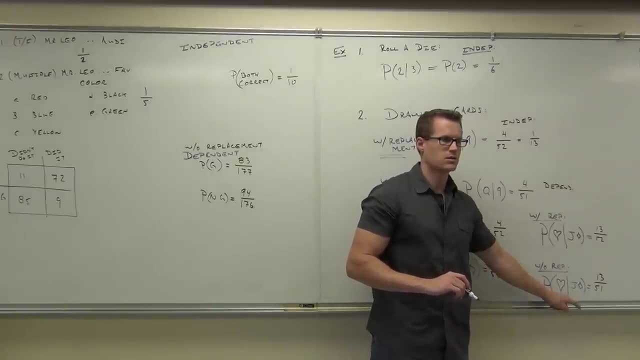 No, Why not Taking a heart away? it would change the probability. It would change the probability. sure, If that was a jack of hearts you would have 12. Over 51. That's right. So probability stuff, as long as you're keeping. 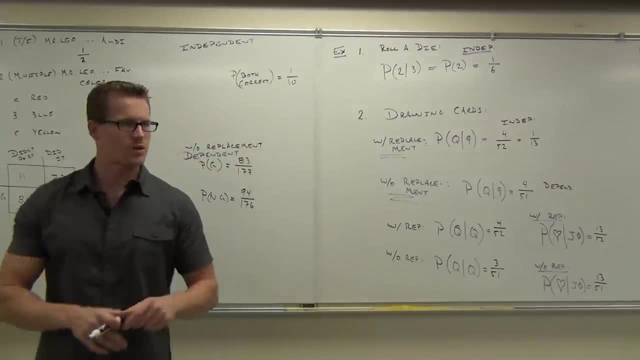 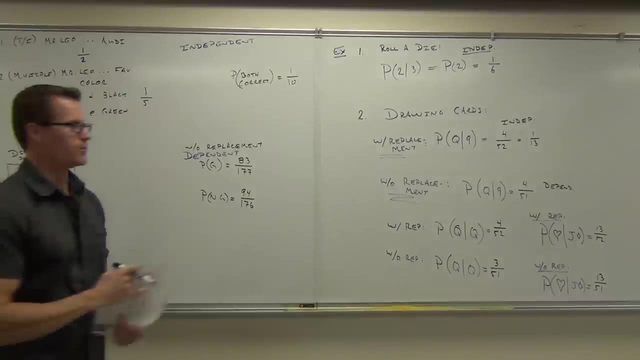 with the dependent independent. you know what replacement without replacement is. you should be okay with this. How many people feel right with what we talked about so far today? Good, good, good, We're ready. we're ready for the multiplication rule. 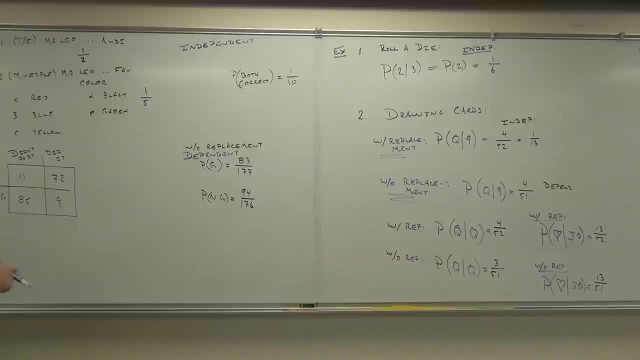 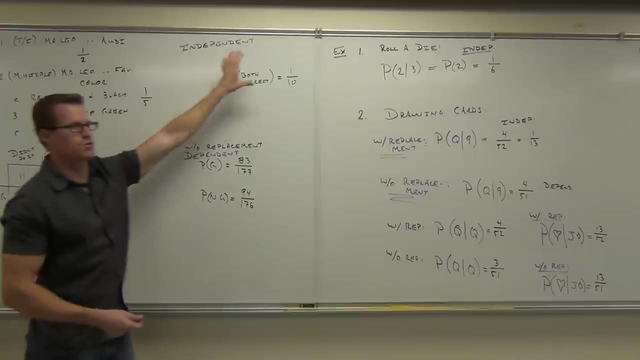 Now, when we're going back over this, here's where we're gonna start. When we look at this thing, can you tell me, is there a way to get from 1 half and 1 fifth to 1 tenth? Have you seen that? 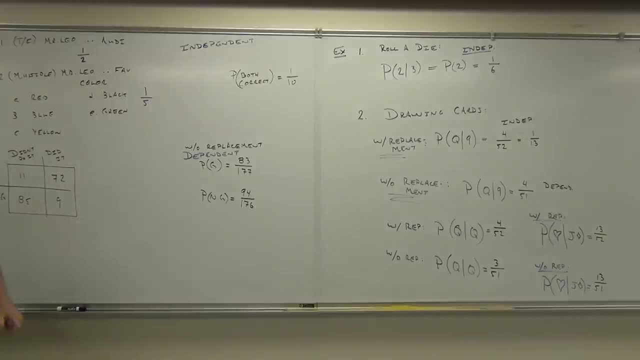 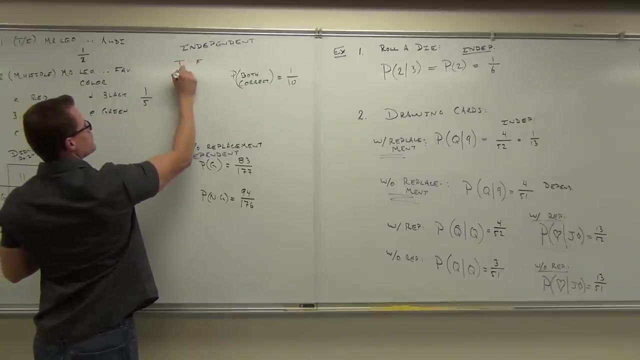 Sure, Here's what we did when I drew that diagram for you, Honestly, The purple one. When I drew the diagram, I drew true, false, and I had 1,, 2,, 3, 4, 5 options: 1,, 2,, 3,, 4, 5 options. 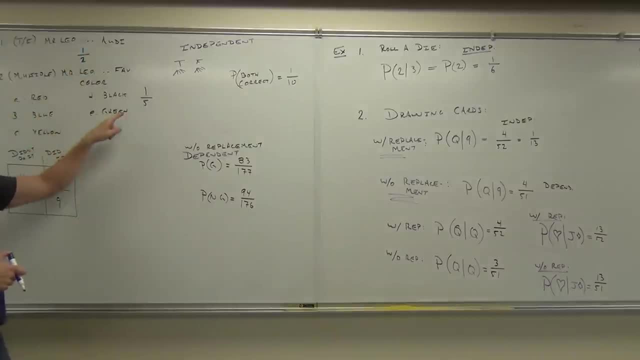 So for every choice I had here I had this many choices. So for a true I had 5 choices, For a false I had 5 choices. So essentially what we did is we said I've got 2 choices for the first one. 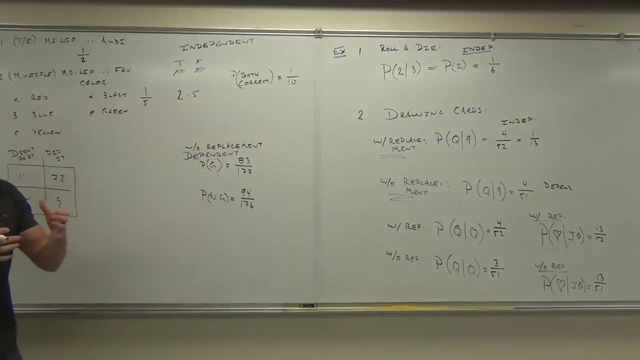 I've got 5 choices for the second one. Combined with each other, that gives me 10 total choices to choose from out of my problems. right, We said we could do true A, true B, true C, true, and so on. 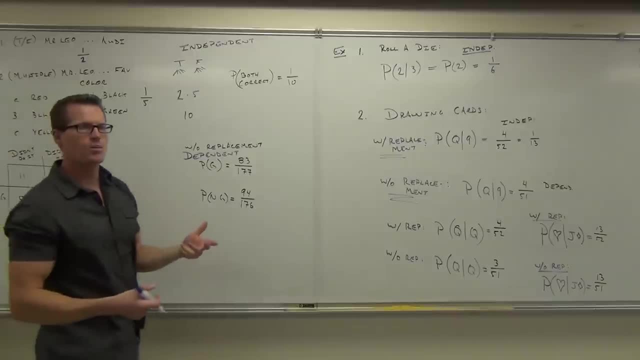 And we could do false A, false B and so on. That gave me 10 choices. How many of them was the right choice? Only one of them. That gave me a probability of 1 out of 10.. If we think about it differently, we go OK. 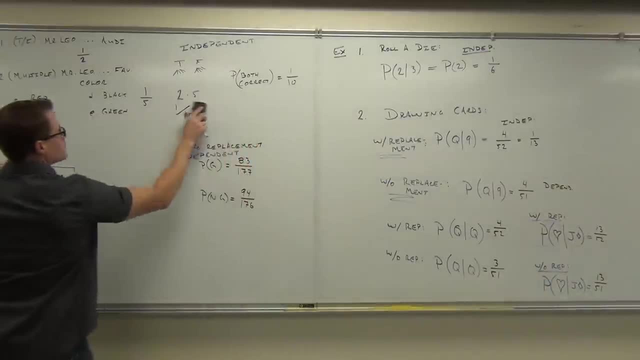 Well, I can do the same thing with the probabilities themselves. If I look at this probability and this probability, we'll notice that the 1 tenth is simply the 1 half times the 1 fifth. That's how we do this. That's the multiplication rule. 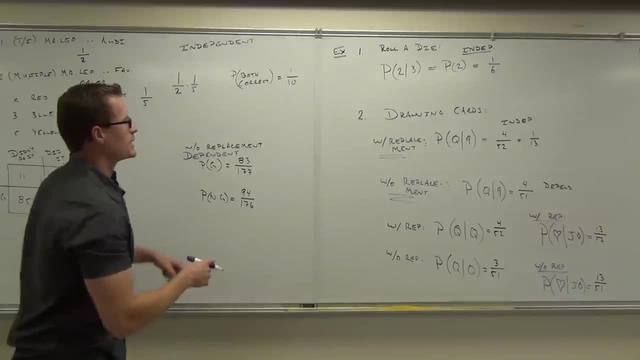 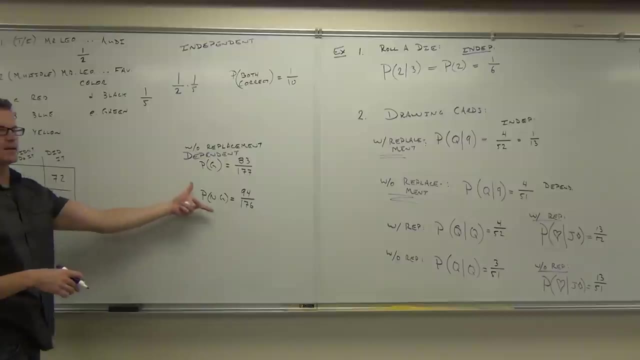 It says: if you have an and probability, what's the probability of, What's the probability of getting both of these right, This one and this one? What's the probability of selecting a guilty and a not guilty, Multiplying our probabilities? And that's going to lead us to the multiplication rule, right? 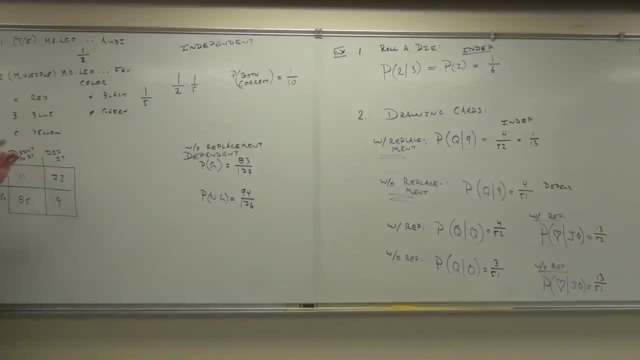 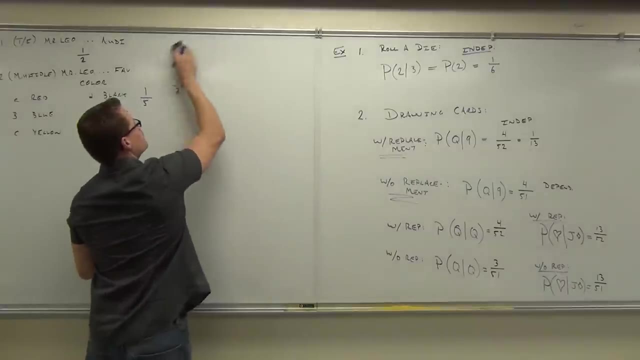 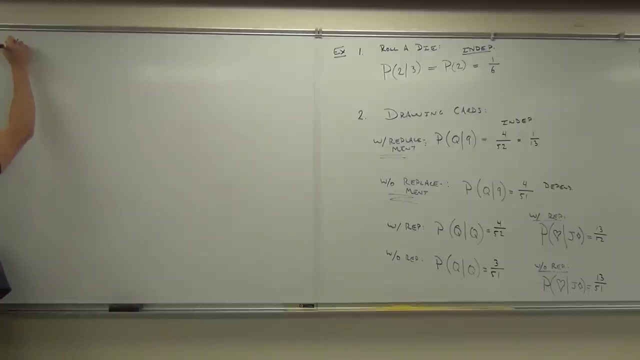 now. Are there any questions on this? before I erase that, We'll move back over here. So the multiplication rule says: I want you to find the probability of A and B. By the way, A and B, this and is this in a single trial? 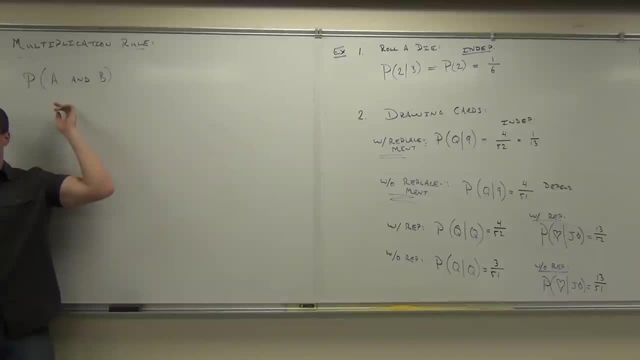 or in successive trials. What is that? Success, Success, Success, Success. In this context, this is in successive trials. The single would be at the back end of the probability. So what this means is A and then A and then B. That means successive trials. 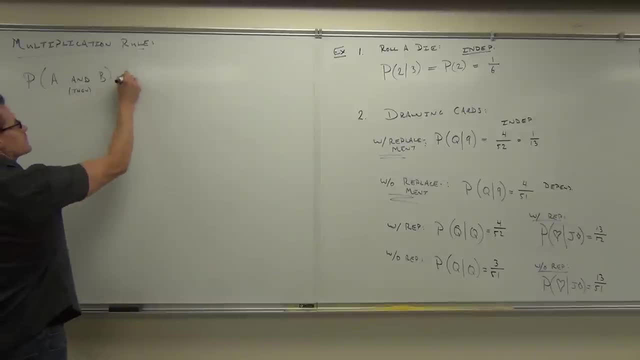 A and then B. Well, here it is. In order to find the probability of an and problem, so probability of A and then B, we do take the first probability: A happens first. Probability of A. So in our question up here, 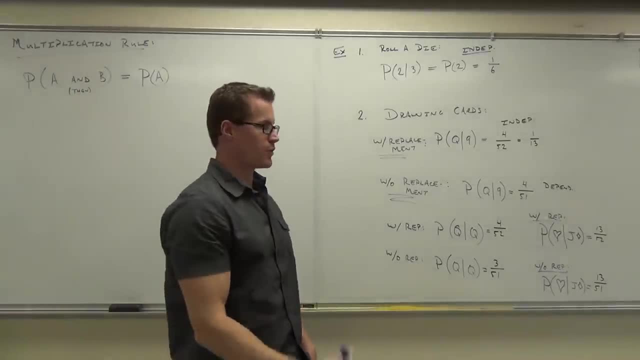 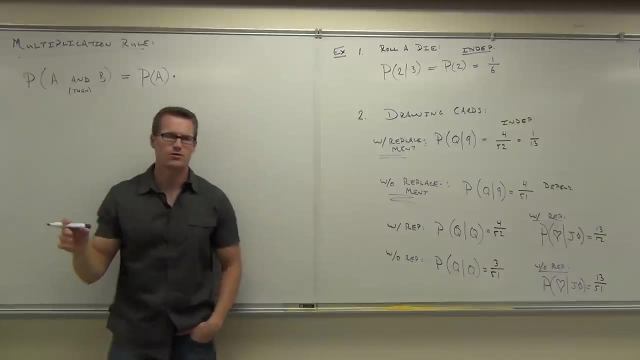 that we had before the Audi question. we have one half. That would be our first probability times how many choices you have for the second probability. So really all you're doing here, folks, you're taking the number of choices you had for the first event and multiplying it. 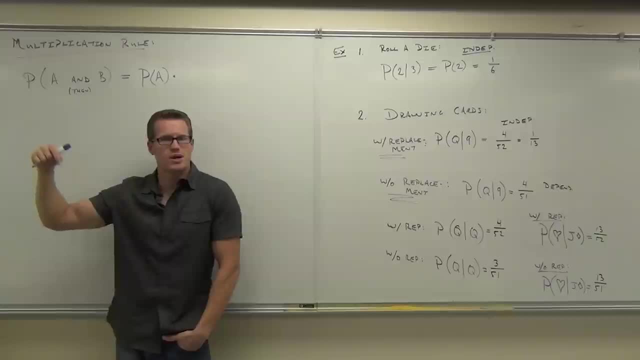 by the number of choices you have for the second, Because for each choice you have on the first event you have that many choices for the second event: The true A, true B, true C, false A, false B, false C. 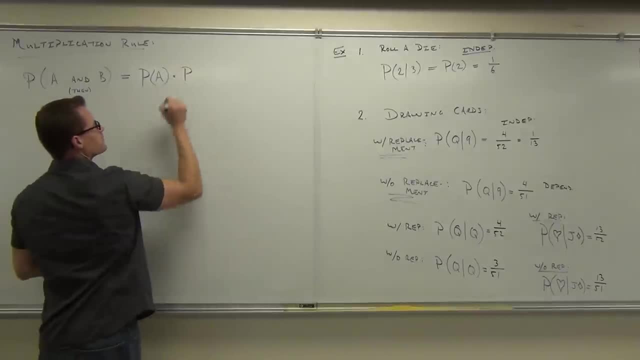 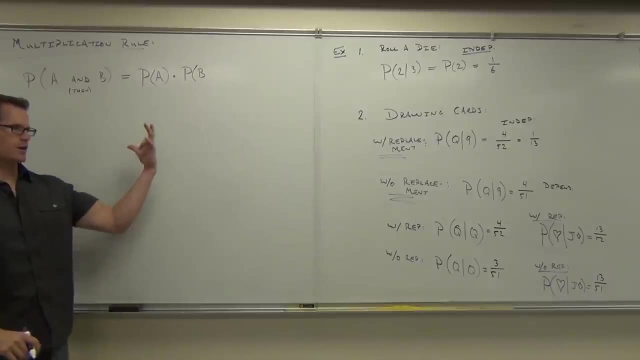 So that's a multiplication problem. So we are multiplying. Okay, So we're going to multiply. Multiply by event B. There's only one more thing you have to take on there. You notice I'm missing the parentheses here, And here's why. 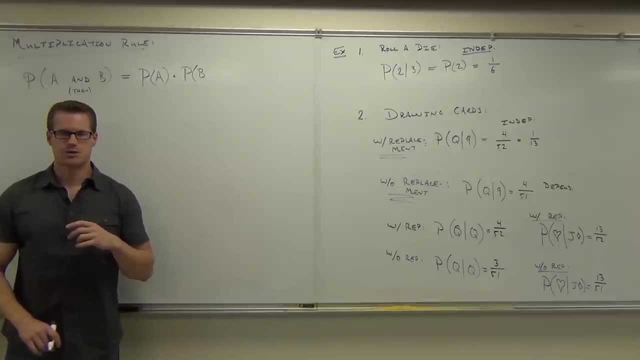 Here's why. Watch on the board here very carefully, please. I'm going to show you something. This works if your events are independent, like they are for the dice, like they were for our first two questions. Because A does not affect B, You take the total outcome here. 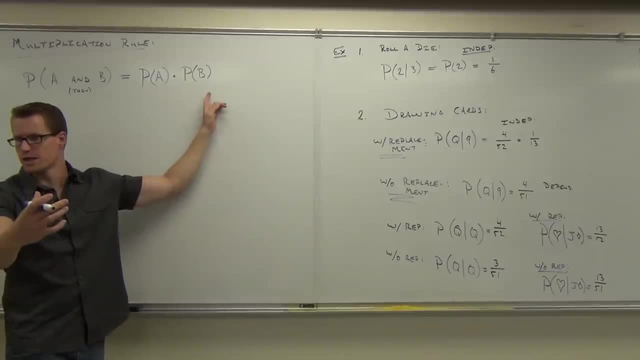 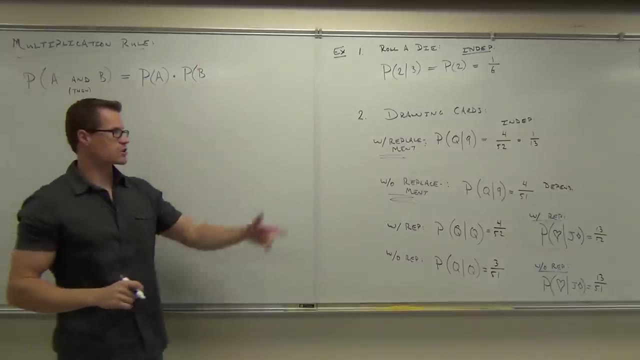 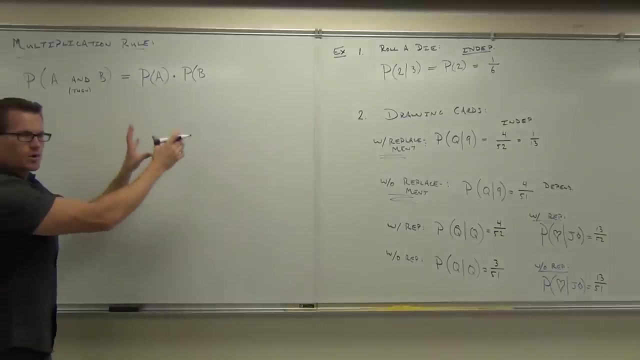 multiply by the total outcome, You get the total for both of them together in the n probability. However, is it possible that A can affect event B? Yeah, we just saw that right here. Without replacement, it affects it. So we have to say not only is it probability of A times, 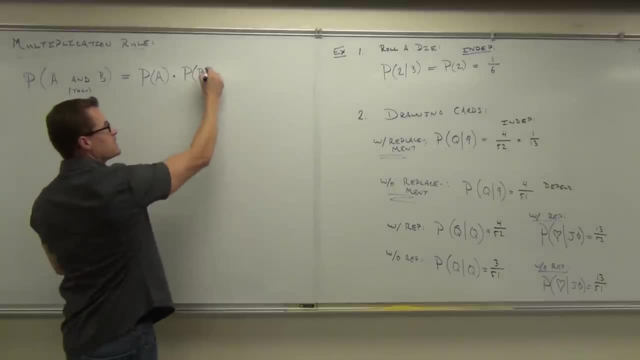 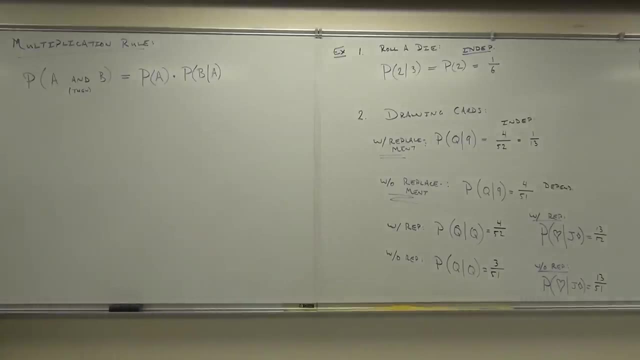 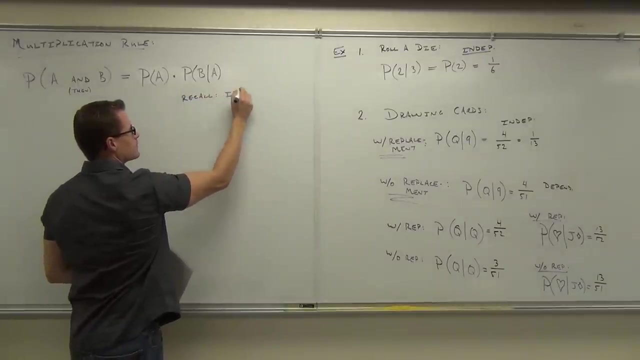 probability of B. it's probability of A times the probability of B, given that A has just happened. But remember, if these two things are independent, what's this equal to Probability of A? So that, yeah, But remember, if independent probability of B, given A equals. 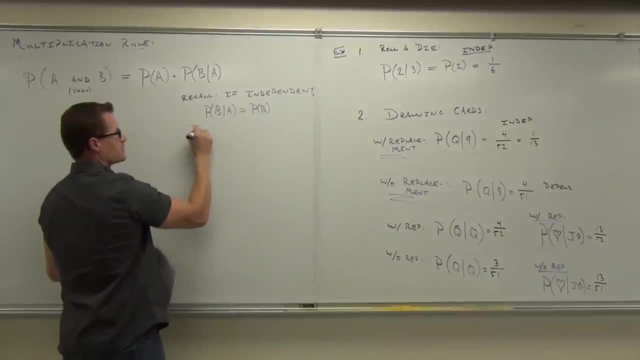 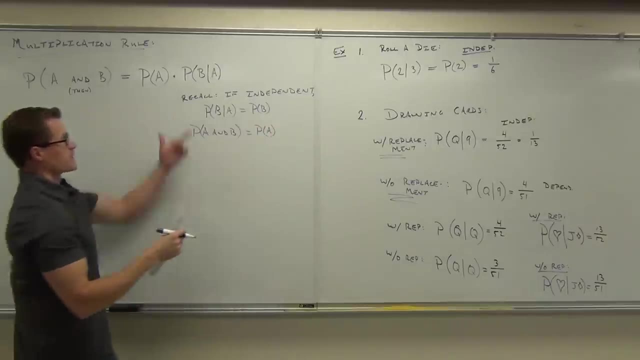 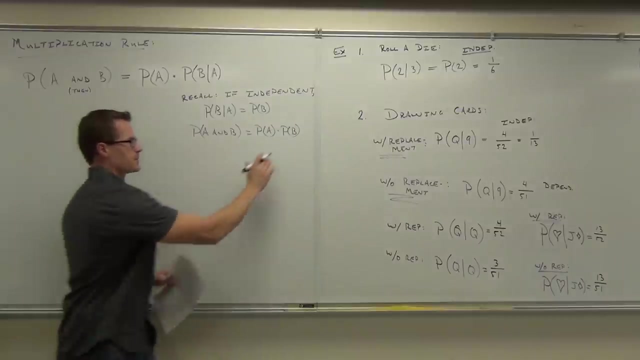 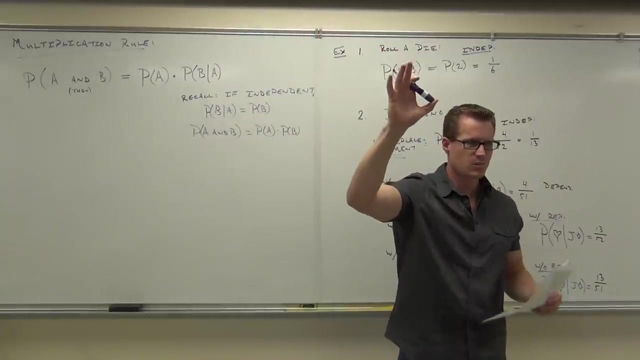 the probability of B. So then this probability would simply equal the probability of A times well, here it would be the probability of B. I need you to check that on the board and raise your hand if that makes sense to you why we're getting two similar things here. 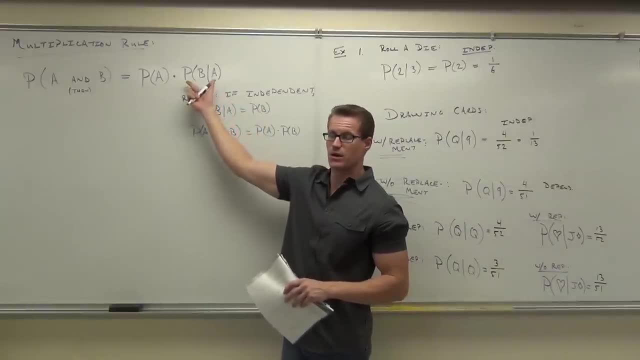 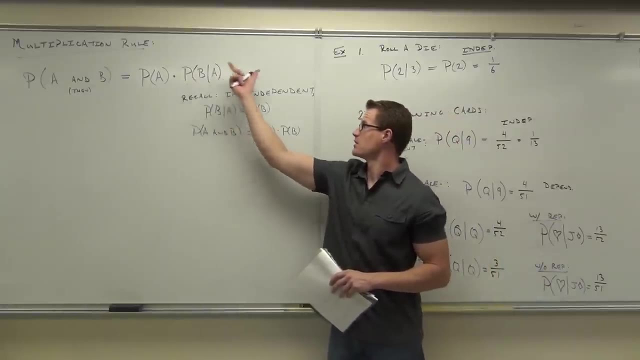 Why we have this one. if they're dependent, well, A's going to affect B And independent, well, B doesn't affect B, And we know that if they're independent, this is the same as this. I usually just stick to this one, because you're never going to screw that one up. 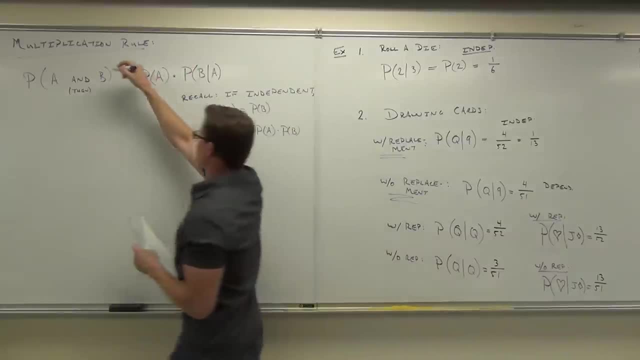 If they're independent, it really doesn't make a difference, right? So we're going to- really we're going to- use this formula all the time. I just want you to notice that if this is independent, you just stick with the probability. 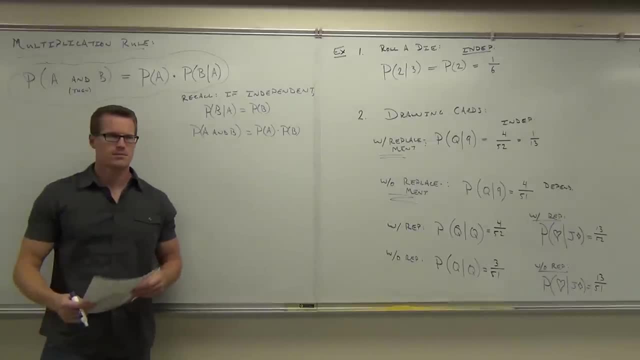 of B. That's why I have that on the board. Are you clear on that one, Yes or no? We're having fun yet. Yeah, Just lie. Yes, This is awesome. I love this stuff. Hopefully you do. hopefully you're having fun. 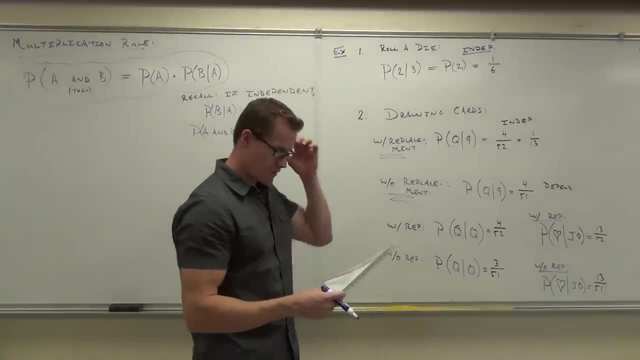 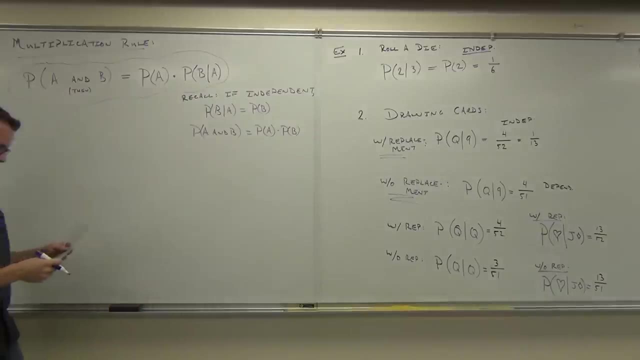 Would you like to try a few examples to kind of flesh this thing out in the last ten minutes or so? Yes, The answer to that question is always yes, That's right. Of course you would. We've got a bag of marbles. 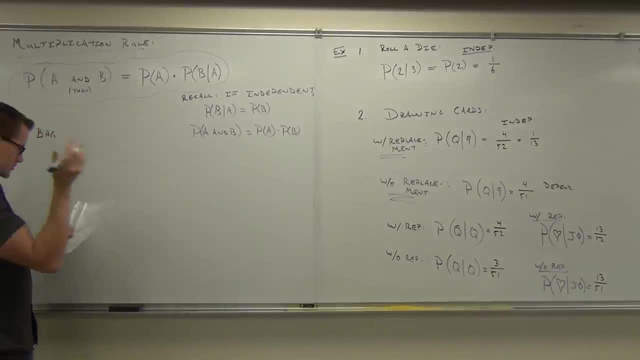 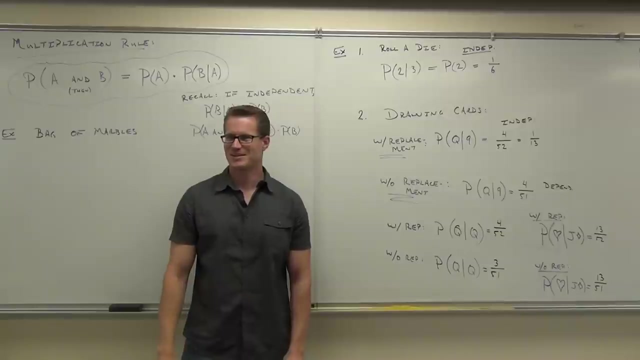 Some of you probably think I've lost my marbles. Have you heard that expression before? Yeah, Okay, good, Good. I think I'm getting older because some of my expressions like pinched pennies, you're like lost his marbles. 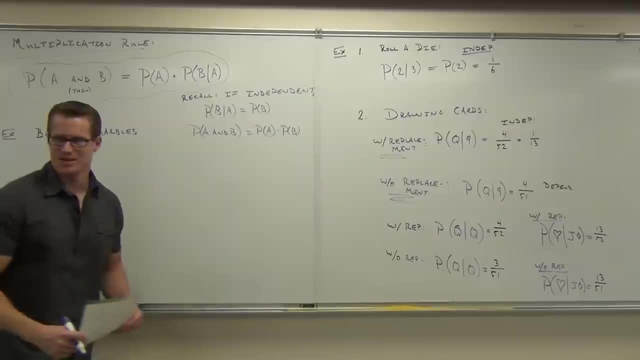 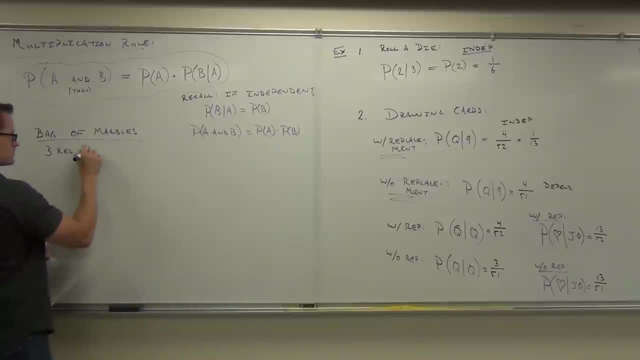 Three red, Three red, Two blue, Two blue, Four green. What we're going to do is find the probability of selecting green and blue. We're going to do this one with replacement: Two blue, Two blue, Two green, Two blue. 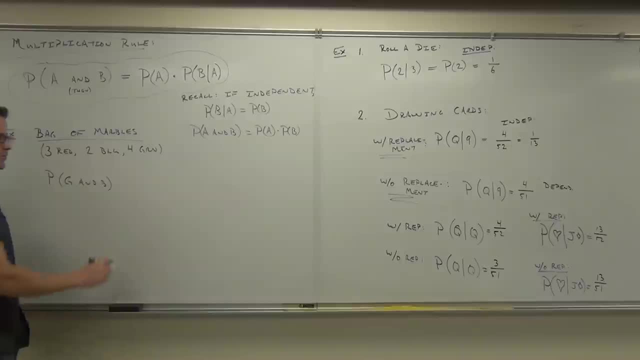 Two green, Two blue, Two green. What? Two green, Two green. You're going to do the same one without replacement. After that, I'm going to have you try a couple on your own. I'm going to find the probability of a red and red with out replacement. 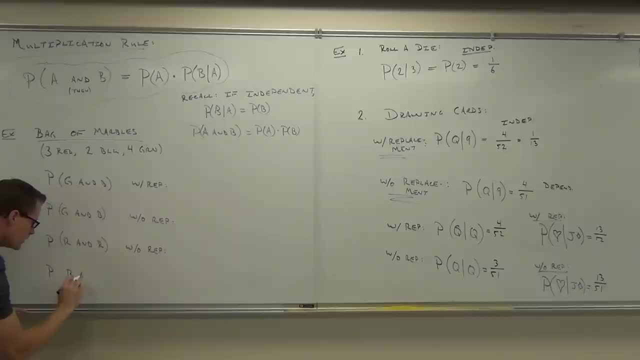 And then I want you to find the probability of a blue and blue and blue without replacement. So that's our goal for today, for the rest of our day, to figure out that stuff. Maybe we'll talk about a couple more later on. 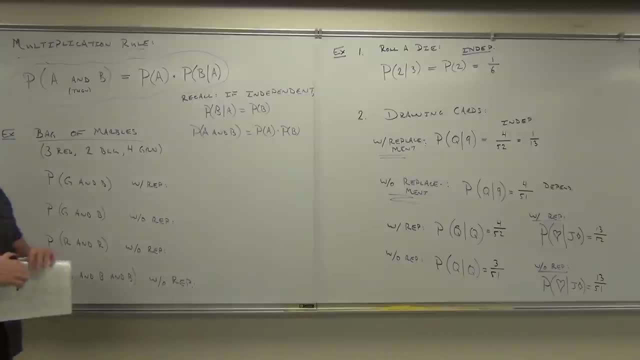 Okay, probability of green and blue with replacement. With replacement means you draw the marble out, you put the marble back, then you draw again. So with replacement, what's the probability of selecting a green marble, please? Four and a nine. 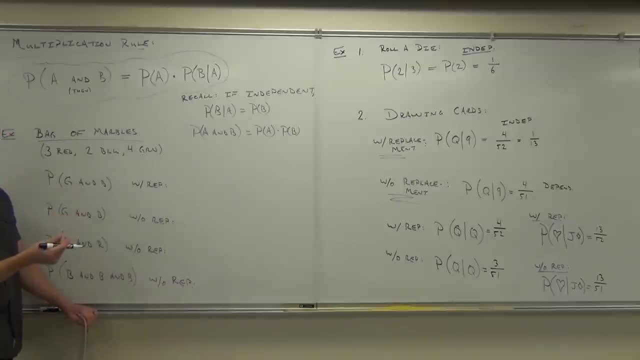 What now? Four and a nine? Why nine? Okay, great. So what we're looking for is the probability of a green marble. What's the probability of green times the probability of blue, given you picked out a green one? Here's how you write this out in math speak. 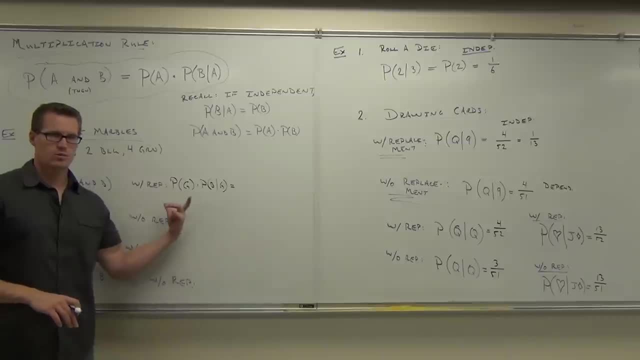 You just need to write the same thing all these times and be able to determine with replacement or without replacement. That's pretty much it right. That's why we stick to this formula. We don't have to get confused between these two. It's just one. 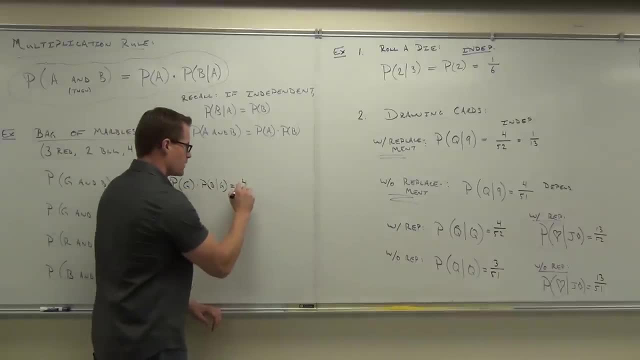 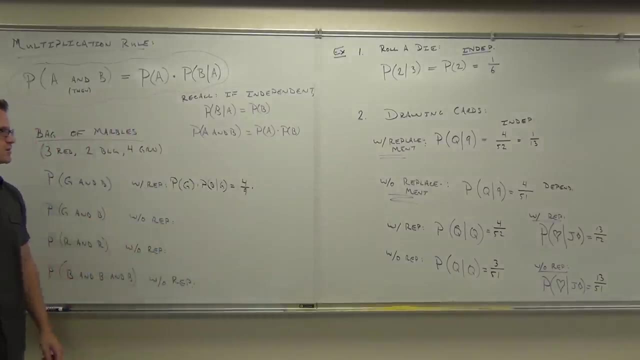 It's just one formula, So what's the probability of selecting a green? You said four out of nine times. What's the probability of selecting a blue marble, given you selected it out- A green marble first? You okay with the green marble? 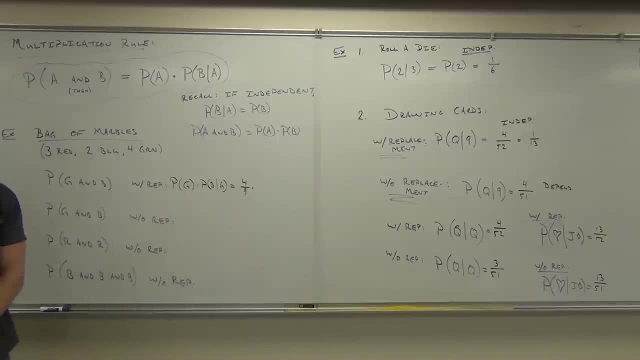 Four out of nine. What's the probability of selecting a blue marble now, given you just pulled out the green one? Four out of nine. Why out of nine? Because it's with replacement? Sure it is, It's with replacement. So there's still two blue marbles. 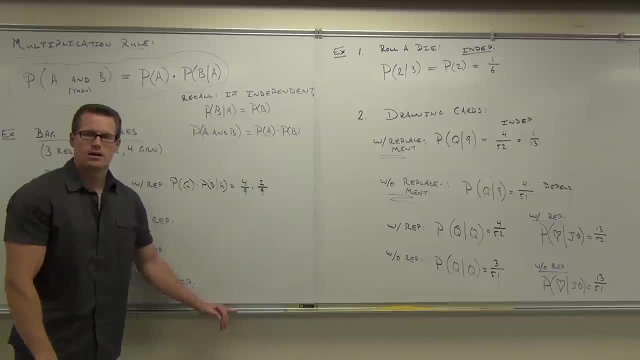 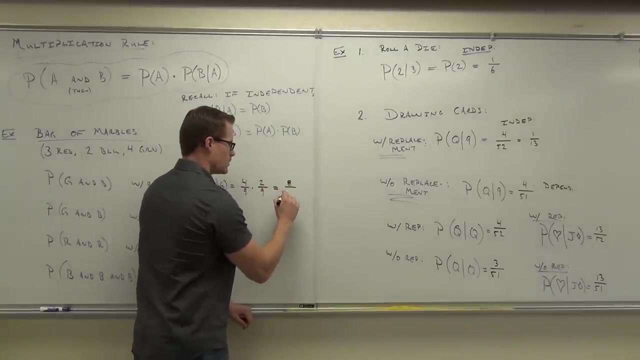 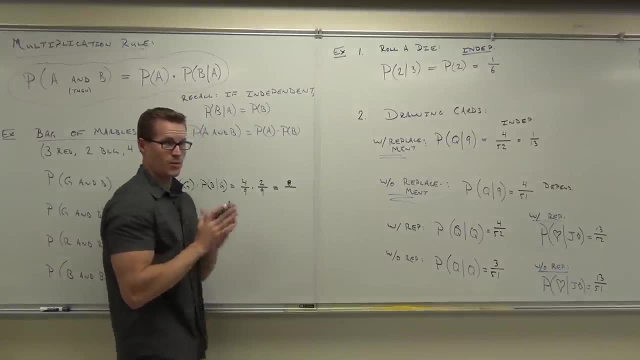 One. Let's multiply fractions. We do know how to multiply fractions. Please, Nine, Nine, Nine, Nine, Nine, Nine. Let's try this question. Do the eights cancel? No, They don't. They don't. 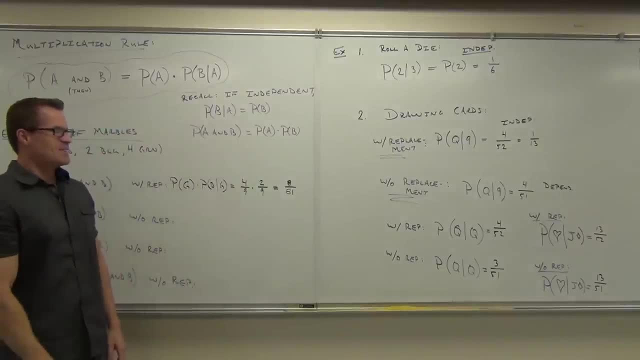 They're not. What do you do? We have to do this right. We multiply the octaves. These are not octaves. We do say it's not eighty, We do. I'm saying, Mr, I graduated in Calculus. 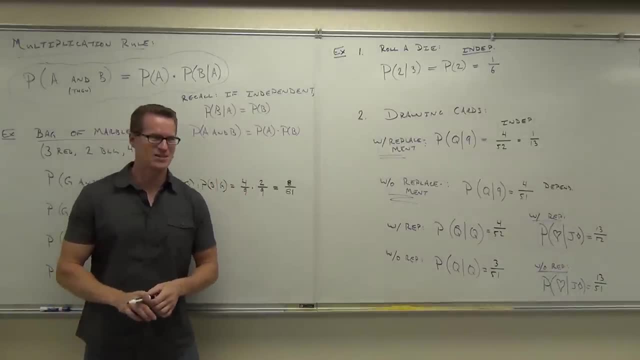 No, it's not eighteen, Okay, Yeah, no, it's saying we multiply it straight across. You simplify as you go as well. Nothing's simplified here. So we have eight over eighty-one. You punch that into a calculator to find a decimal. 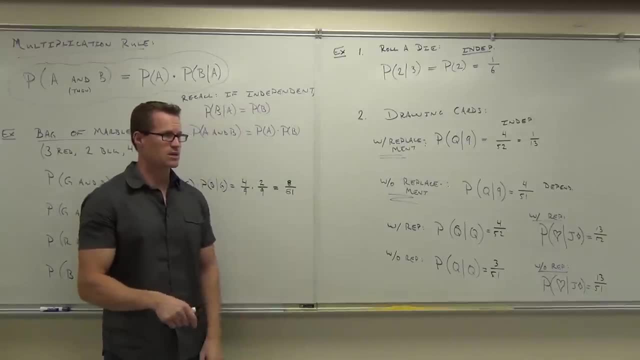 Notice how that's a relatively small probability. So say what's the probability of selecting a green marble, putting it back and then selecting a blue marble. Right, putting it back and then selecting a blue marble? It's pretty low. 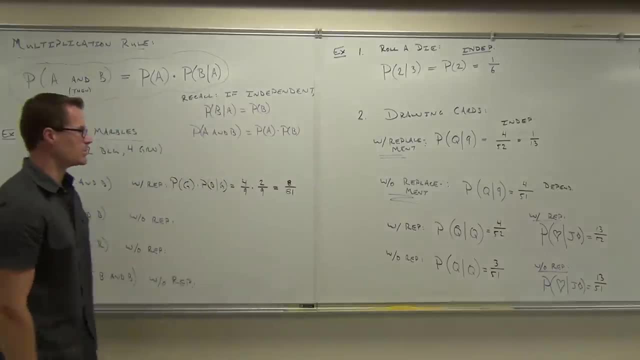 It's not up there. It's not like 50-50 or something like that. It's pretty low probability. Okay, let's do the green and blue without replacement. So this would be the probability. It's going to be identical. 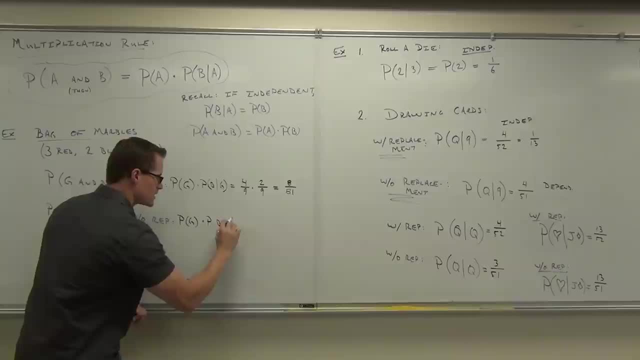 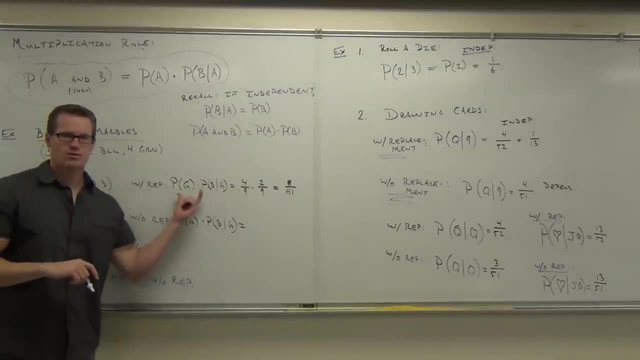 Probability of selecting the green times the probability of selecting the blue. given you just selected the green, What's the probability of selecting the green? Notice how this one's the same right Probability of green. that's just there. That's your first marble. 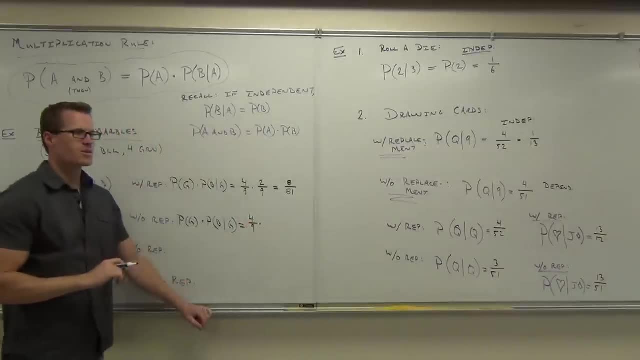 That's not going to change Times. can you tell me the probability of selecting a blue marble, given you just selected the green marble and you kept it out? Good, There's still two blues, but there's only eight marbles. 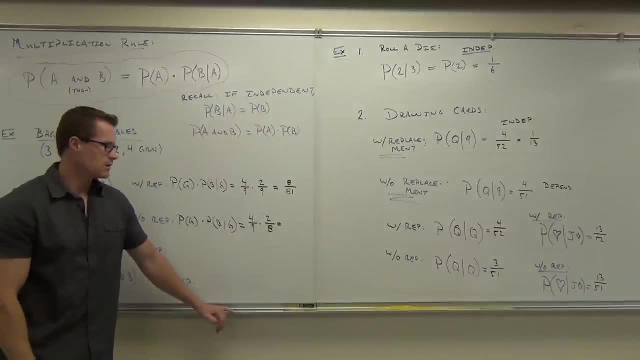 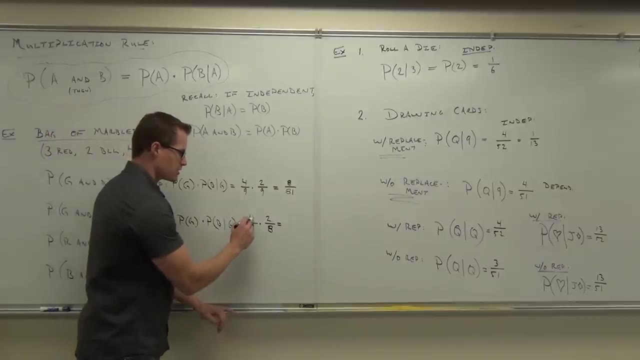 How much is that going to be? You could put 8 over 72.. However, this does simplify, so you need to know how to simplify fractions. 4 goes into 4 one time and then 8 two times True. 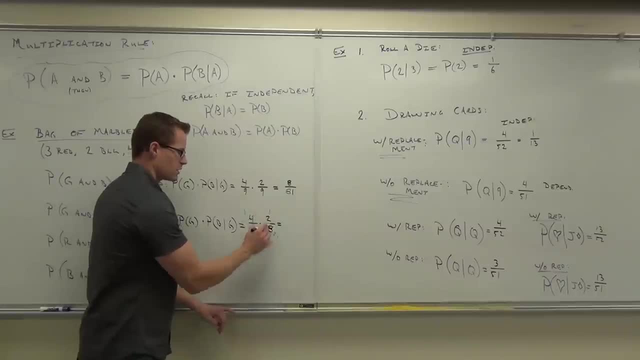 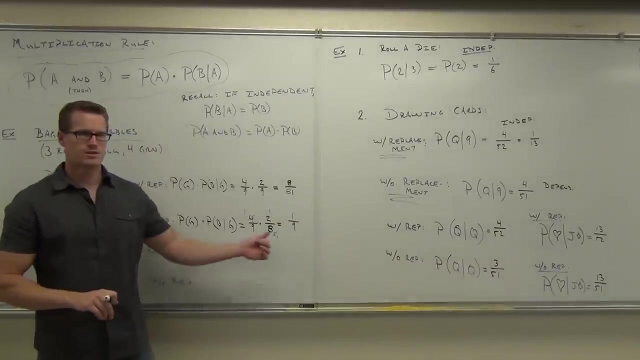 Yes, 2 goes into 2 one time and then into 2 one time. You get one-ninth, You get one-ninth. It's a slightly better probability that this is going to happen than this is going to happen and I hope you understand why. 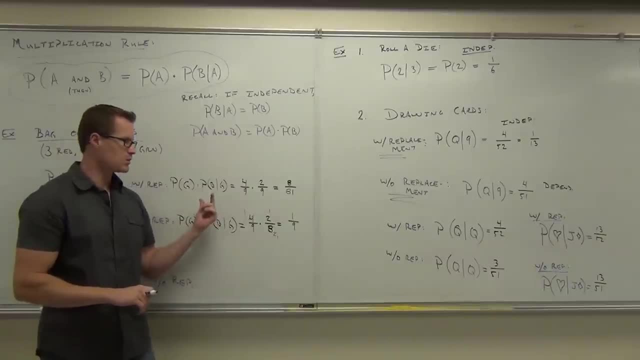 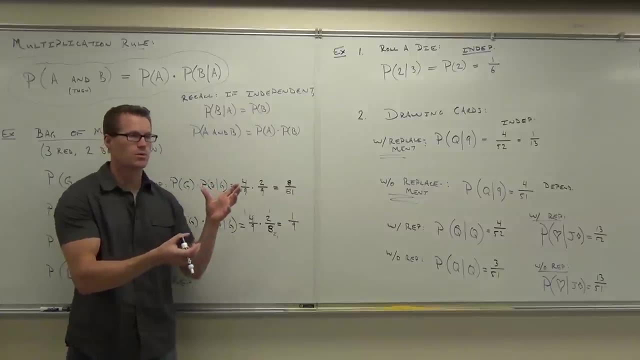 If you pull out a green marble and then you look for a blue marble, if you put it back, you add one more. If you add one more to the marble numbers, it's not green, right, Or, I'm sorry, it's not blue. 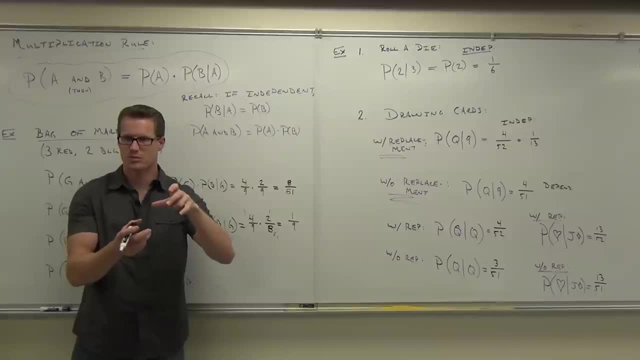 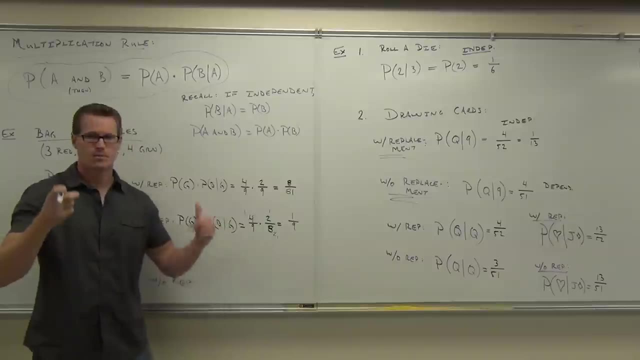 So you have less probability of selecting that blue marble. but if you keep the green one out, there's only eight marbles not to choose from- You have a better probability for that second marble to be blue. That's the idea here, okay. 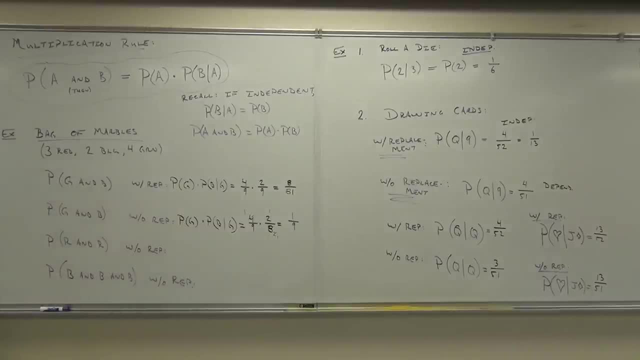 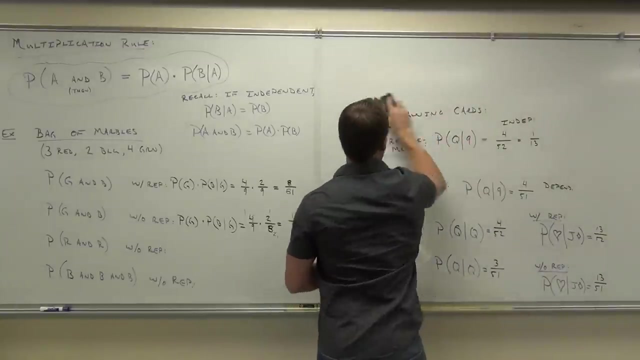 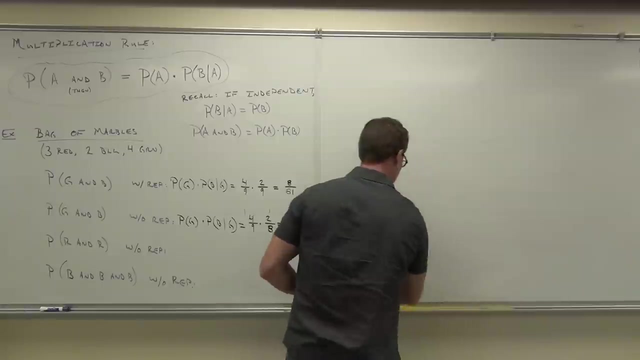 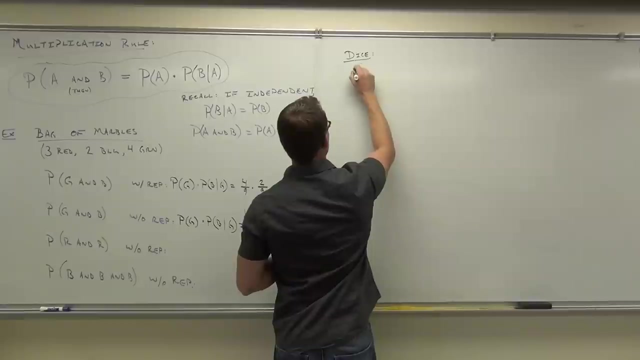 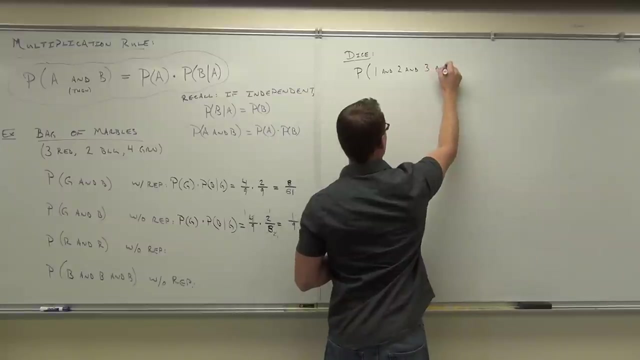 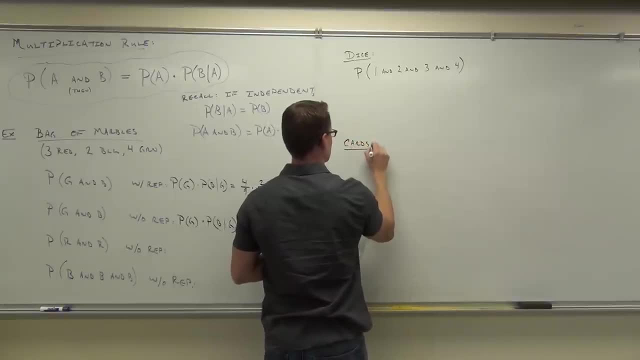 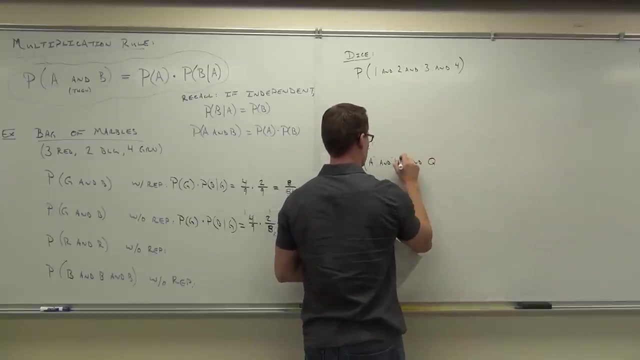 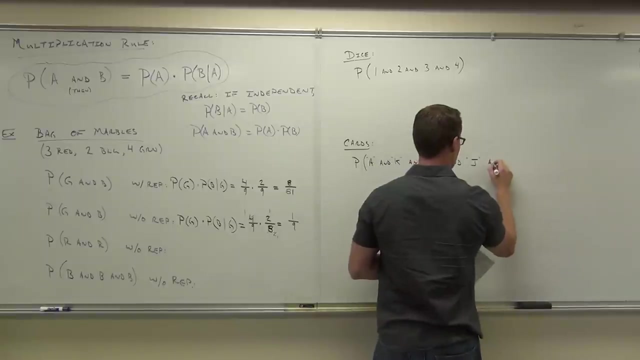 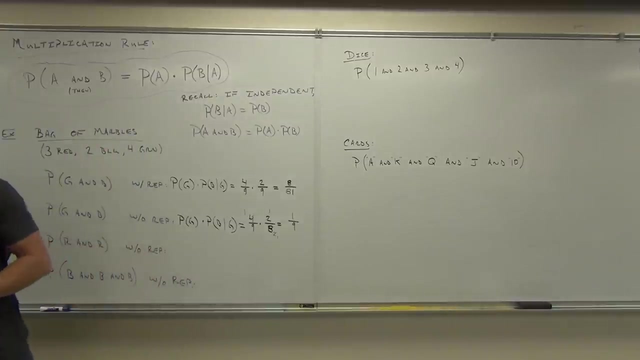 Thank you. We only have a few more minutes so we're going to start on this problem over here. The probability of selecting a red and a red without replacement, meaning you can select a red marble, you're not going to put it back and you try to select another red marble. 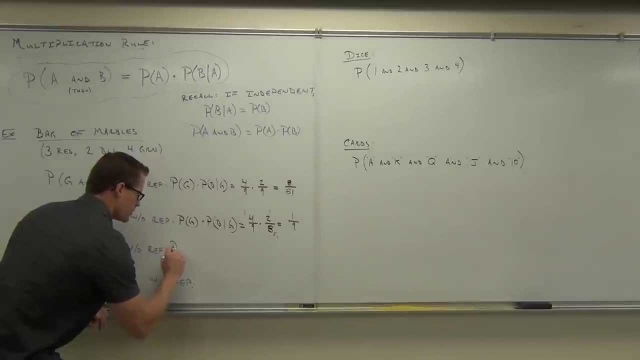 The first red marble. you have three of them. so probability of red times the probability of red, given red without replacement, The probability of red this one is three out of nine times the probability of getting a red, given that you've got the red out already and you've kept it out. 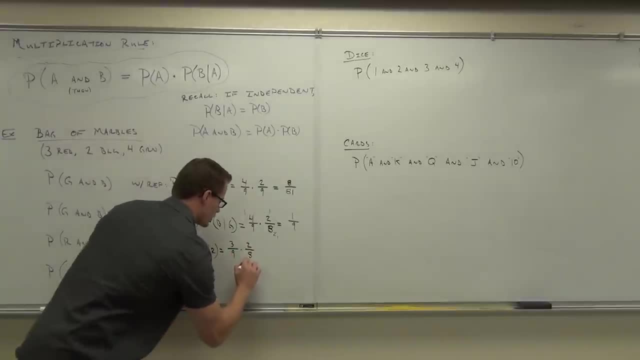 How many reds are left? How many marbles are left? Perfect, So you're going to get six. You can reduce this as well. Sorry, Two goes into two. one time Two goes into eight. four times Three, nine, one, twelve. 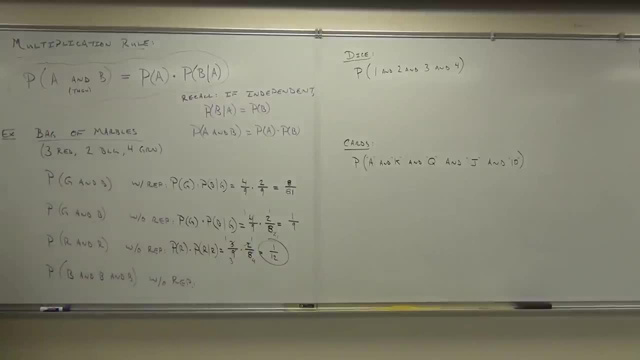 You have a one twelve, So you're going to have only one probability of selecting a red marble and then another red marble. Are you okay with that one? How many people got that one? Good, You can give me a decimal as well. 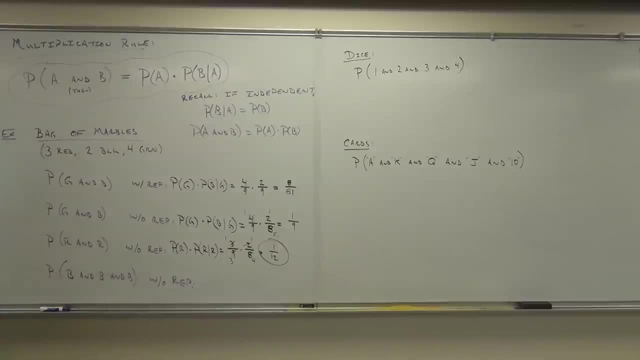 That's fine. How about blue and blue and blue? Well, this would be blue, given you get a blue, given you get a blue. So what's the first one? blue? What's this probability of selecting your first blue Times? 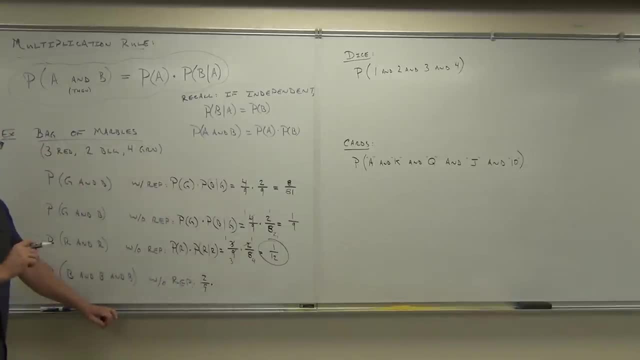 Times. What's the probability you're going to keep it out- out, by the way- and select another blue One. Okay, What's the probability you're going to get another blue Zero? Why, zero, Zero takes no one. 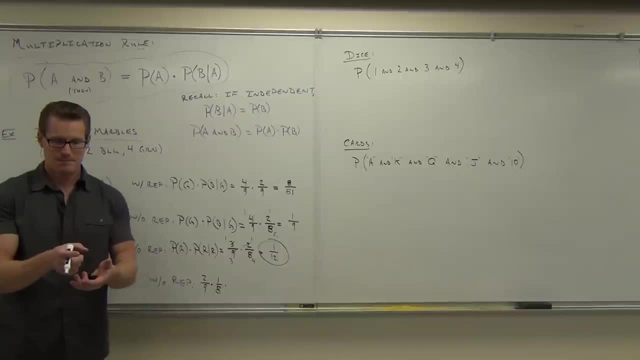 If I say this: hey, I've got a bag full of two blue marbles and the rest of them are different colors. I'll give you a million dollars if you select out three blue marbles in a row without putting them back. Or you give me ten dollars if you can't do it. 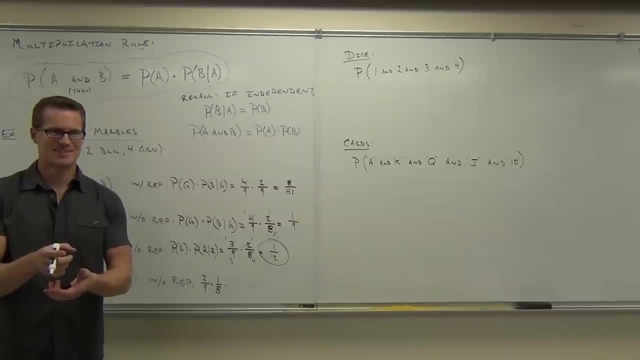 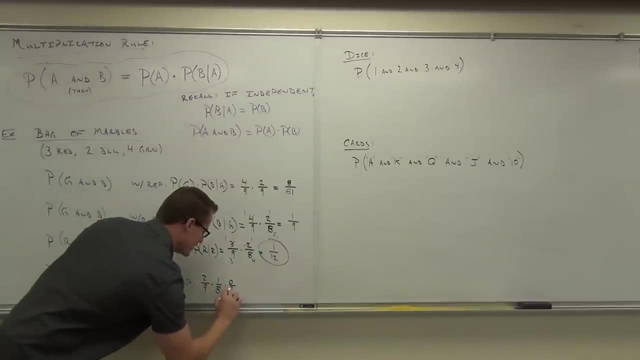 Is that a good deal? I'll make you that bet all day long. Is it going to happen? No, There's only two blue marbles. You can't draw out three if there's only two of them, So you'd have zero over. 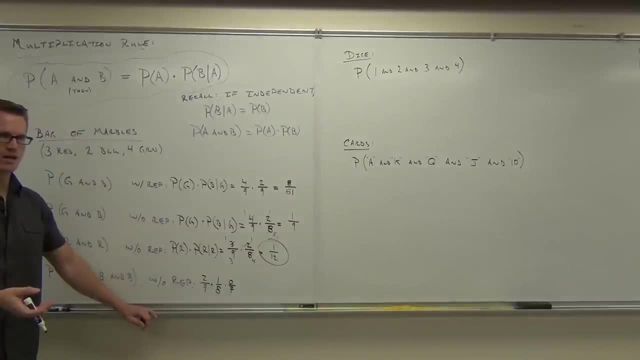 seven for sure. right, There's zero blue marbles- over seven marbles remaining. But look what happens here. What's two times one times zero? Zero. Nine times eight times seven is some big number, but it doesn't matter, You have zero over some. 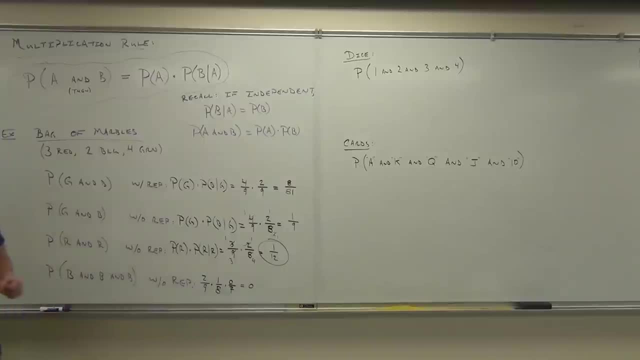 number, This is going to be zero. That's an impossible probability. Now, as far as the last one goes, the last minute and twenty seconds that we have up here, If we're going to roll a die, what this is going to be. 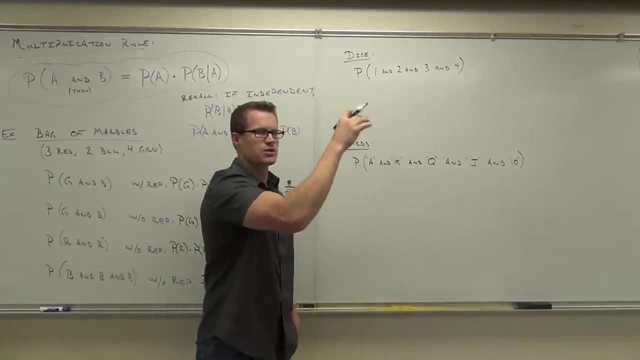 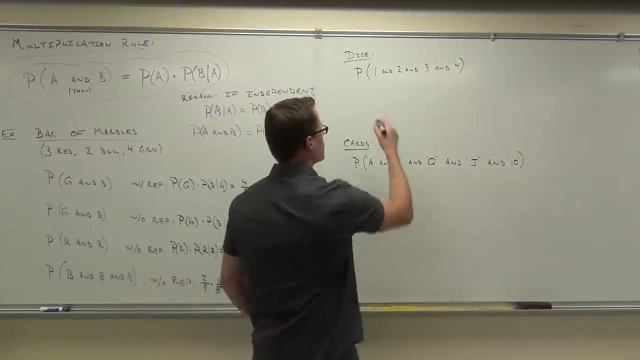 is the probability of one times the probability of two, times the probability of three times the probability of rolling a four, Because all these things are independent, The dice doesn't affect each other. So this probability would be the probability of one times the probability of two. 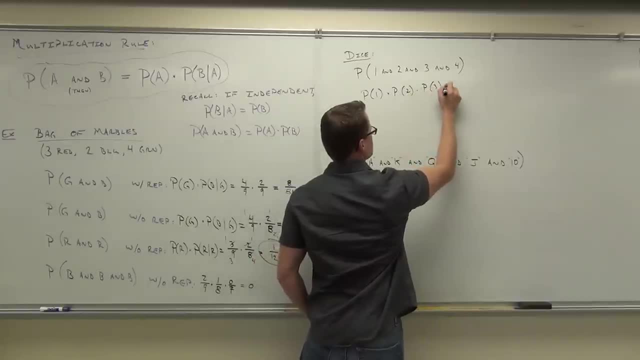 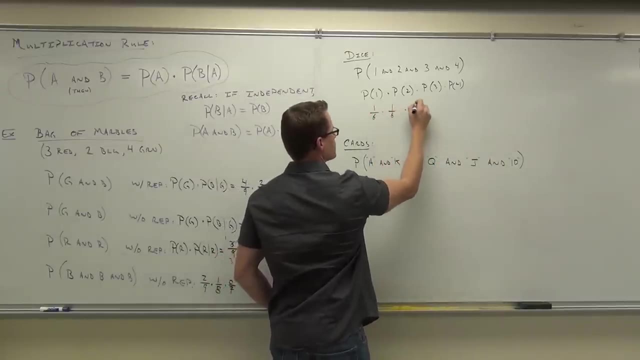 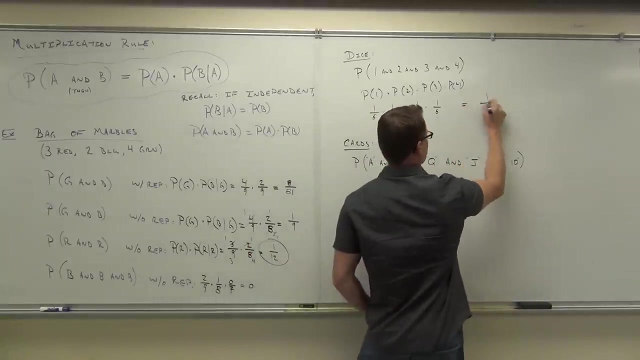 times the probability of three, times the probability of four. They're independent events. Those probabilities aren't affecting each other. So you would have one-sixth, one-sixth, one-sixth, Or someone take six to the fourth power numbers, Anybody. 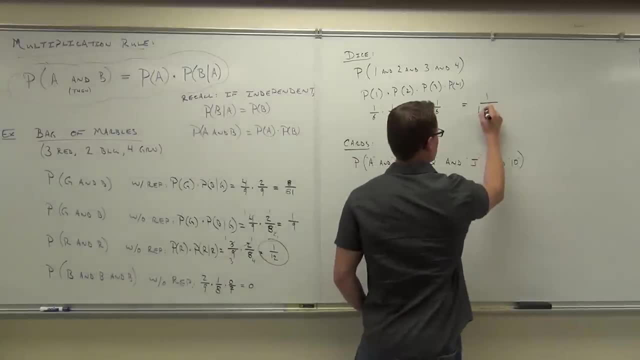 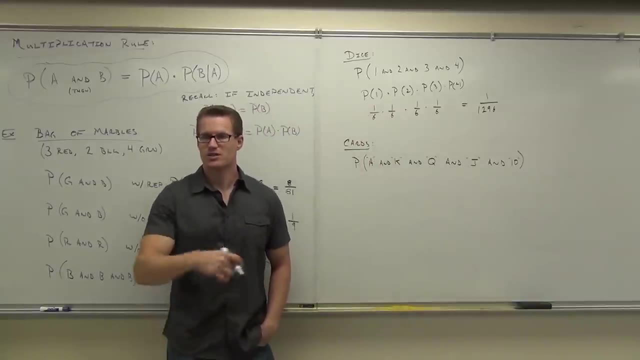 One thousand two hundred and ninety-six. Is that a good probability? So let's say I'll make you a bet on this one And say you roll the die four times in a row. You have to get a one, a two, a three and then a four. 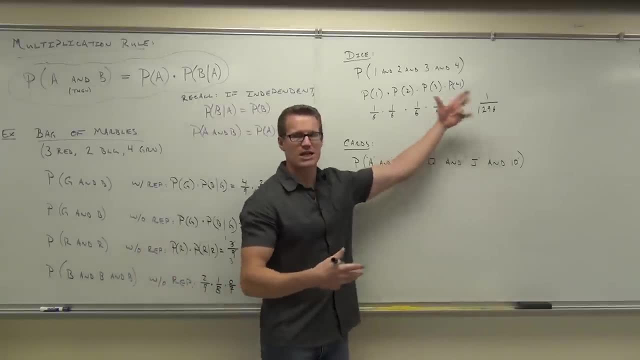 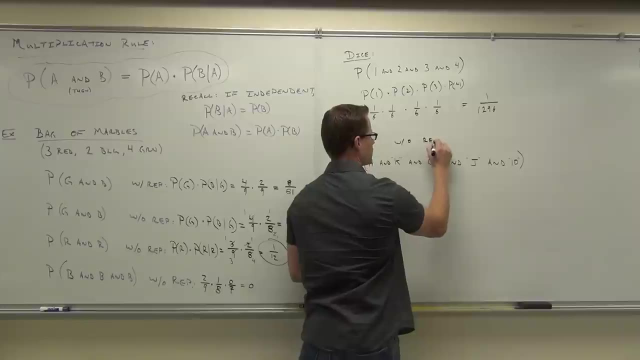 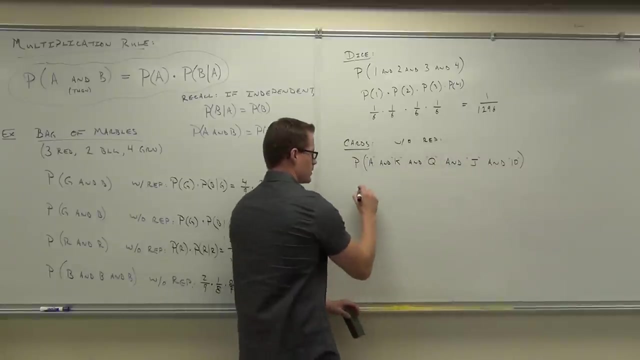 Is that going to happen? Probably not. You guys understand the independence as far as this goes. How about this one? This would be without replacement. Without replacement: Probability of the ace. How many aces would you have to start with Out of? 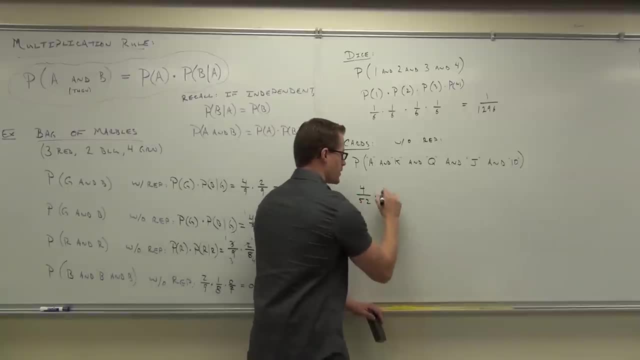 Times. How many kings would you have Out of? Explain why. fifty-one Times how many queens Out of? Four jacks out of forty-nine, Four tens out of forty-eight? If you multiply those, you do your simplification. I don't know what the numbers would be.